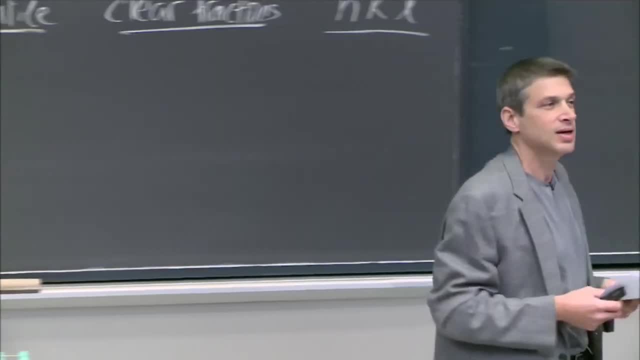 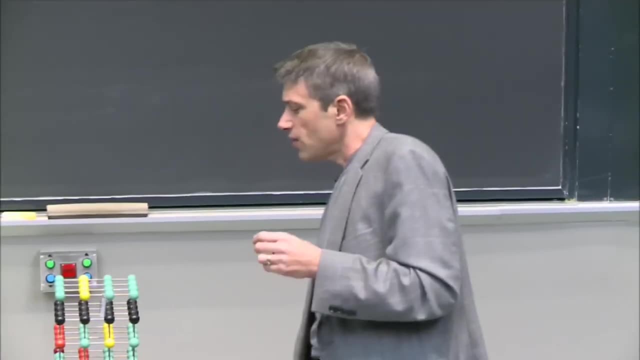 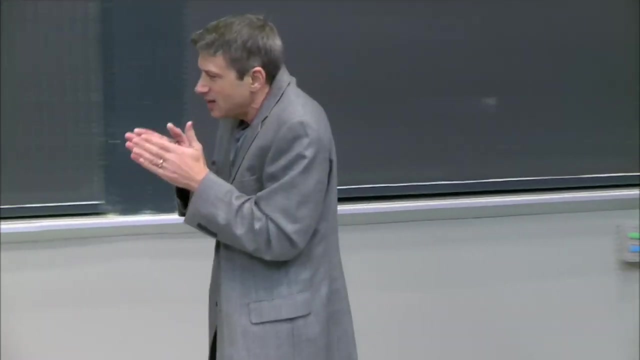 I want to go back and make sure we kind of get this right. We talked about the Bragg condition and we talked about how you know the unique thing about about X-rays is that their wavelengths are right in that, in that you know, in that sort of precious distance regime of the spacing, 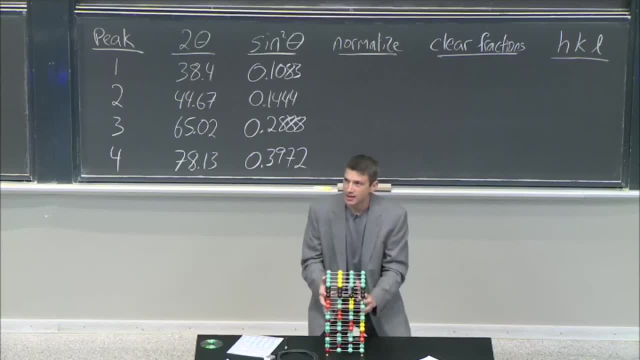 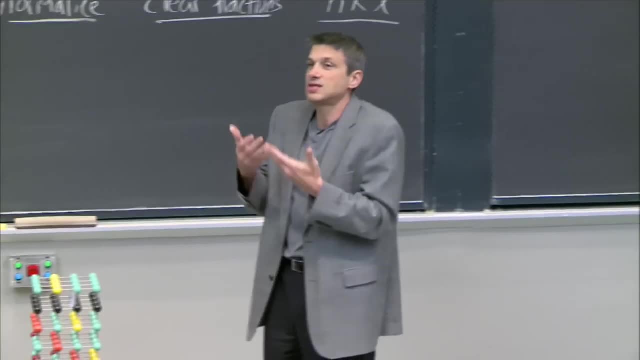 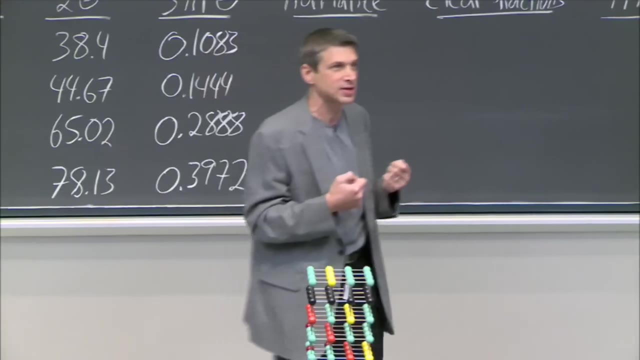 of atoms in a crystal. And so if I, if I shine them on the crystal, then they're going to be, they can diffract and they can have constructive and destructive interference, but only if they sort of line up right. And that's what the Bragg diffraction tells us. It tells us the condition. 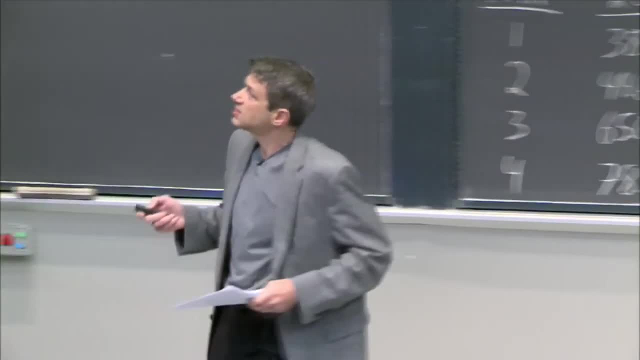 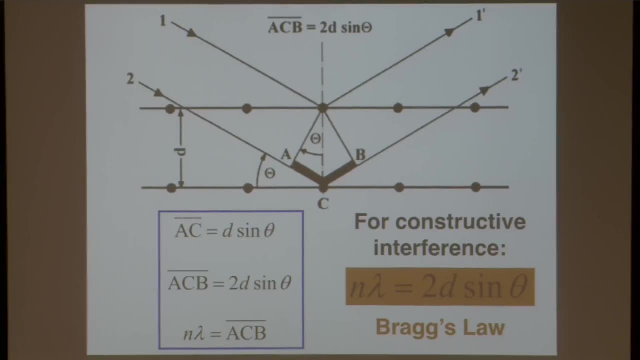 the Bragg condition for when they line up And, in particular, this is a pretty nice image. okay, So you can see here's one ray coming in, one X-ray coming in, and it's a wave, It's a wave. 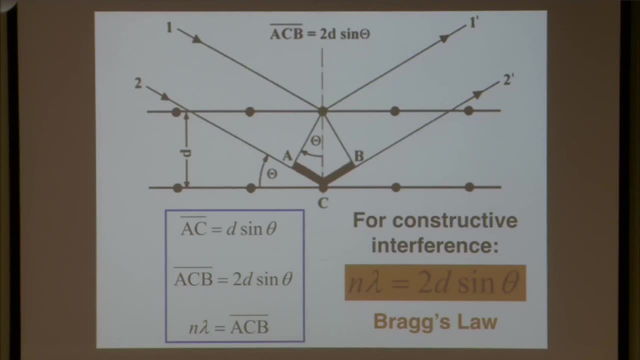 So it's going to be a wave that goes like that, And then it bounces off this surface. Now a second one doesn't bounce off that top surface, It bounces off of the one beneath it. Okay, And they're separated by a distance D, So this could be any set of planes, right? So if you take this, 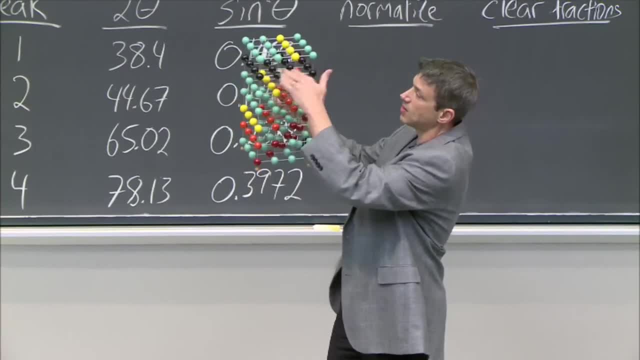 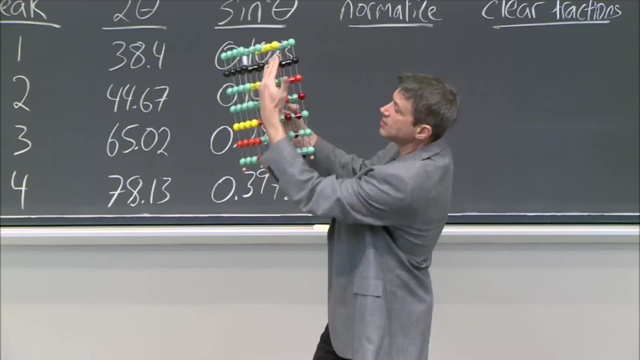 so here are my planes now. So so these black atoms are one plane, right, But these yellow ones are another one. That's another plane that you could see. Remember, one of the assumptions of the Bragg condition is that these planes are like mirrors, So we lose a sense of where. 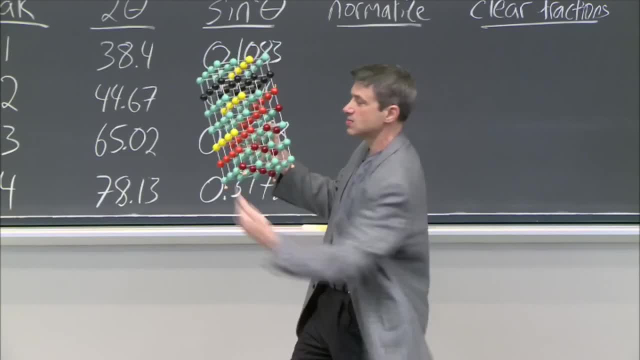 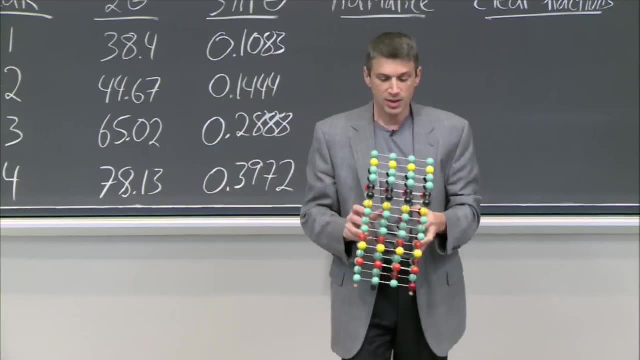 where the atoms are exactly, And we just write a mirror there. We say it's reflecting off the mirror. So where's the next one? right, You can take the orange ones- That's another plane. the red ones and so forth, right? So that's what you're. you're now you're. you have a wave on. 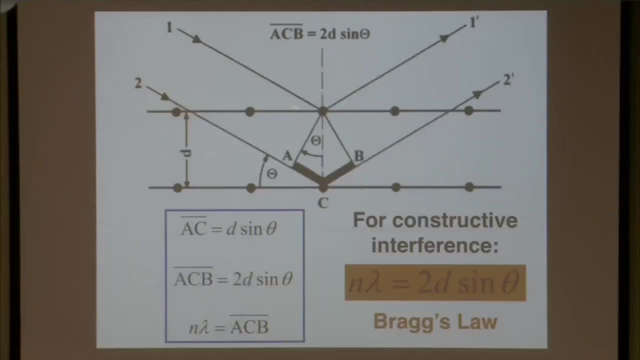 top. Okay, You've got a wave on top and then you've got a wave coming down and bouncing off the one beneath it, And for those to constructively interfere so that you pick up a signal in the detector right, There's only one way for that to happen, And that's if this: 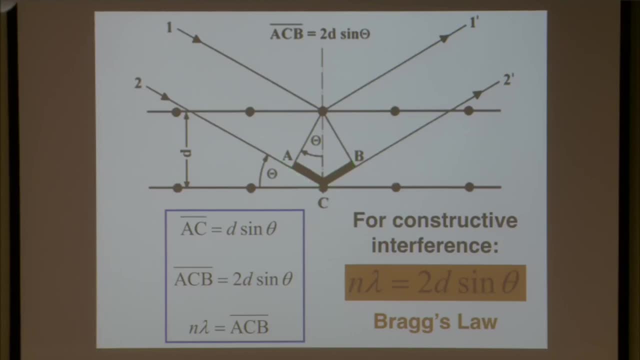 distance plus that distance is equal to a multiple of the wavelength right, And that is the Bragg condition. You can see why it comes off. Why doesn't it? you know it has to come all the way down to here, which makes that theta equal to that theta. You see that because 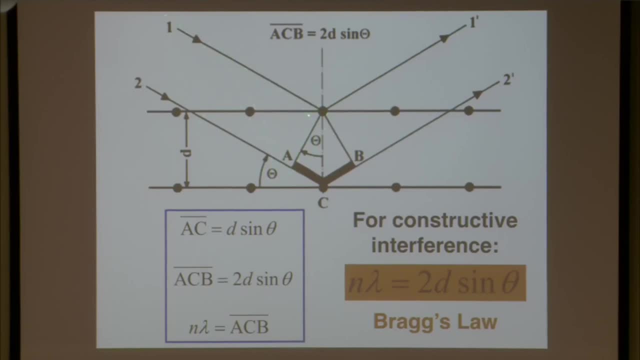 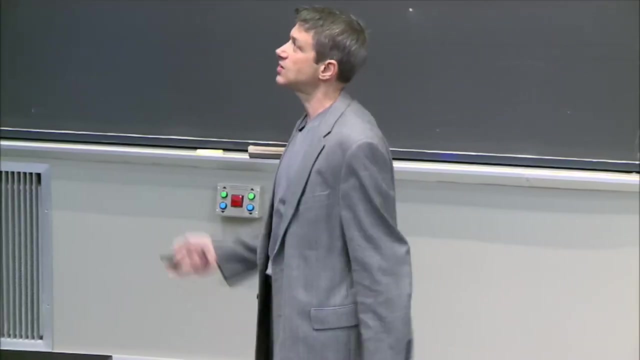 they've gone up to this point, up to that line, they've gone the same distance. So they're waving together right. And it's that point where now, this is the extra that the one that bounces off of this plane, that's the extra distance it goes. That's the Bragg condition. Okay, That's the Bragg. 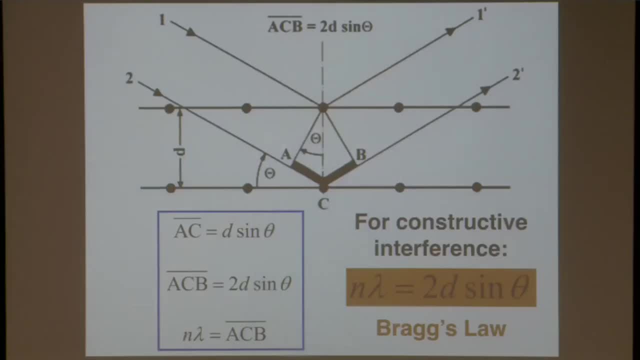 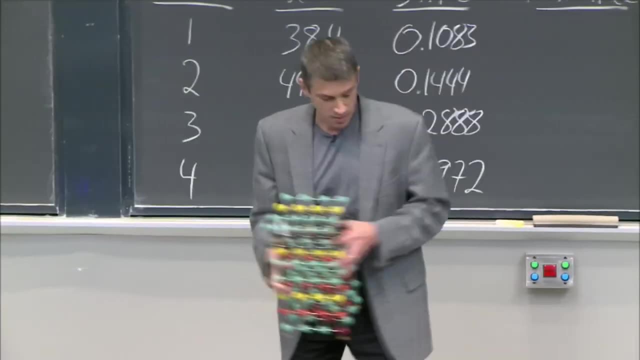 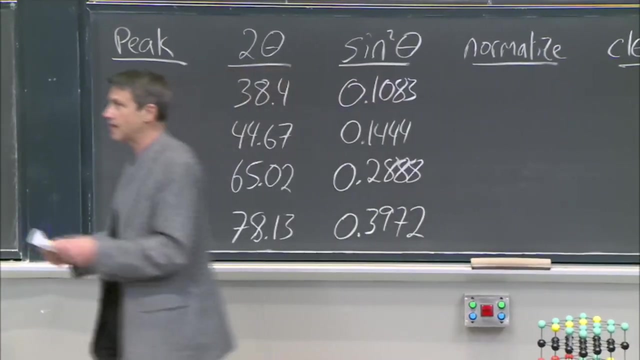 condition, And remember in this class: okay, so it could be any, uh, multiple, but but here we're just going to assume n equals one because it's the easiest case. Okay, good, That's the Bragg condition Now. um then we did something beyond just just that, because 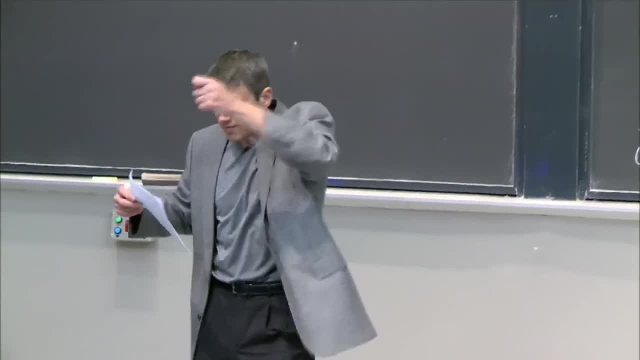 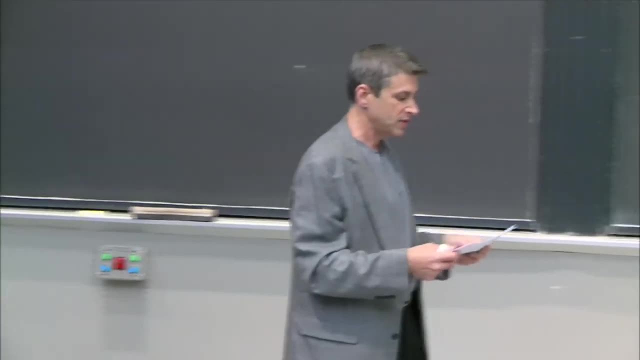 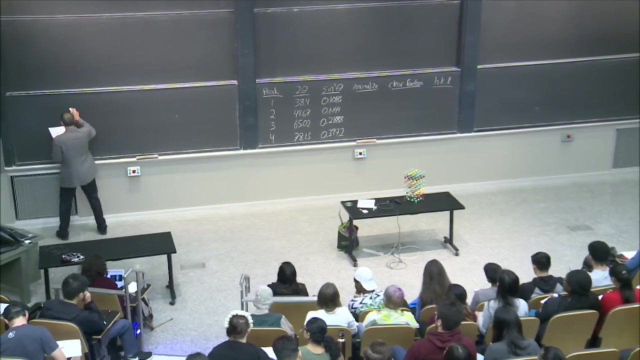 that tells us, you know what the wavelength has to be to get a spot, to get something the detector can see, because it constructively interferes. Everything else is destructive. no signal, right? Uh, but we did one more thing right. We also said that D for some. 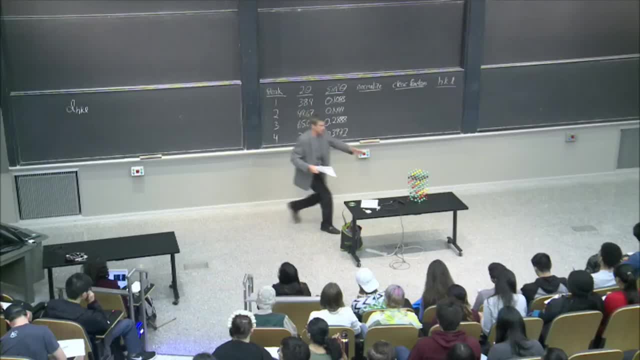 set of planes. remember this: this HKL is just telling me which one of these I'm talking about. That's what HKL is. I'm going to pick one of these planes and the distance between them as DHKL. Okay, good, And and what we know from before, from our 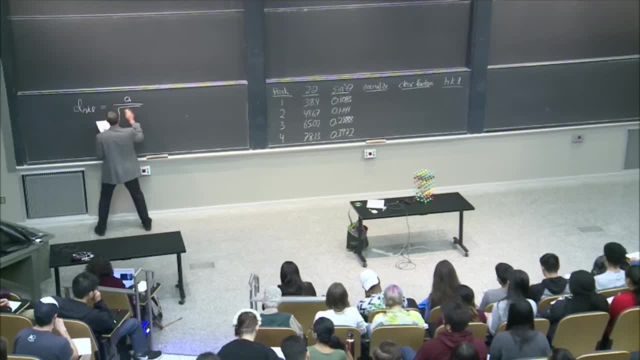 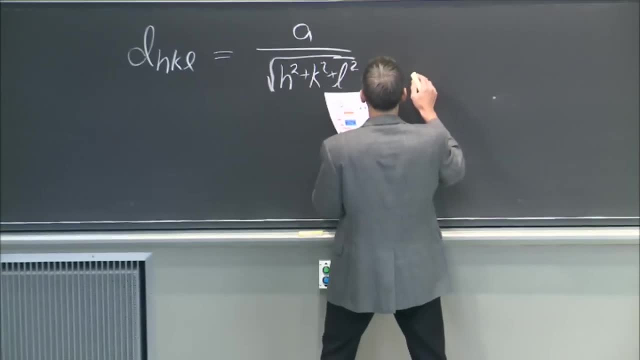 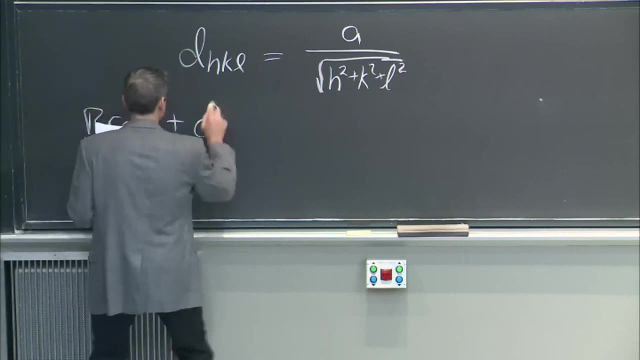 Miller times. we know that that is equal to the square root of a squared plus K squared plus L squared. for the cubic lattices we're talking about right. So you see, it's kind of Bragg plus Miller, Bragg plus distance, Miller, right, Miller, cubic. That's what we're really. 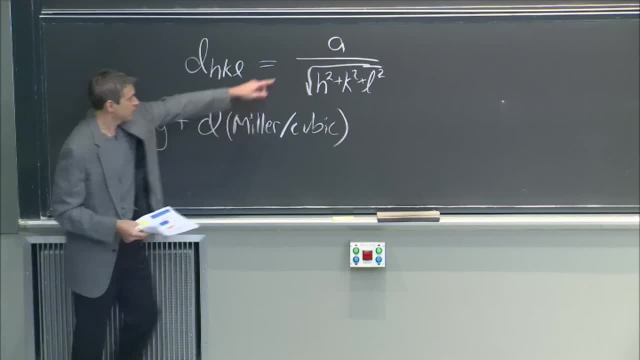 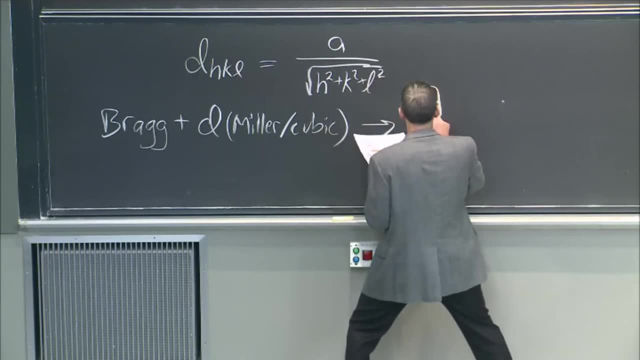 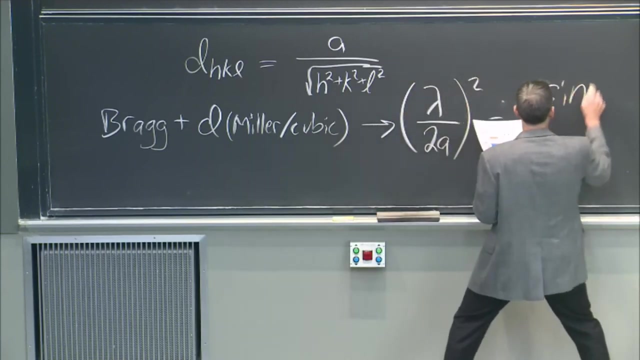 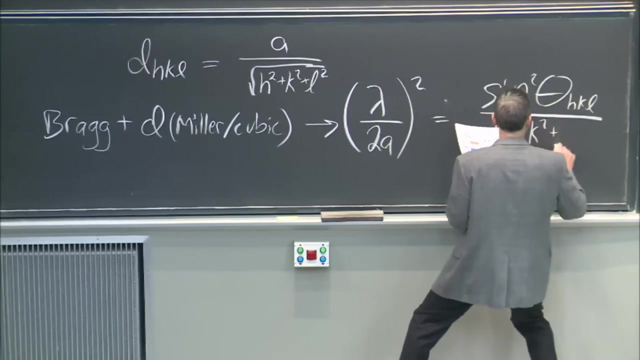 combining here The distance given by this formula when we talk about Miller planes that combined Gave us this: Lambda over two, a squared equals sine squared theta, HKL over H squared plus K squared plus elsewhere. And all I've done is substitute and square. Okay, And we did. 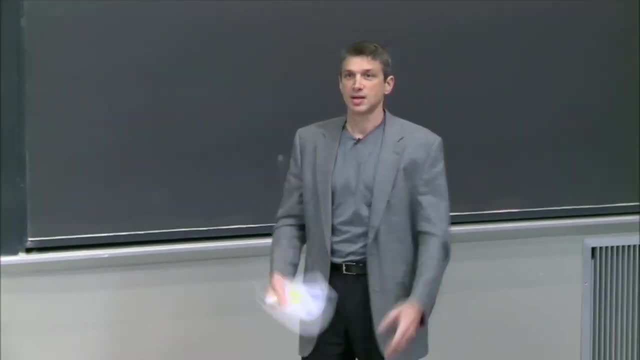 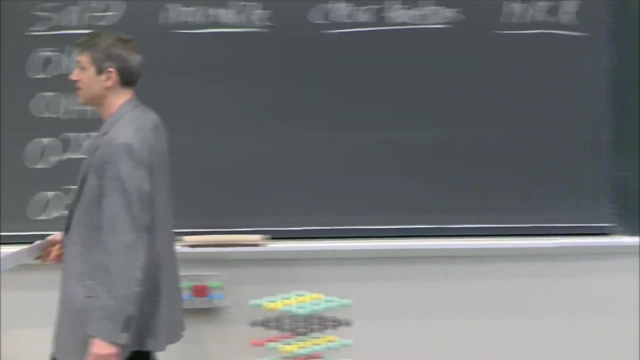 one more thing on Wednesday, and we talked about constants and we said: well, something's equal to a constant, then it's a constant, Right, That's some good math, That's some good math. And so we said: well, that's the. 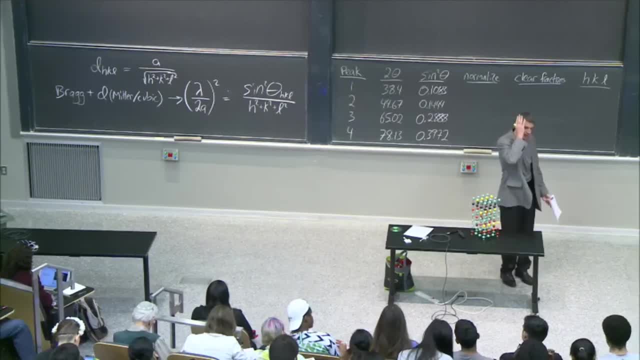 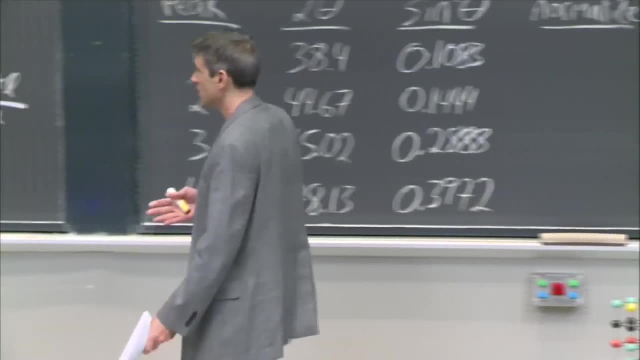 whole beauty of these characteristic x-rays, because if you take like a K alpha line from copper, it's always 1.4, 1.5, four. sorry, Angstroms, it's always Lambda equals 1.5, four. 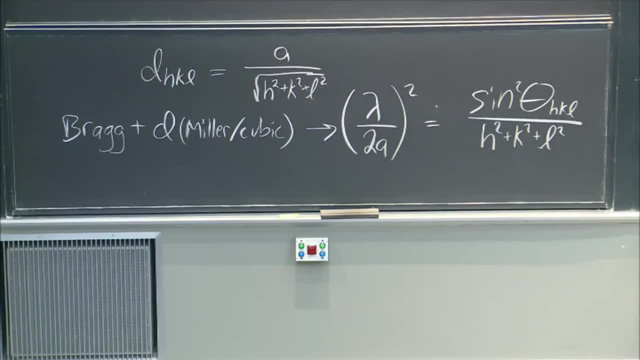 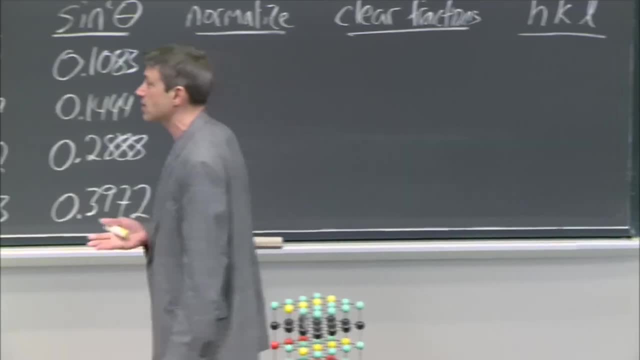 That's what's so nice about it. It doesn't depend on anything else, Just the metal you put in there as the target And it's called a target because you're you're targeting it with electrons. So the copper target, K alpha. 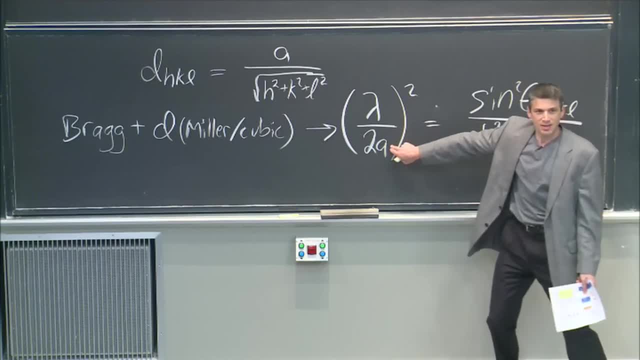 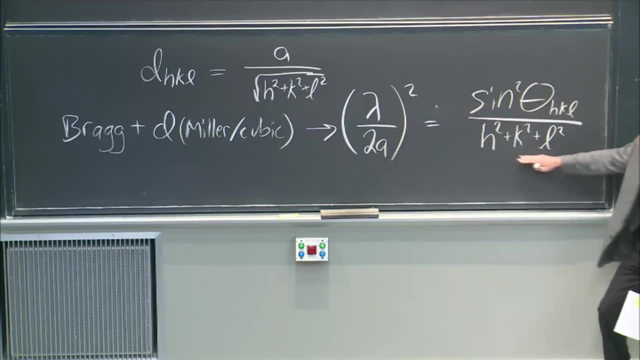 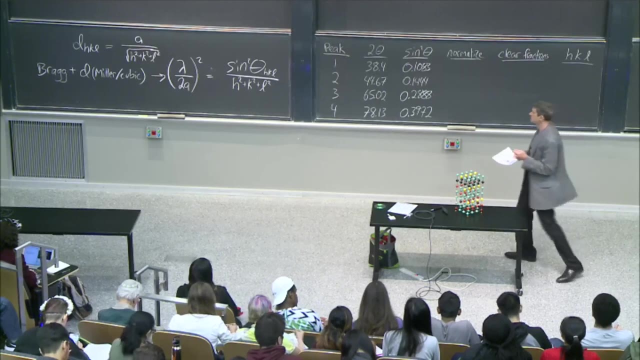 Lambda, constant, lattice, constant- That's built into the name constant. constant equals the angle and the plane it's reflecting off of, And so our, our, our job, then, in crystallography and doing x-ray diffraction, our job is to figure out how to keep this thing a constant. 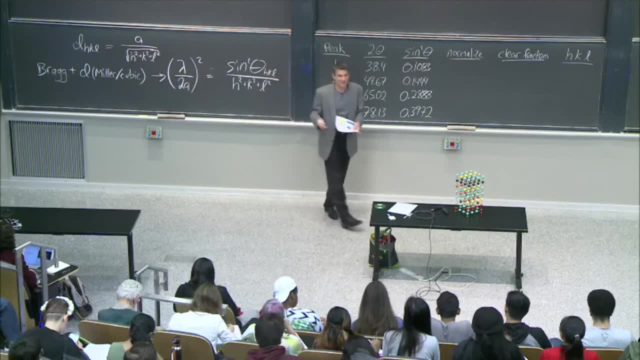 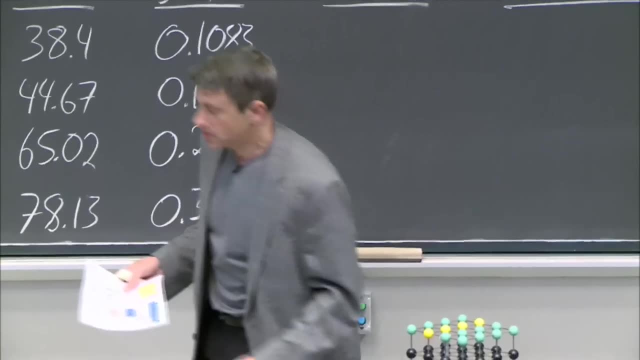 the same constant, right? That's what constant means. Okay, And that's our job, And that's that's where we left off. We said, okay, well, let's take this to the next level, Let's do an actual experiment. 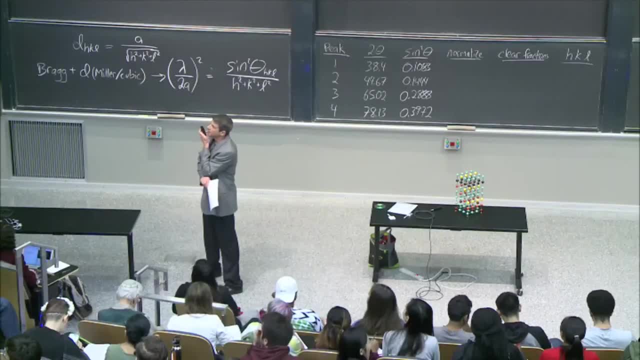 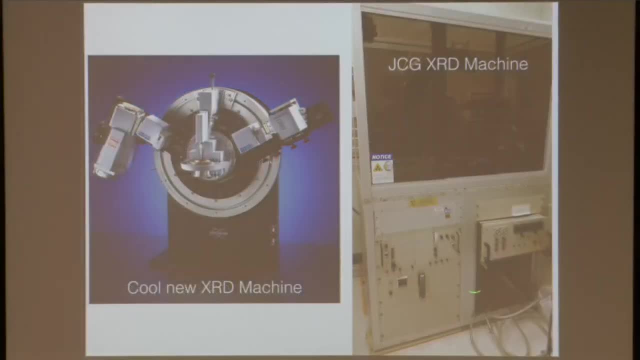 Now, how do you do experiments? Well, you have equipment, and this is what a really cool XRD machine looks like. This is what happens when you don't have any money, And so this is what's in my lab. but you see, it's true, You can come see it, but you see the the point is: 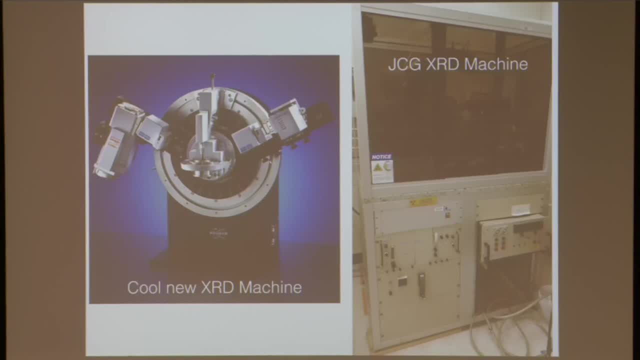 they knew the same thing. We don't need fancy equipment at MIT. No, we can. it's the ideas that matter that you're putting into this thing. But that's kind of cool. I like the way that looks. Same thing right. Source sample detector. It's hard to see. 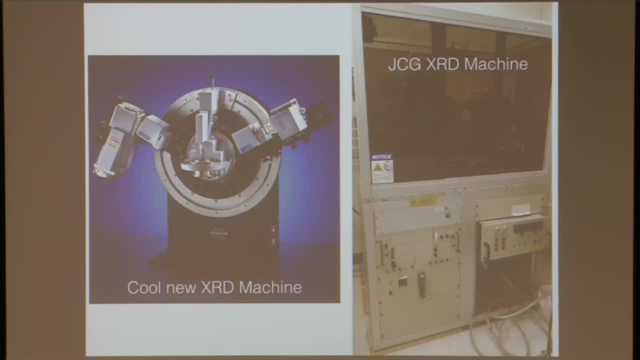 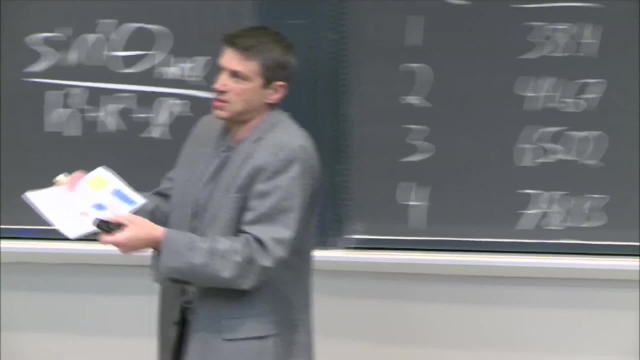 but source sample detector from the sixties, ish, Okay, All right, But so now it's easier. Of course you can understand. I mean, some of these things have different ways of doing, but you can understand. like changing the angle, it's going to be easier to move that sample. 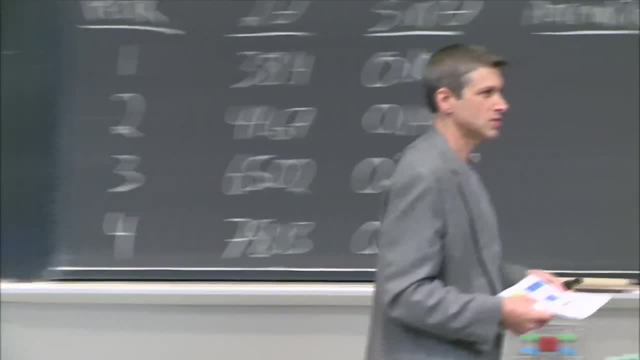 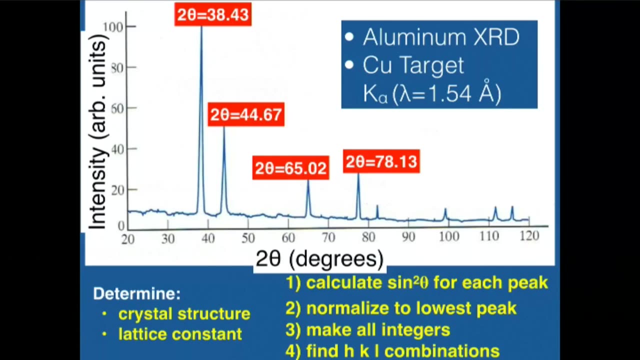 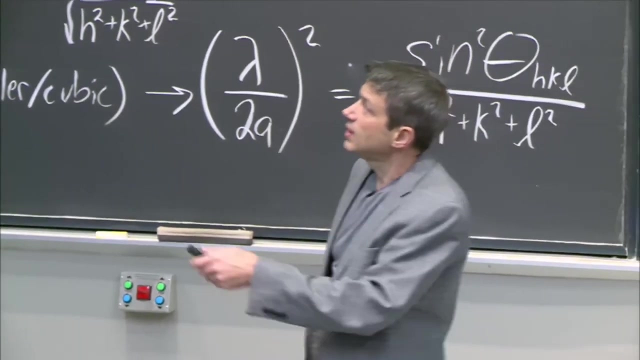 right, And then maybe the detector moves, but you might keep the source x-rays fixed. And what happens while you do this? And you generate a spectrum, right? So so you're changing the angle, You're keeping this fixed and you're saying: what do I got? Okay, well. 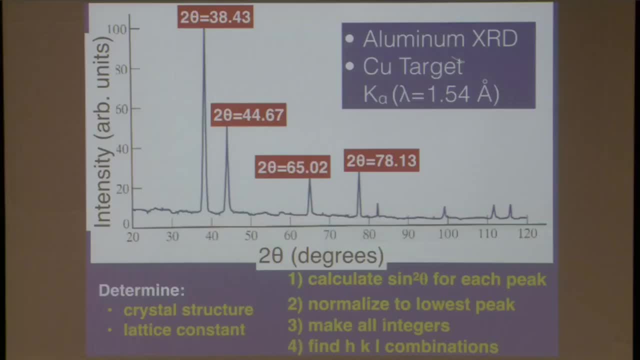 here. in this case, I'm telling you what I got. I got aluminum, I put aluminum in there and I shot x-rays. and I have to. you cannot, if anybody gives you an xrd pattern, they got to tell you what kind of x-rays they use. right, That's really important, Or at some. 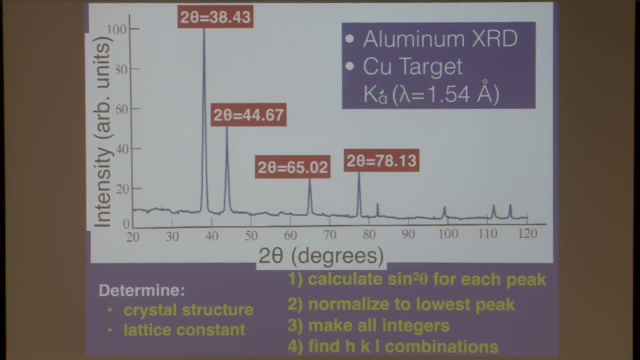 point. you got to know this. This is pretty important. The lambda is from a copper target and the k alpha lines is 1.54 angstroms And this is the spectrum And I'm being asked to get the crystal structure. 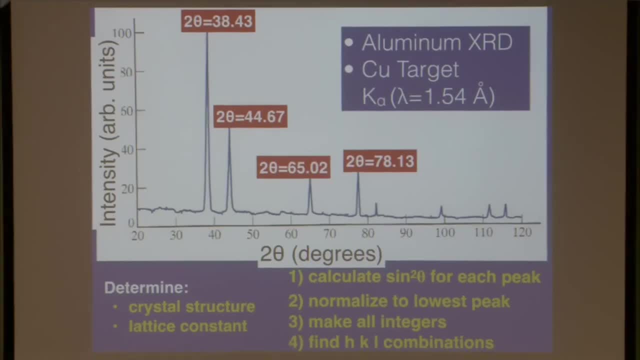 of aluminum and the lattice constant. And I can get that because, look, I can simply read off peaks and those are the peaks And I've kind of highlighted them there. to theta, right To theta, Remember we put more for historical reasons. You take two theta measurements. 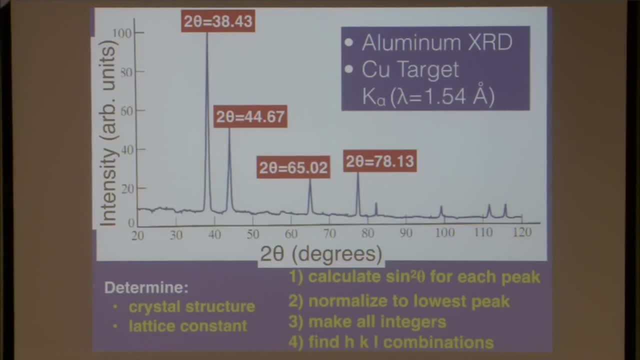 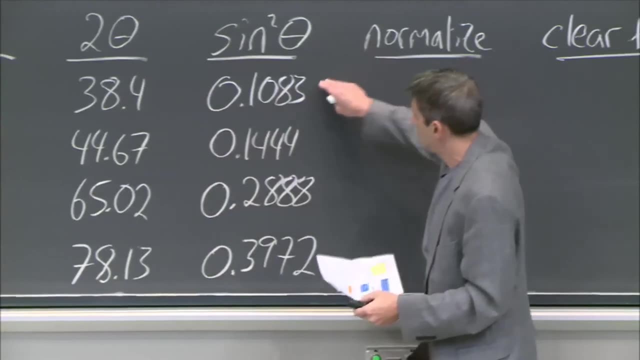 even though in the Bragg condition it's just theta. Okay, we can divide by two, right. And so here are those first four peaks, And I've just listed them here: Peak one, two, three, four. Here's peak one, Sine squared of half of that Gesundheit. Okay, there it. 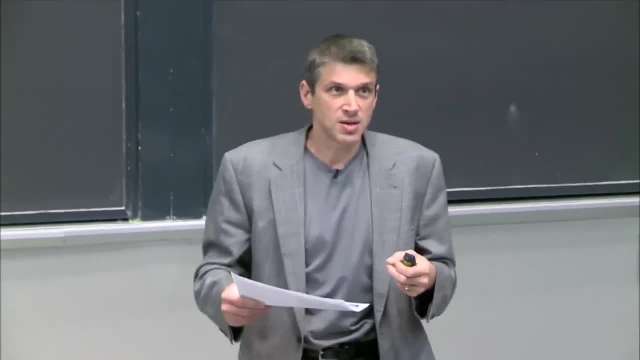 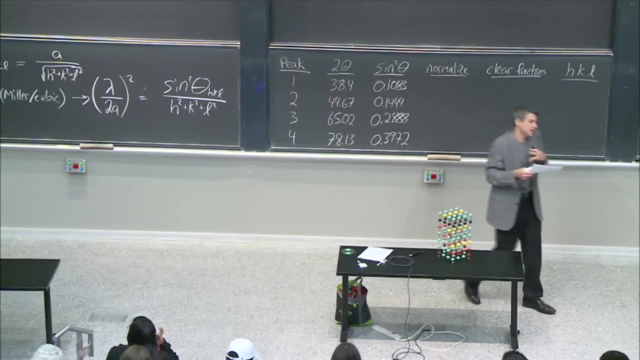 is, And then we have our recipe, And I gave you this recipe as a way to keep this constant. It's an easier way to do it if you scale and clear fractions. It's just easier, right. So that's why I've given you that recipe. 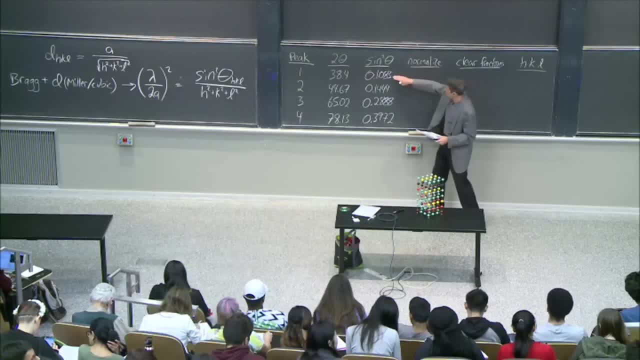 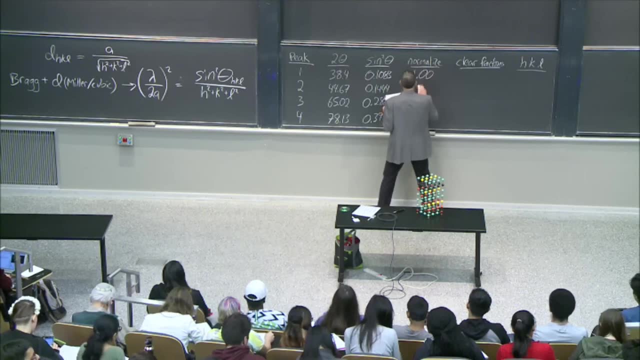 So let's do that. So first we'll normalize. What does that mean? Well, you have the smallest value of sine squared theta. I'm just going to divide everything by that. Okay, so that's where we left off One, because that's what I'm normalizing by, And then this one would 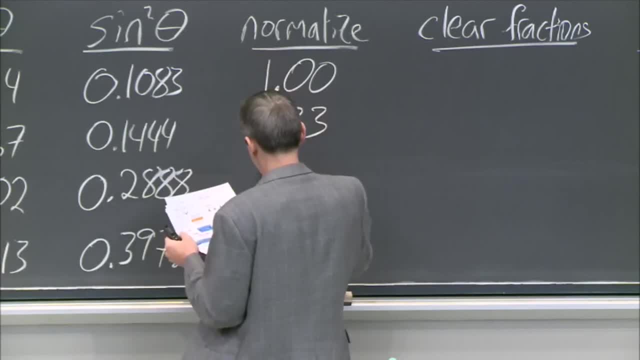 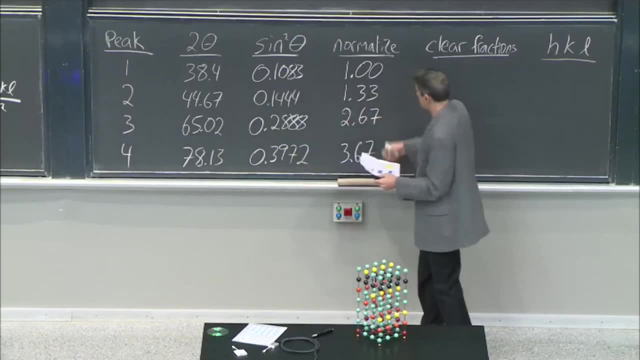 be 1.33.. And this one would be 2.67. And this one would be 3.67. And so that's good, but I don't want fractions. It's going to be easier for me to think about this as integers, And. 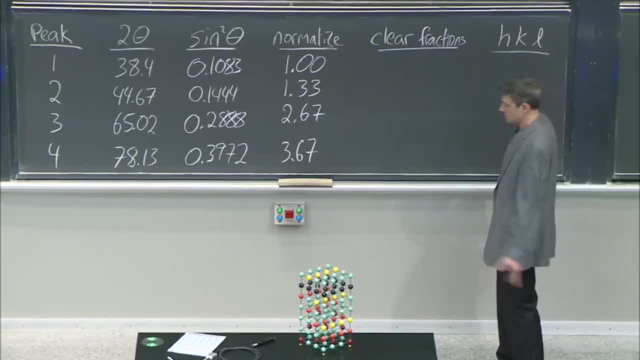 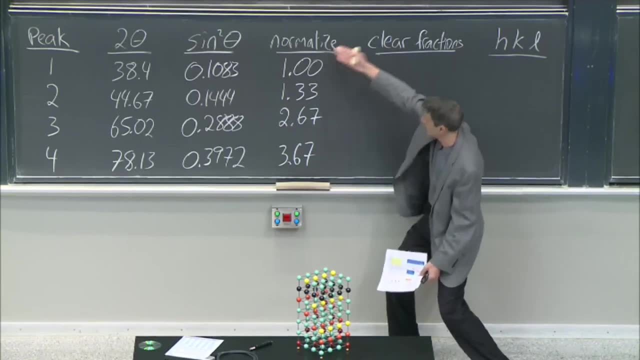 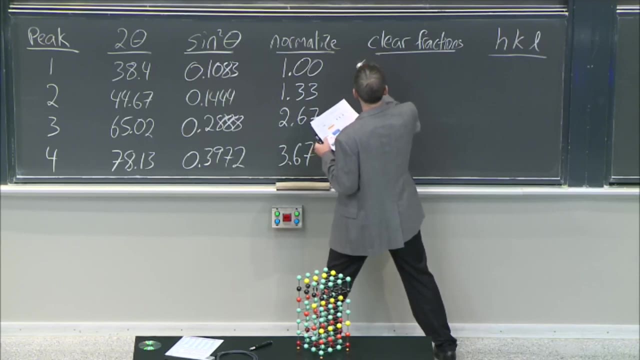 so we clear fractions. What does clear fractions mean? That Clear the fractions, Get rid of them, Make it integers. How do you do that? Find what. you multiply this by so that they're all integers. Okay, I got an idea. How about 3 times 3?? In this case, times 3 equals 3.. Okay, good, And in. 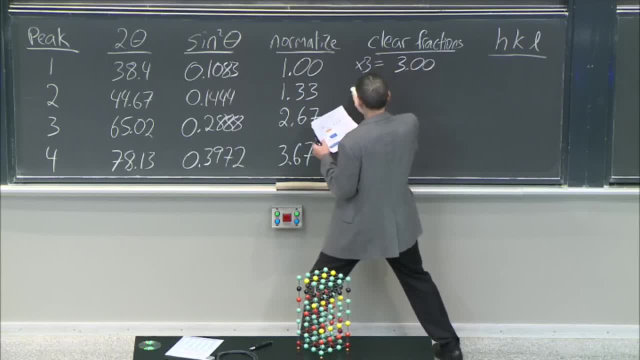 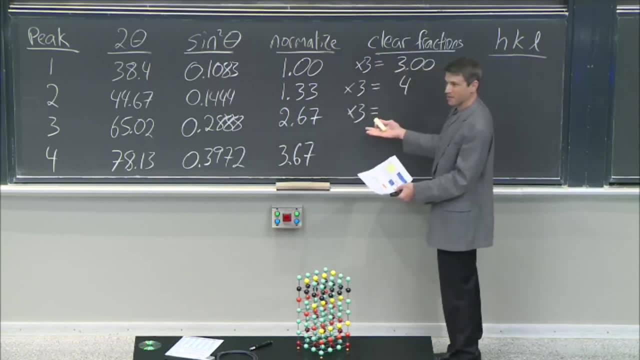 this case? well, I don't mean to. Okay, anyway, times 3 equals 4 times 3.. Don't do that, Chris. Okay, good, multiply by a different number, right, I'm clearing the fractions for the whole. 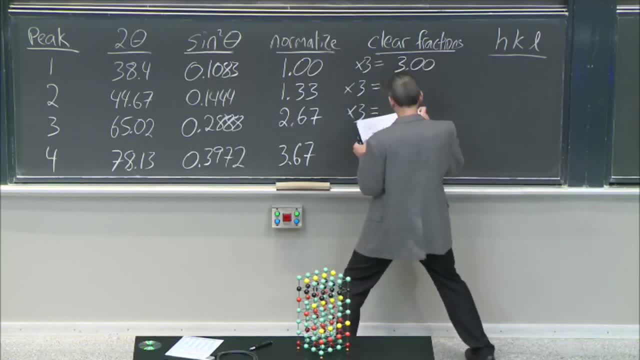 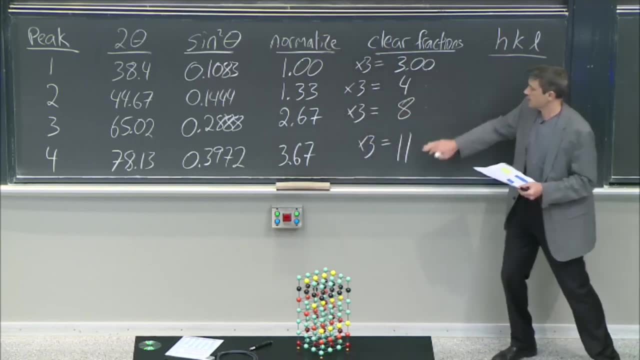 table. I'm multiplying by the same number. Okay, good, 8 and this is times 3 equals 11.. So I've got 3, 4, 8,, 11, and that's what I need to work with. That's what I. 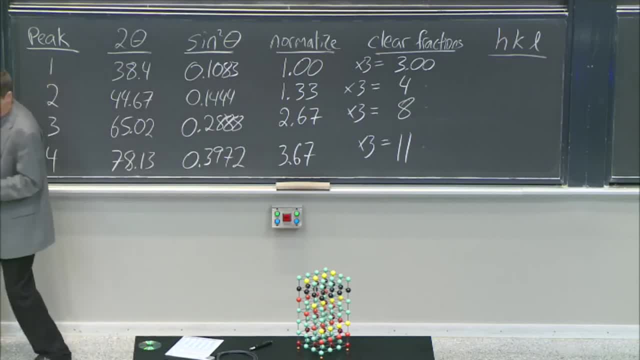 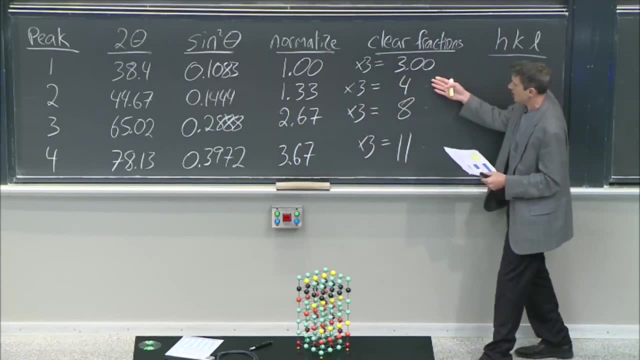 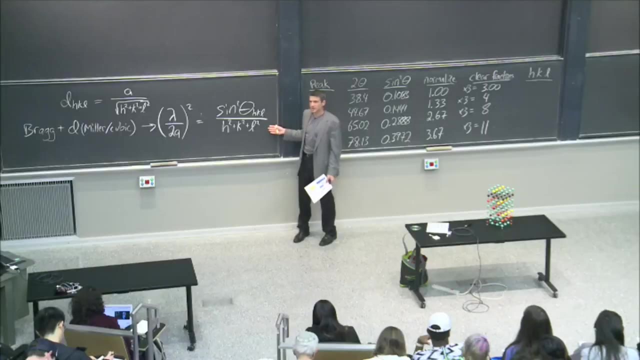 need to work with, because now you see, it's now you know, I hope it's kind of starting to make some sense If this, if I can get this to be h squared plus k squared plus l squared, well then I've done my job, I've kept this constant. 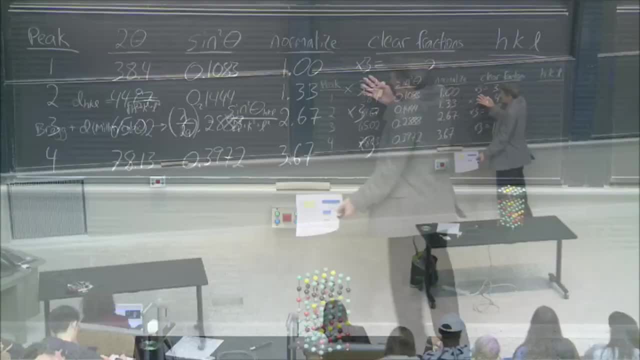 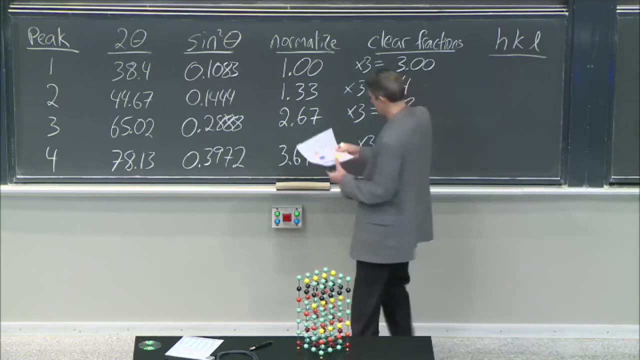 That's the trick, right. I've done my job. I've just made the math easy. If I can get h squared plus k squared plus l squared to equal these things, right then I'm keeping it constant. So let's see, what would that be? Well, here it would be so. 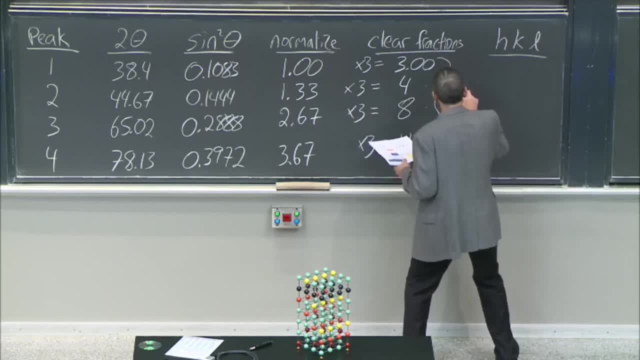 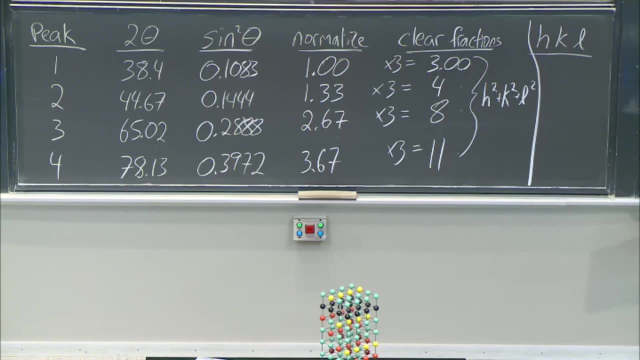 this has to be h squared, let me just write it here- plus k squared, plus l squared. okay, I want those to be an h squared plus k. So if I do that, well, this looks a whole lot like 1, 1, 1.. That works. and for 4, 2, 0, 0.. Okay, and for 8, 2, 2, 0. and finally for 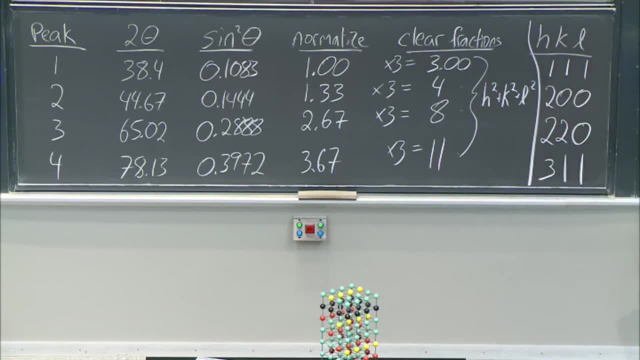 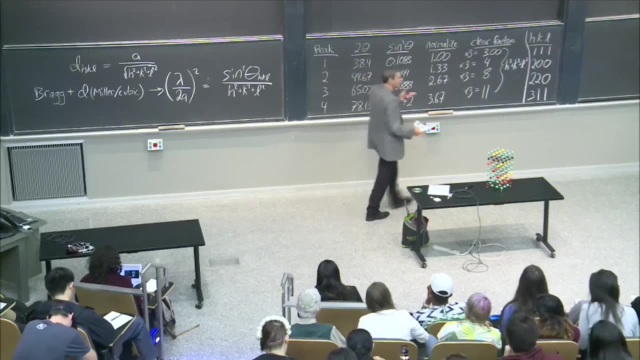 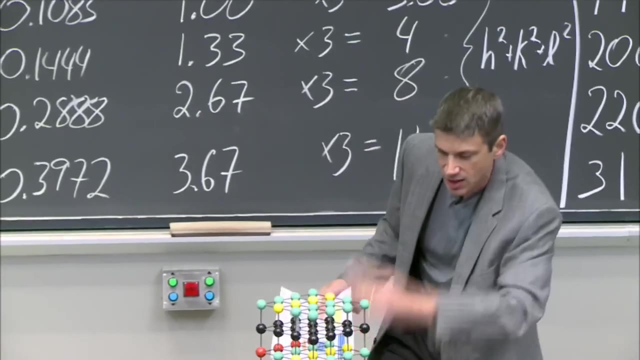 11,, 3,, 1, 1.. Oh, it's a beautiful thing. Okay, I've gone from angles to planes. These are planes: H, K and L mean one of these. It means one of those. 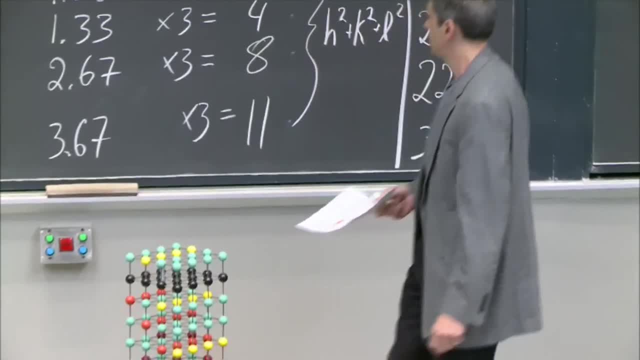 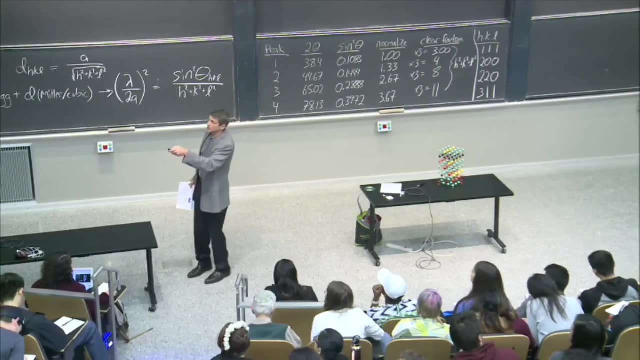 That's what it means. a set of those right, And I have found now which ones, literally which ones give me each peak. This peak is the 1, 1, 1 plane. It's X-rays bouncing off of that, reflecting off of that. 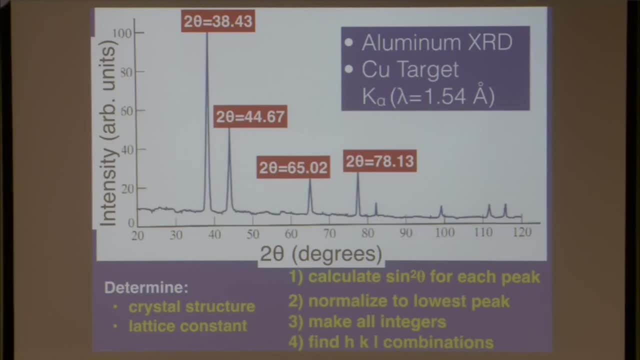 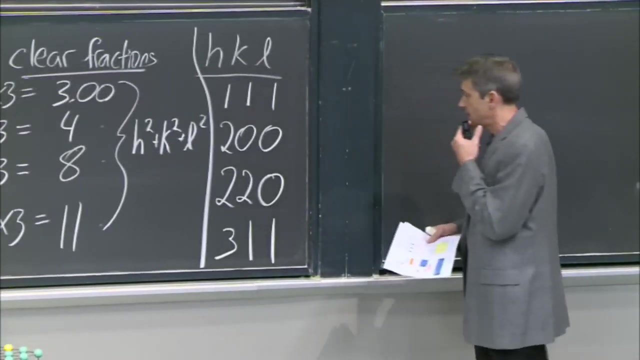 and the one below it and the one below it, and seeing where it gives you constructive interference and gives you the Bragg condition and therefore a peak. Okay, All right now, hold on, Hold on Now. okay, have we determined the crystal structure? 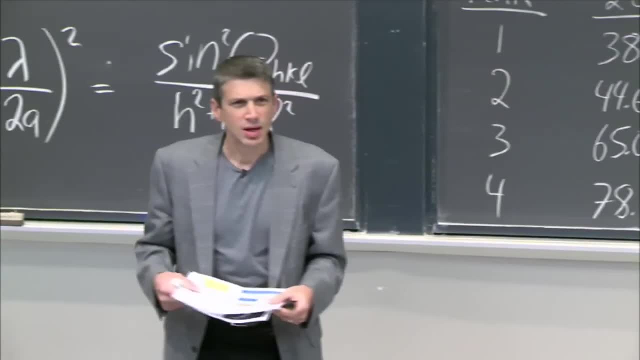 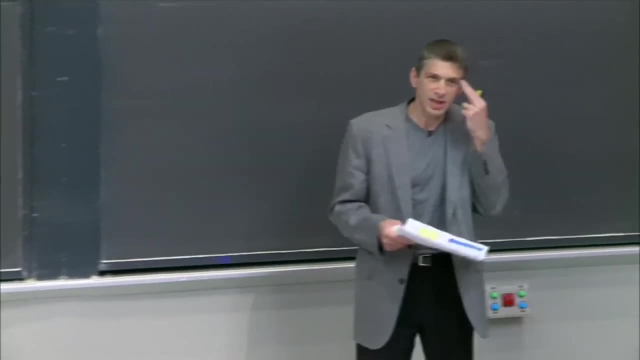 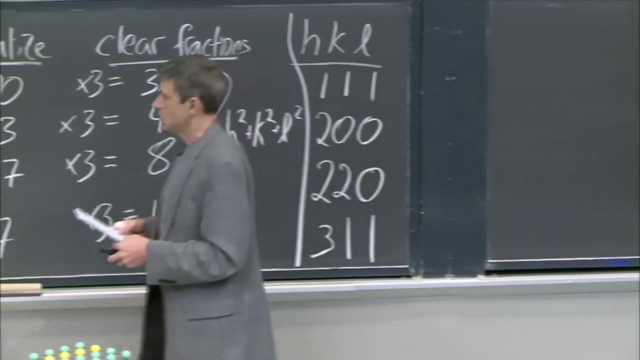 Have we determined the crystal structure? Can anybody? How do we get the crystal structure from this, From this Peaks? How do we get? Well, let's see, Okay, It it, could it. let's see, could it be? could it be BCC. 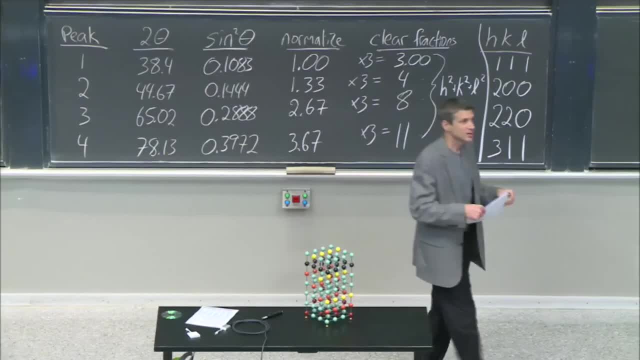 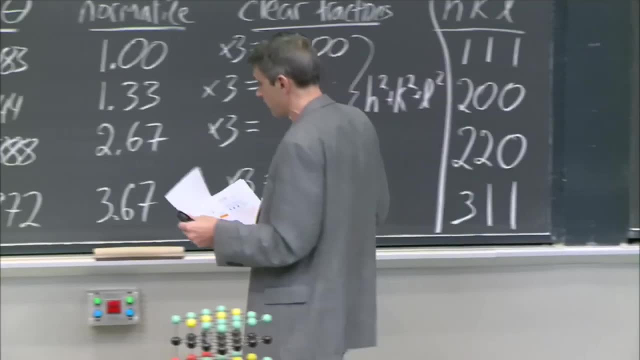 What? what else did we learn on Wednesday? right, What else did we learn on Wednesday? We learned about selection rules. You've got to remember the selection rules Those factor in, So let's write those down here Let's remind ourselves of. okay. 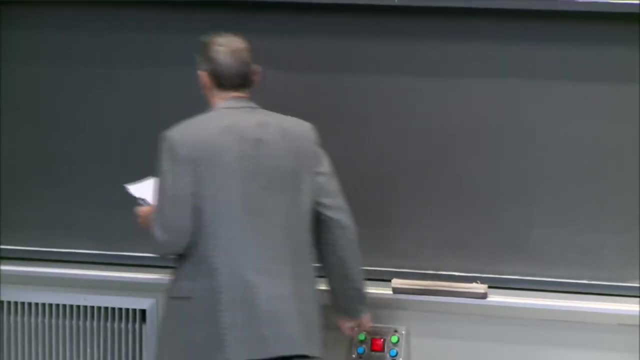 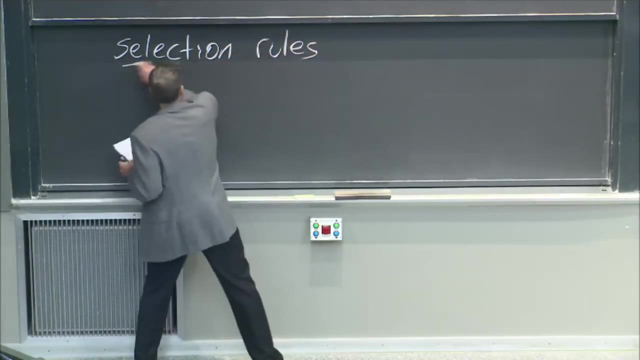 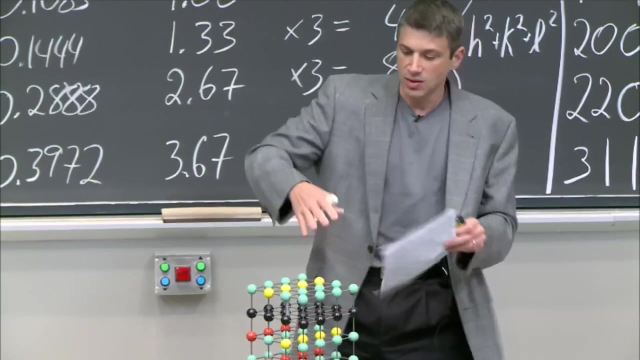 that's important. All right Now. I mentioned how this came about. I don't need you to know how to derive the selection rules, but I did talk about why they come about right, Because you could for some of these cuts. 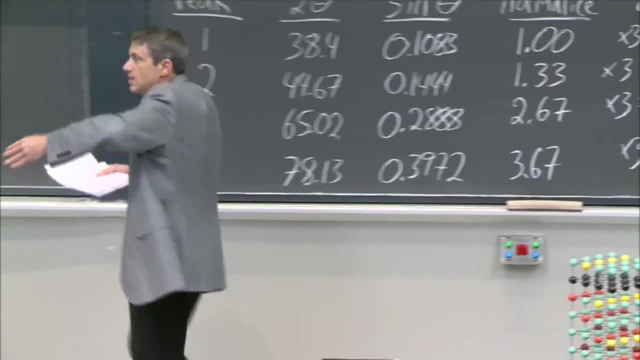 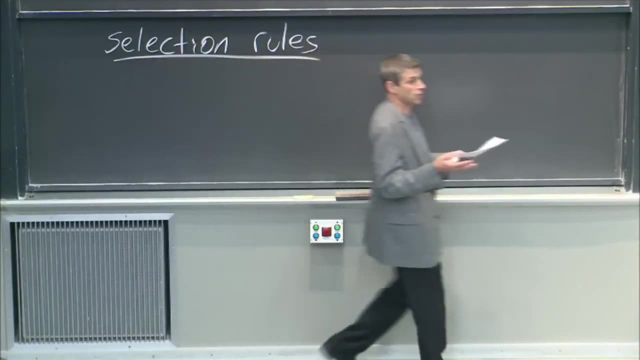 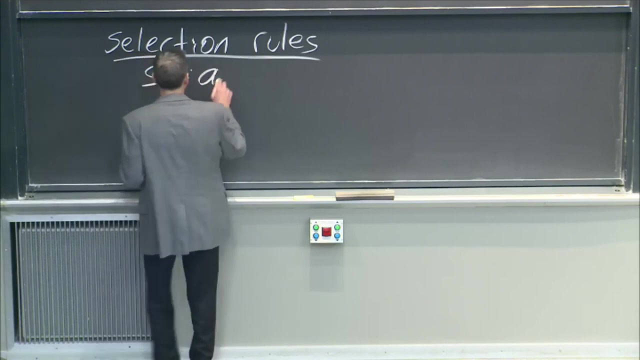 you could have a plane in between that destroys the signal. Okay, Depending on which, which crystal structure it is and which plane you're in. Okay, And you're talking about. and when it comes down to it, for a simple cubic it's anything goes, anything. 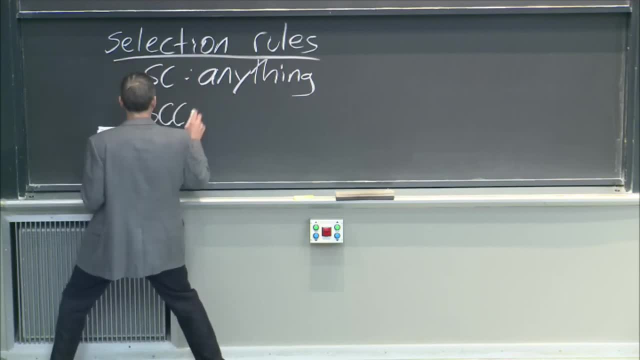 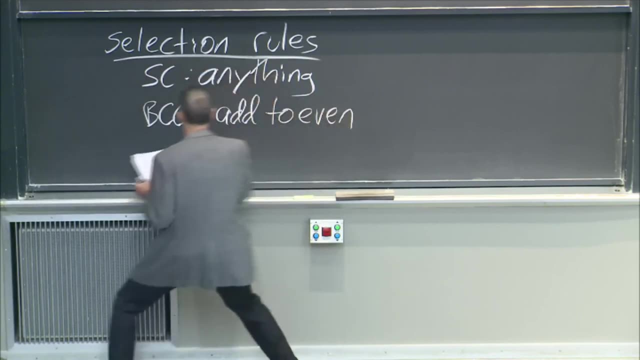 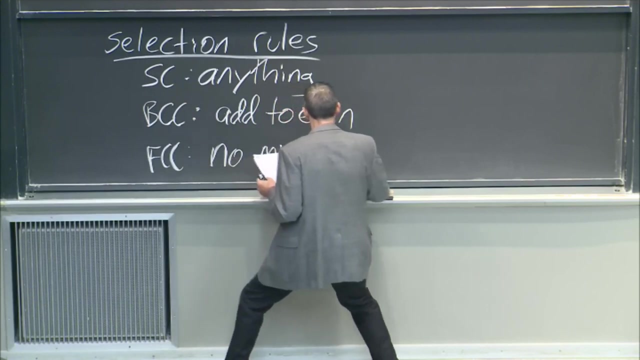 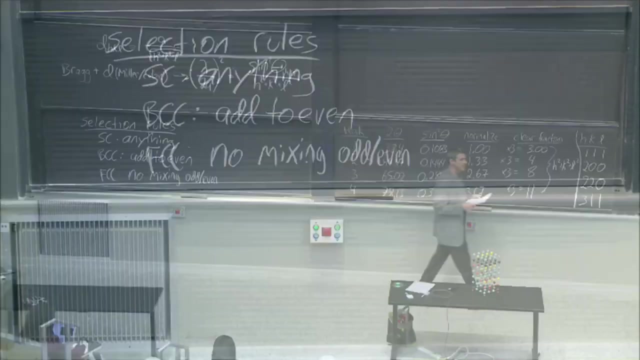 Oh, polonium. And for BCC, it's adds to an even number. And for FCC, no mixing, no mixing of odd and even. Those are the selection rules. You don't need to know how to derive them, but I do want you to know what they are. 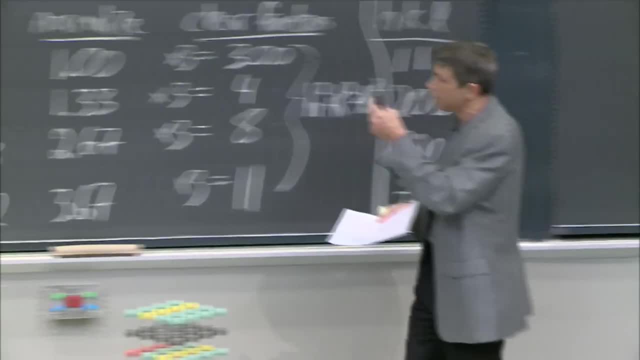 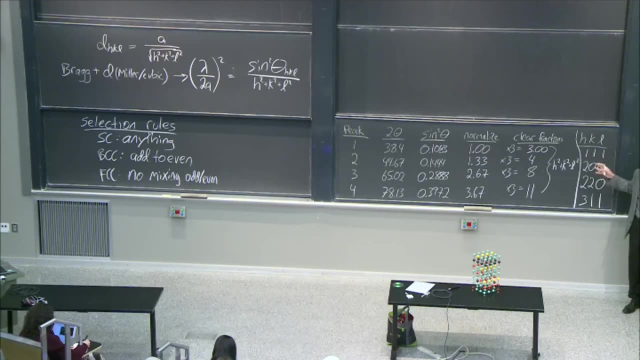 Those are the. so now we can see. well, okay, hold on. If this were a BCC crystal and they had to add to even one plus one plus one is three, bam, it's not BCC, right Yeah? 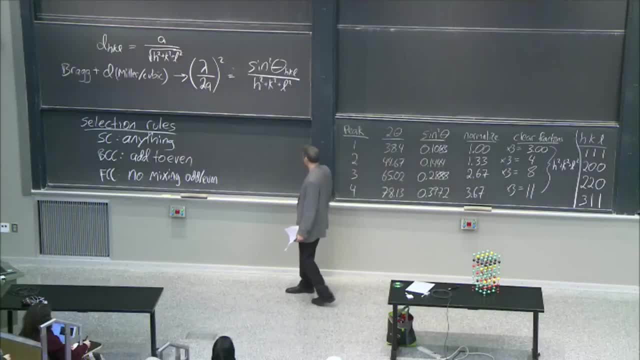 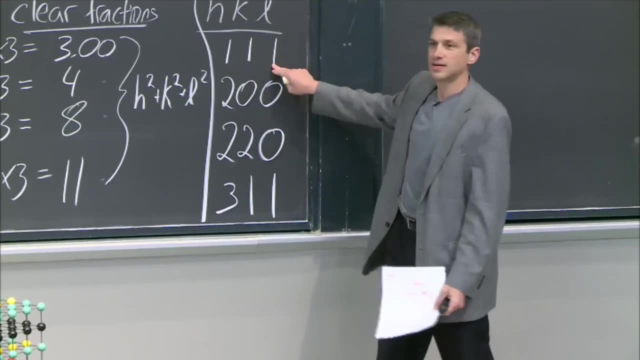 Okay, Yeah, But. but. but now hang on, If it's no mixing. odd even, did I handle that one. Okay Yeah, Odd, Even, Even Odd. This looks like an FCC crystal to me, right, This looks like an FCC crystal. and I can go even further. 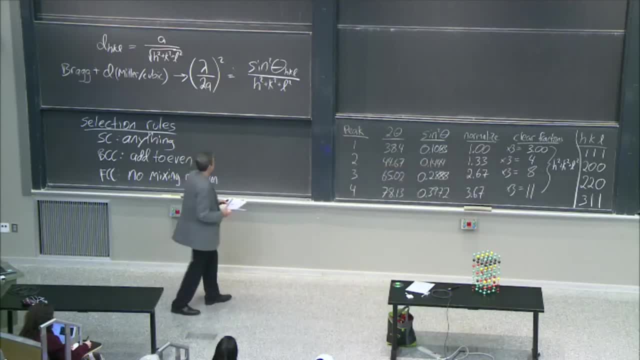 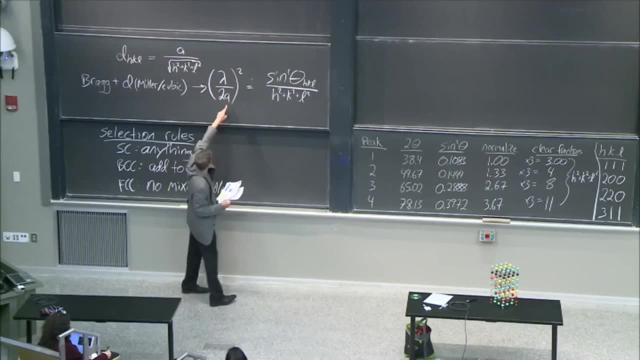 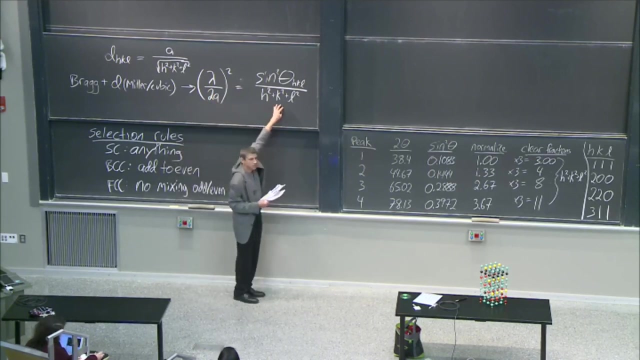 I can calculate the lattice constant. I can calculate the lattice constant cause. it's right here, It's right here, right. So that's the lattice constant, That's a number, that's a constant Lambda. So I could take any one of those planes, any one of those. 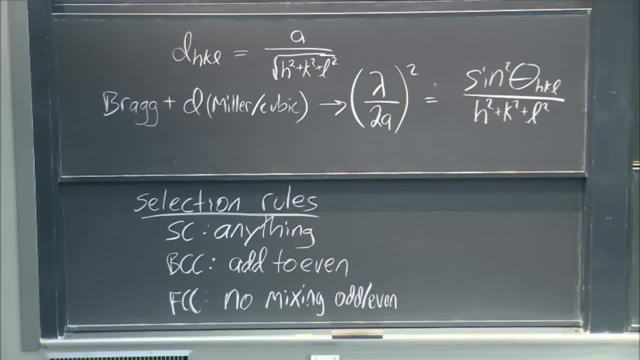 any one of these four peaks And I, and if I, if I did this right, if I did this right, they better give me the same lattice constant, and that's actually the last step in the recipe that I put the right. Yes, 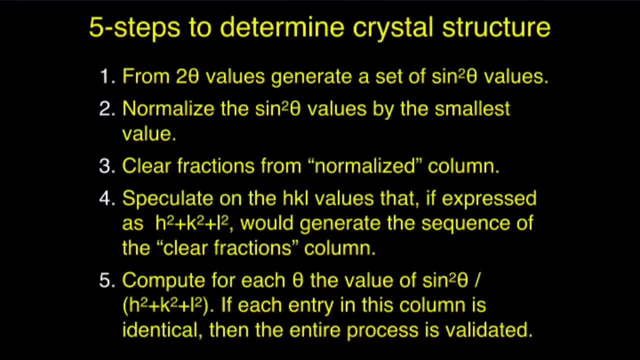 All right, This is the recipe I gave you on on Wednesday for you all to become crystalographers: x-ray diffraction nurse. That's okay, We'll make it work. You're x-ray diffraction nurse And, and the thing is, you got to remember how powerful this is. 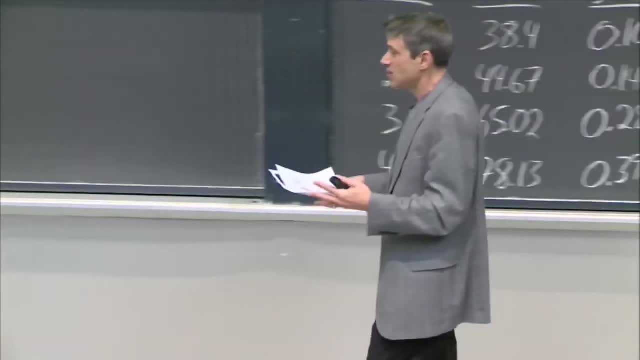 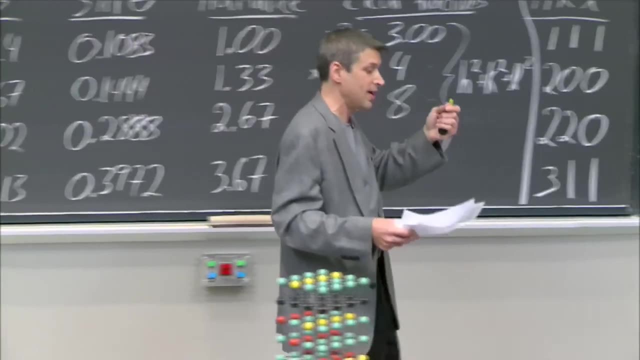 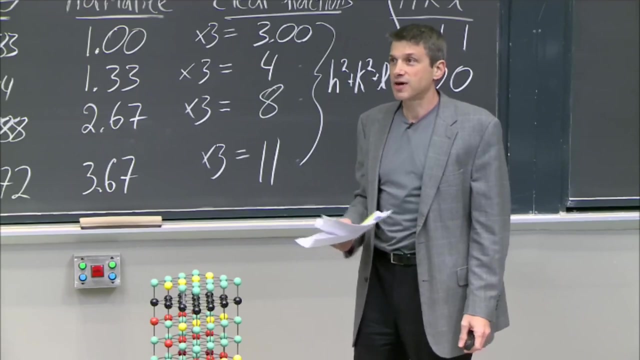 How powerful this is, because you we've learned about perfect crystals and now we've just gotten the single, most, one single most important way to figure out which one we have: we shine x-rays on it and we look for diffraction peaks. That's it. 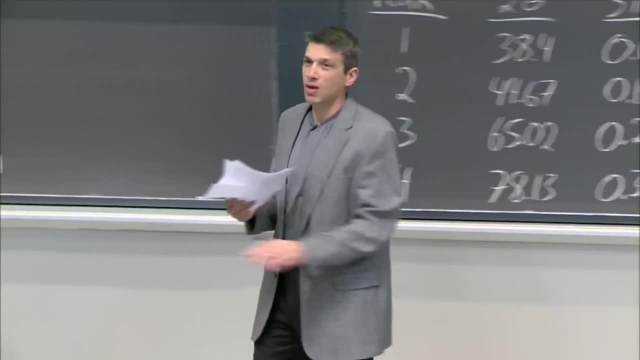 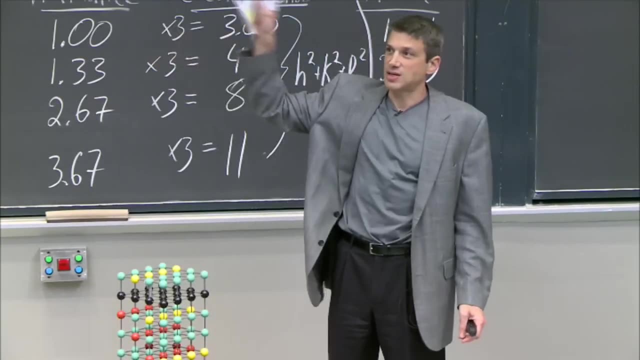 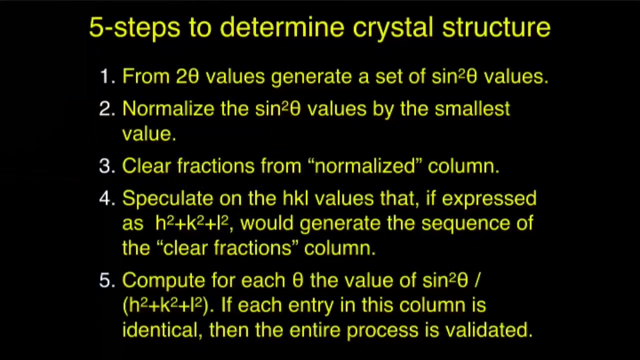 This is a very powerful tool and it is used all over the place in, uh, in materials, chemistry, physics- you name the field- x-ray diffraction is a starting point for characterizing the crystal. And so the last sanity check that you want to do here, because it'll help you, make sure you did. 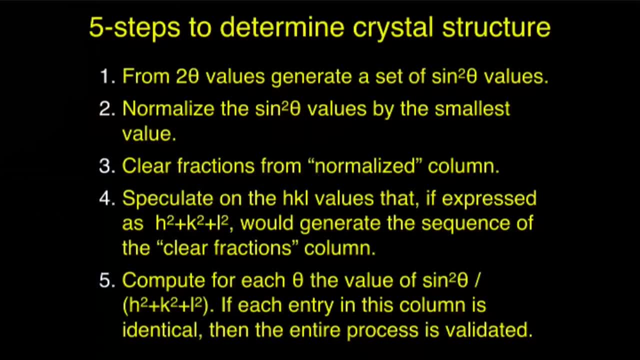 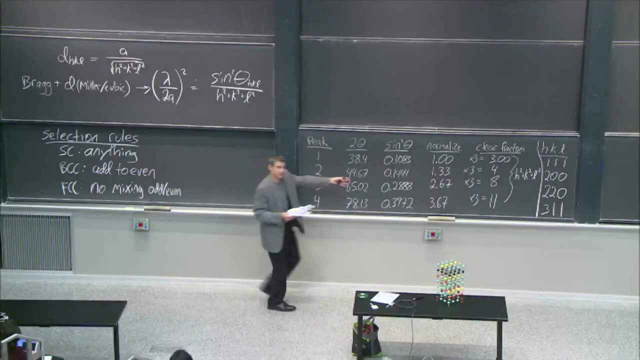 these points correctly is: compute these values, because you know this. this is it right? Sign: squared over a. squared plus K. squared plus L squared better be a constant. If it's not, then you've done something wrong in this analysis, right? 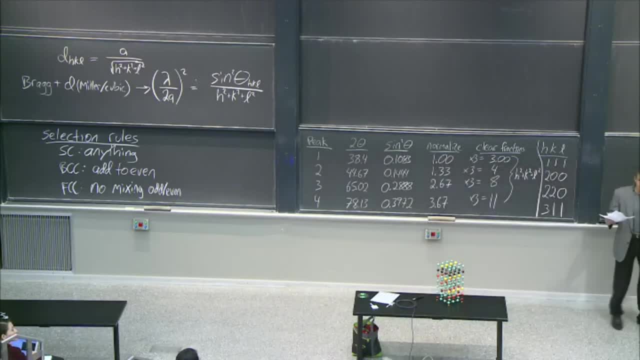 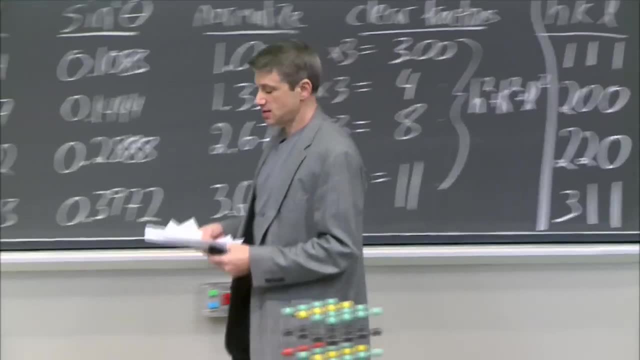 Right, We, you could just calculate the lattice constant for each piece. It's weak, and they also better agree, And so I won't do that. but it turns out we did it right. for each one of these, That is indeed a constant. 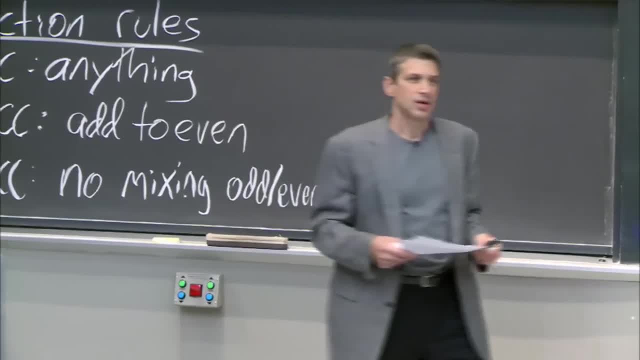 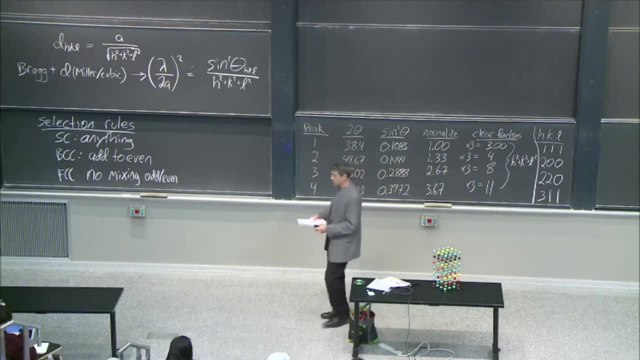 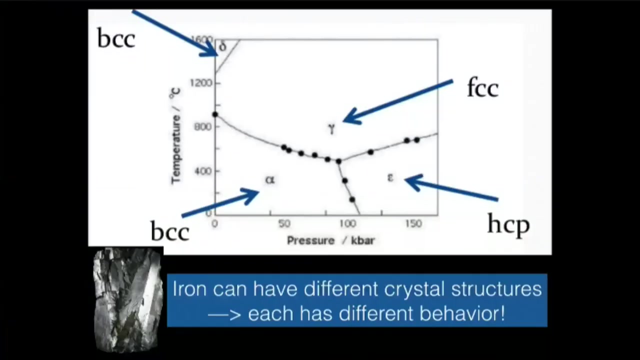 We have achieved our goal. with great power comes great responsibility. How you use XRD. how you use XRD, Well, let's see. let's use it to figure out what phase of material we have. But this is, why does this matter, right? 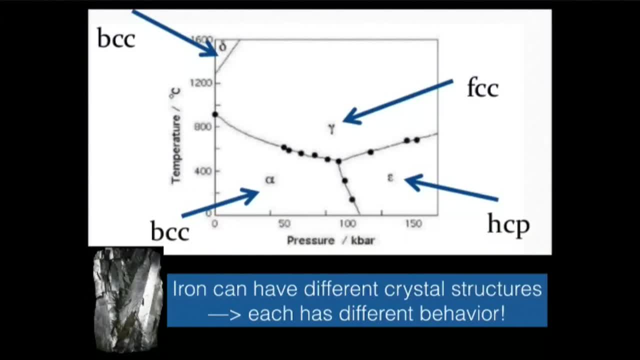 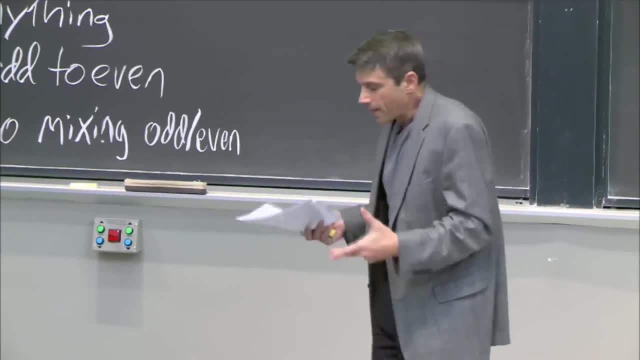 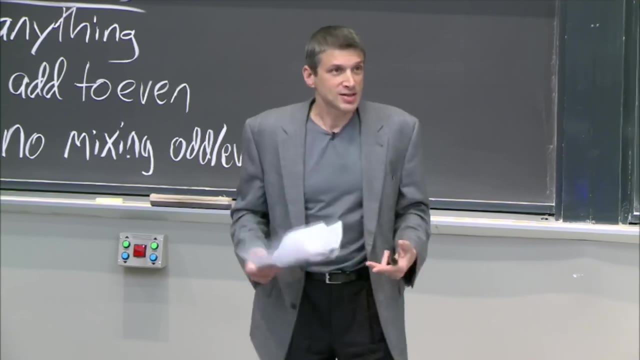 Well, I have a why this matters, but but there's multiple reasons for why this matters, as, as I think we talked about. you know, the properties of a material depend on the chemistry and the material, but they also depend on the structure of the material, and we're making solids. 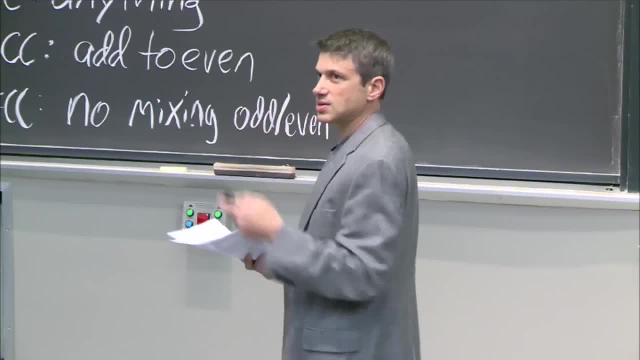 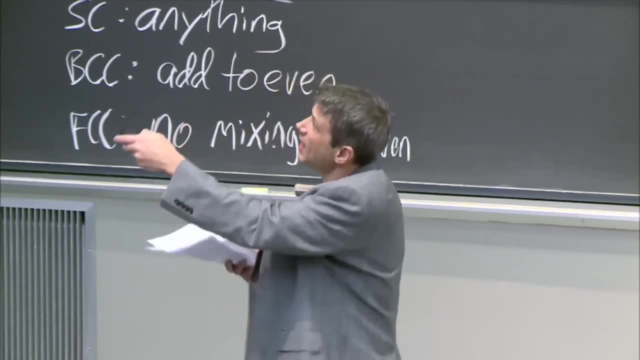 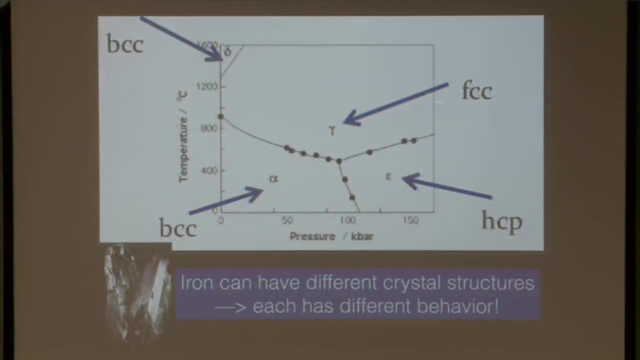 So those structures are crystals until next week when we destroy the crystals by putting defects in them. but for now they're these perfect crystals and they have this kind of repeating pattern. Don't worry about HCP. Ah, we're comfortable. FCC, comfortable BCC. 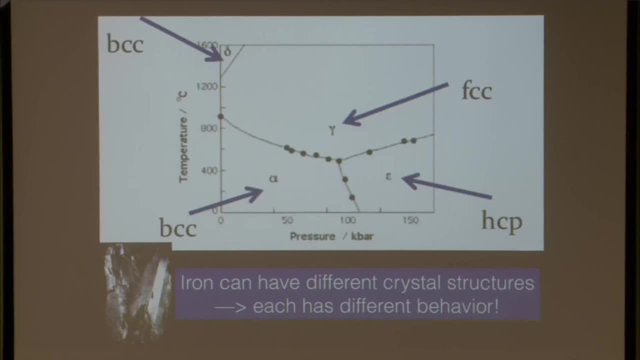 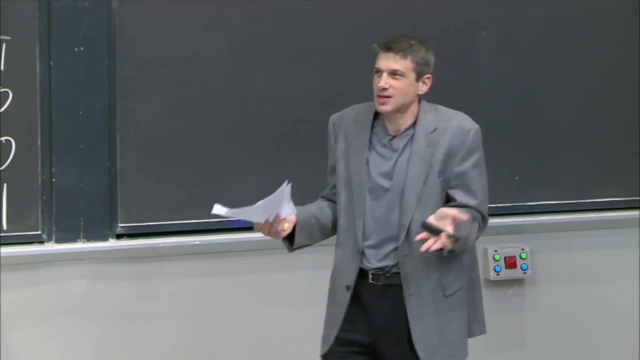 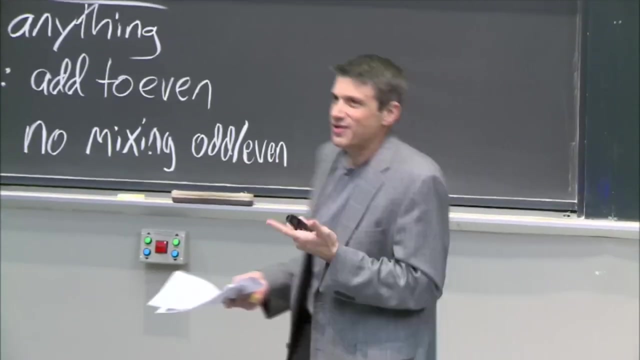 Now, this is called a phase diagram. This is called a phase diagram. These diagrams will be on the quiz next week. I'm kidding, They're not going to be on the quiz because this isn't a class about phase diagrams, but but I want you to know. I want you to know what a phase diagram is. 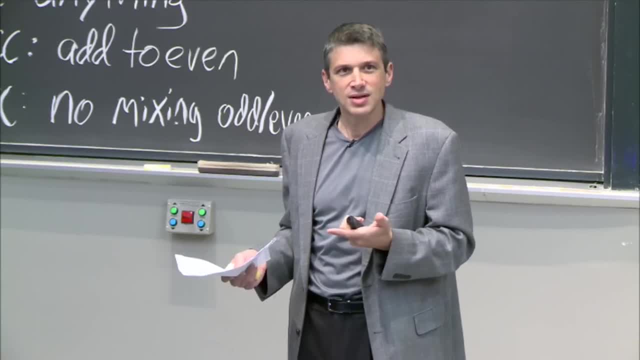 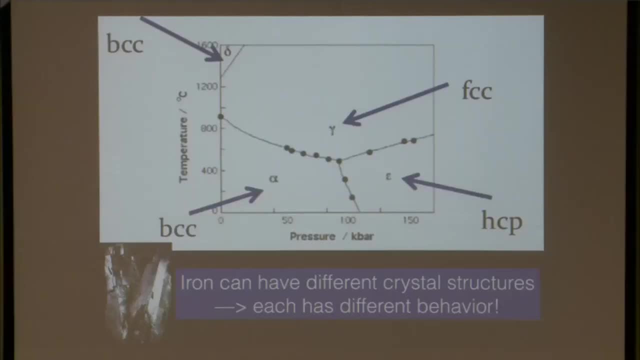 It is a map of materials. It is a very important. it is like a treasure map, literally treasure map Because you find I need iron to have a different property. Oh, if I go to this pressure and that temperature, aha, it can have a different property. 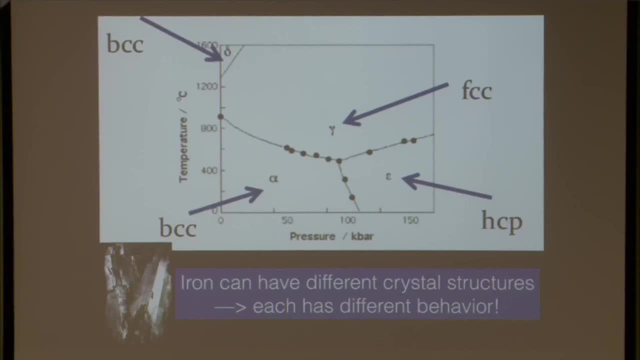 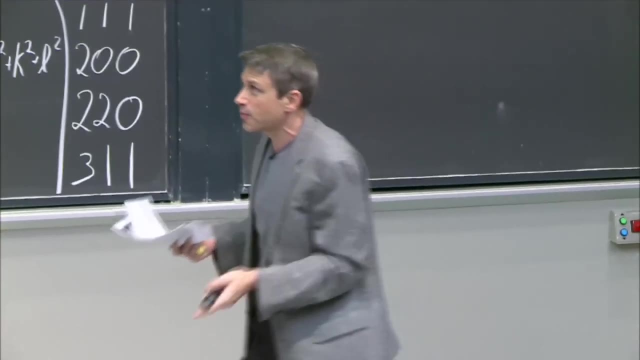 Why? Because it has a different crystal structure. So the crystal structure of something- in this case it's iron- depends on the pressure and temperature, and the and the properties depend on the crystal structure. So we've got a way now to change materials. same element: 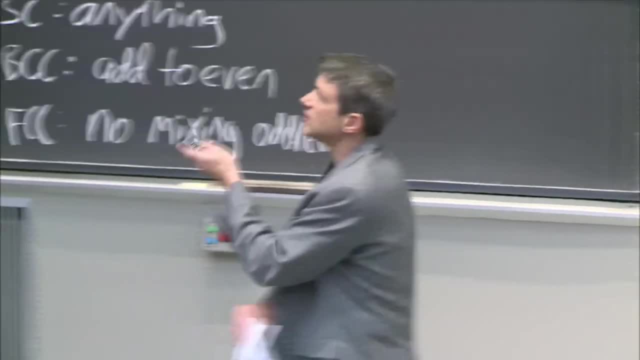 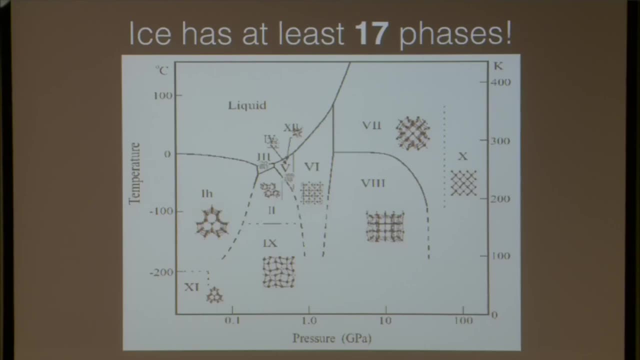 I'm just changing its structure. I love this one. This is water. Now You, You know, don't worry about how complex this is. Actually. the whole point is it's complex. This is the phase diagram of water. Now, this doesn't even have them all. 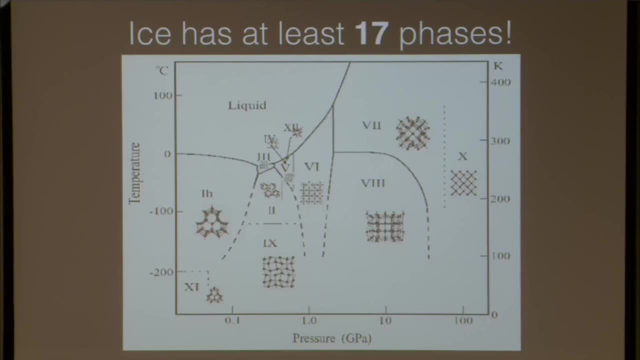 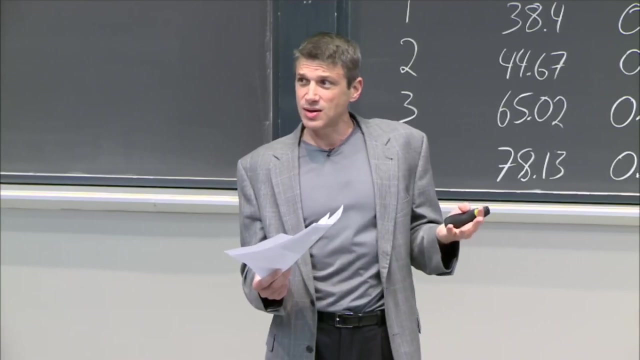 There are 17 current phases of ice, 17 different crystalline structures of ice. That is incredible. right Now you you can actually imagine why from your knowledge in this class. already Those are hydrogen bonds. They're kind of strong, but they're not too strong. 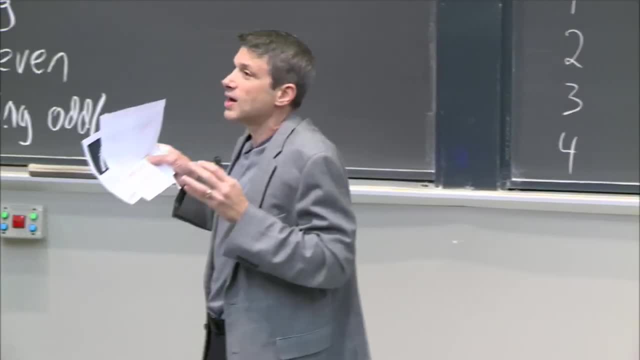 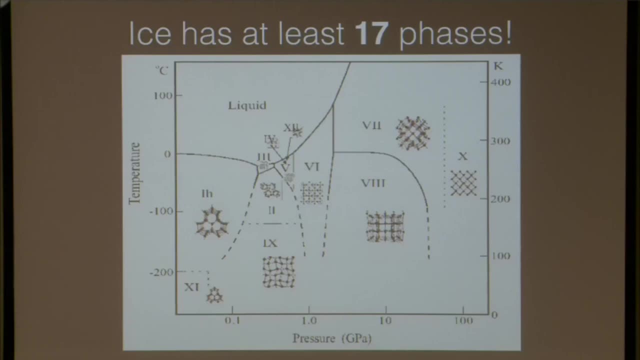 There's a lot of ways that those water molecules could form a Solid, And they do, 17 to date and counting. but see, and this tells you which one you have now, earth's operating conditions are right around here and that's a really good thing, because there's a liquid phase and there's ice. 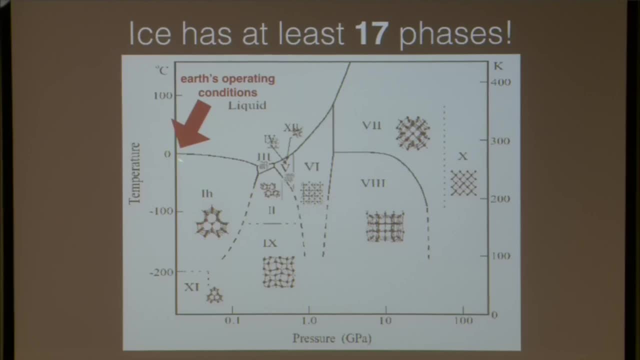 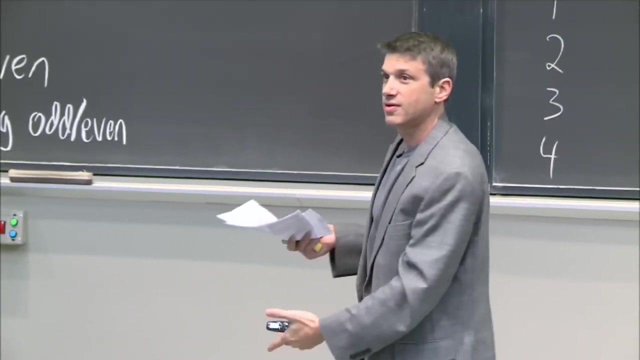 One is here, I H is ice one, and it's a really good thing because of the fish, because if you, if it weren't ice one, then when it freezes it wouldn't have, you know, a different density and the ice wouldn't float to the top and the fish could still live, which they do in the winter. 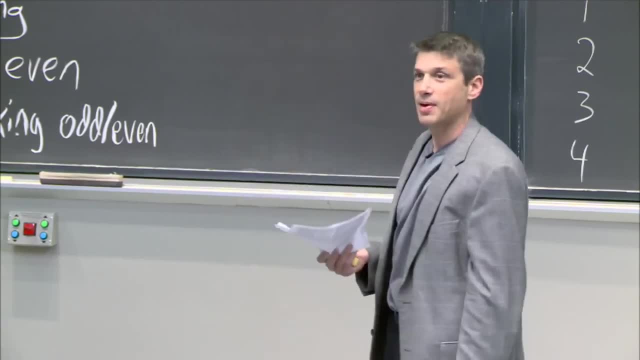 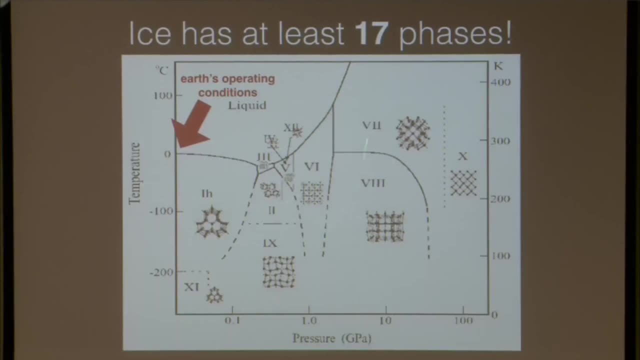 Because you don't freeze from the bottom, you freeze from the top. that's because it's ice one and not ice eight. it would be terrible, right, But yet we know about these. and how do we know? we know because of crystallography, we know because of XRD, we can figure out. yeah, if you're out- and maybe this is, it's a Friday night, so maybe this is a good idea, it's a good time to mention it- you might get ice in your water out at a restaurant. 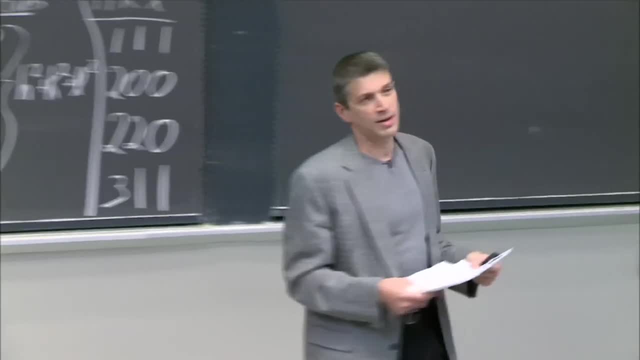 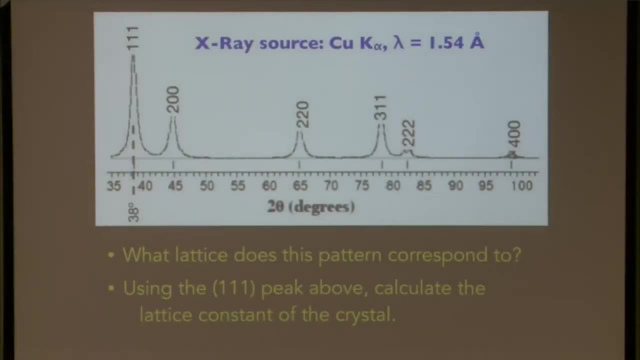 How do you know which kind of ice it is? Talk about XRD as the only real way to figure out which one of these you really have. Okay, So, for example, if I were to think of other types of problems you might get. well, here's a good one. 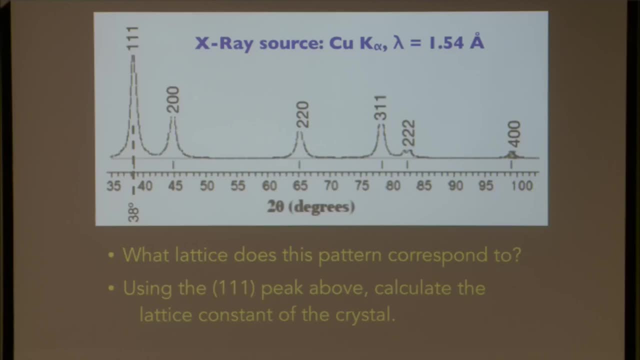 Okay, here's a good one. So this is an X-ray diffraction spectrum and I give it to you and I don't even tell you what it is. Why is that? Here's a pattern. I put something in there. I measure these peaks. 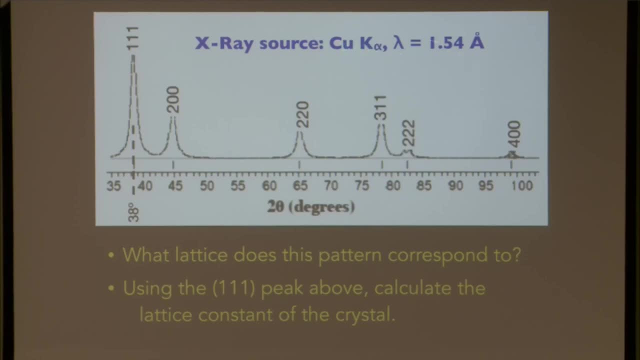 And I tell you the source: It's the K alpha line of copper, so that's the wavelength of the source. First thing is: what lattice? what symmetry does this correspond to? Is it simple cubic, body-centered cubic or face-centered cubic? 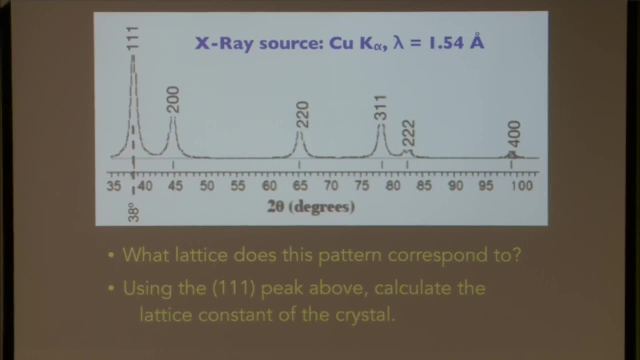 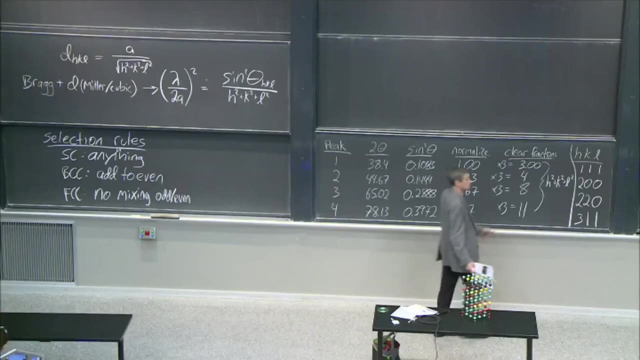 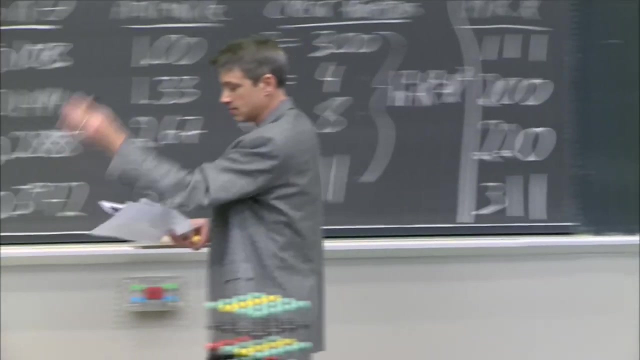 Can we get that? We can get that because of the exact same thing that we just talked about. right, Okay, This cannot be. if it were simple cubic, you'd see the peaks, But no, some peaks are forbidden, so they don't show up. 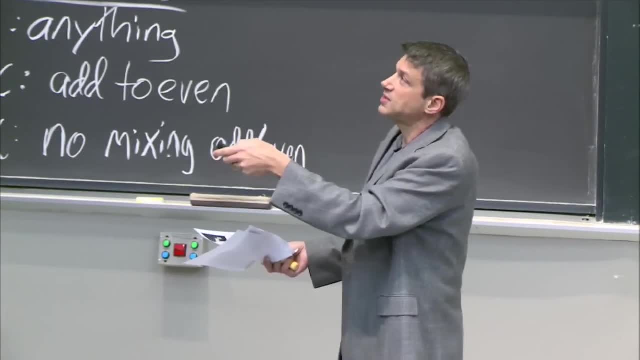 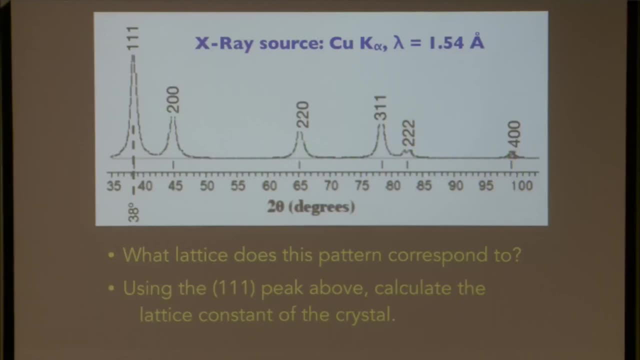 Right And you only get peaks that look like an FCC. according to our selection rules, No mixing odd. even That works. So this is an FCC crystal. So I've already learned that. And then I say, well, what's the okay, use the 1, 1, 1 peak to calculate the lattice constant. 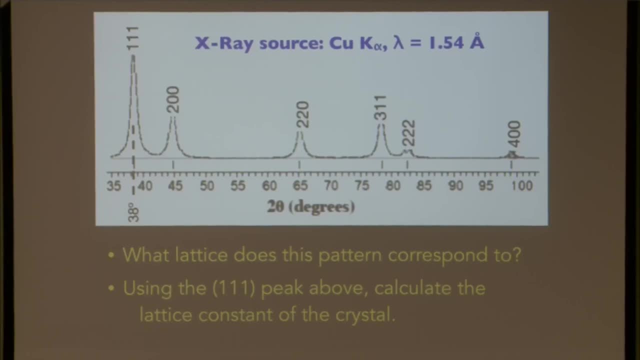 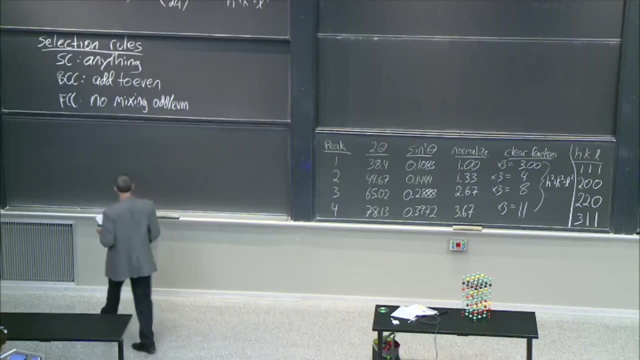 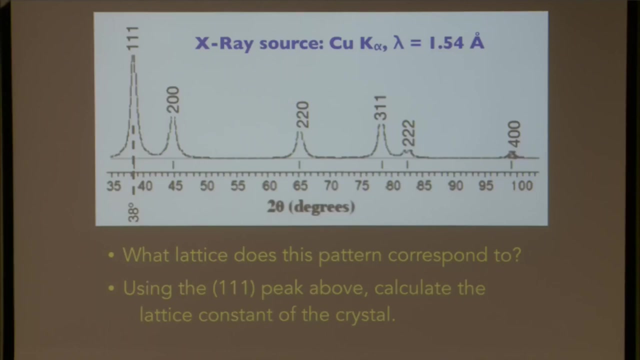 Okay, Well, we can do that Right. So if I were to, the 1,, 1, 1 peak is even labeled there. It's 38 degrees, 38 degrees, And so 2 theta is 38 degrees. 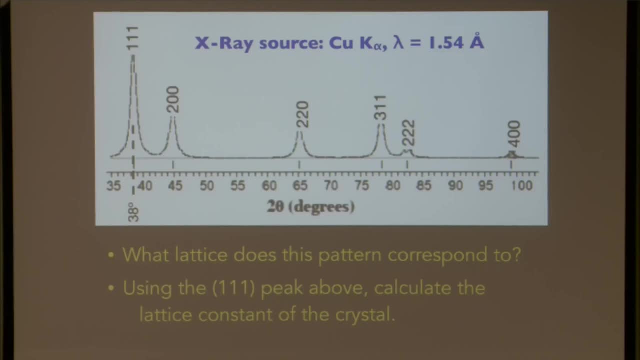 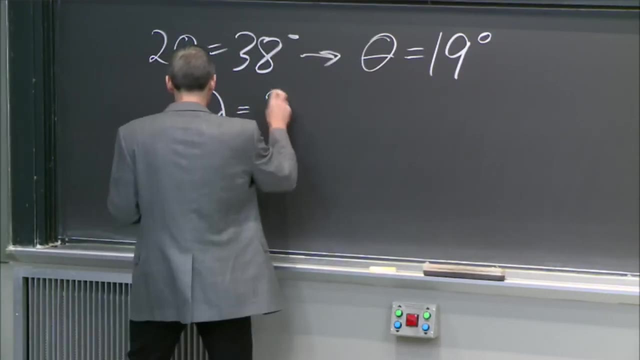 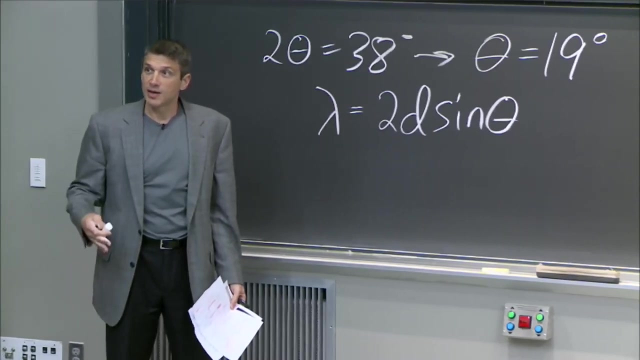 So that means that theta- okay, I can do this one- is 19 degrees. Okay, Now, oh, from Bragg, Lambda equals 2dc Sine theta. But look, label, label the plane. This corresponds to a plane. 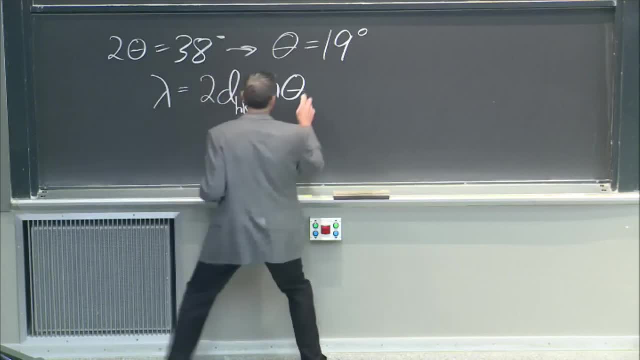 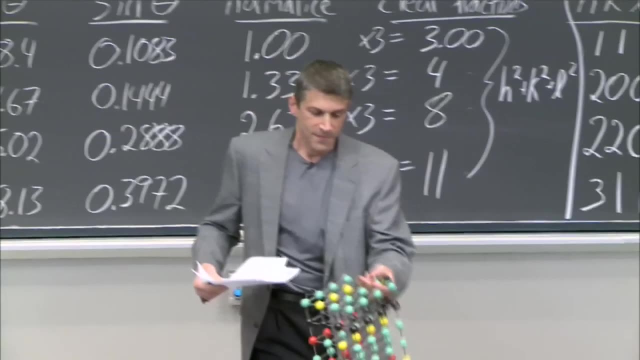 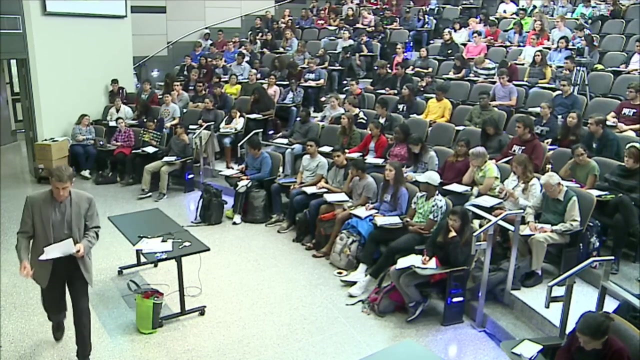 So some distance between some planes corresponds to some angle. that gave me constructive interference for those planes. Let's pass this around so you guys can look at these planes. They're beautiful things. Now that means that if I, if I look at the first peak, I know what well I've labeled. 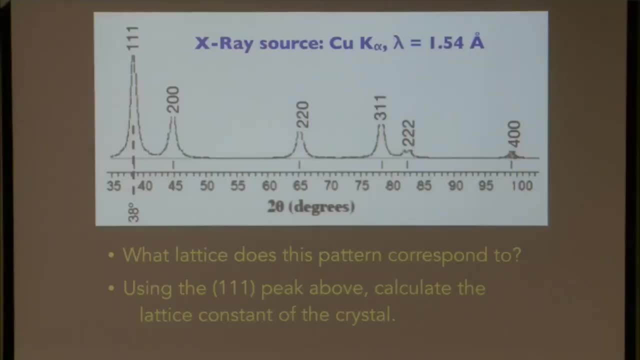 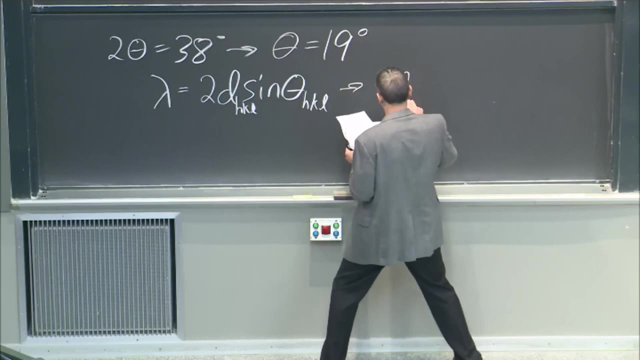 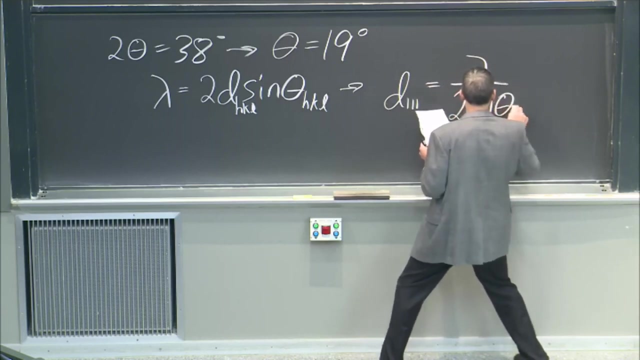 them here. In the last one I didn't, And you want to find those Here. I'm giving you the planes. So if I do that, then d 1, 1, 1 equals lambda over 2 sine theta. 1, 1, 1, which equals 2.37. 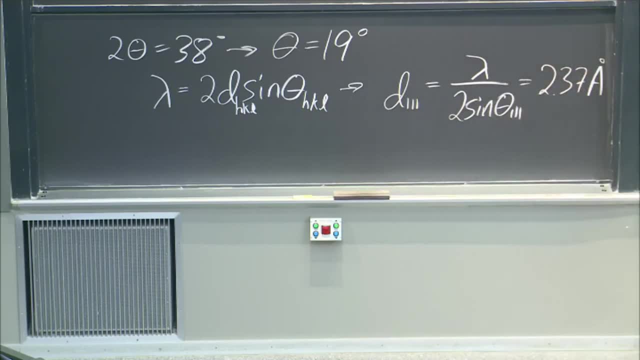 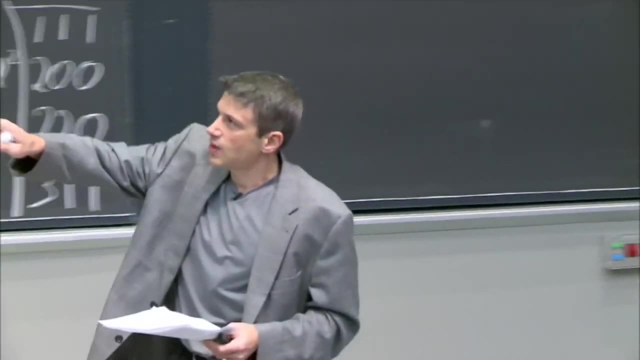 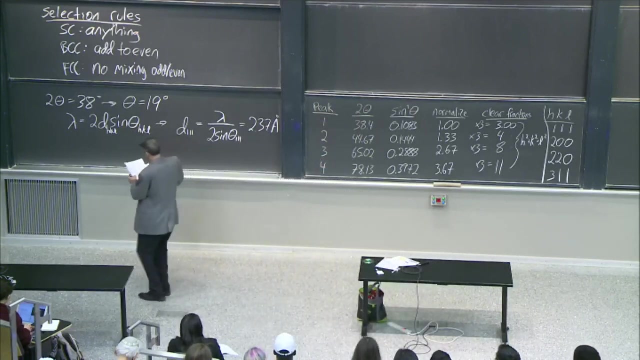 angstroms. Okay, Have I answered the question? I haven't answered the question yet Because You see the the question says: what's the lattice constant? Well, but, but I'm very close, The lattice constant. the lattice constant is related because of Miller. 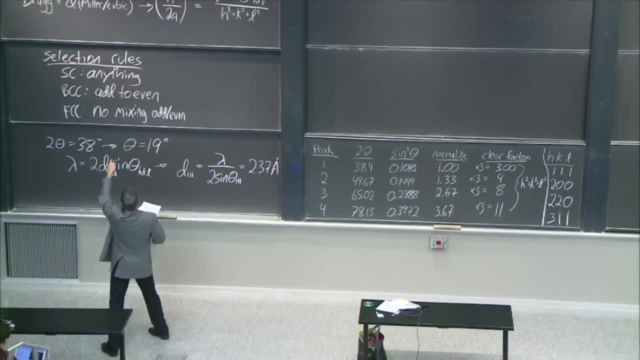 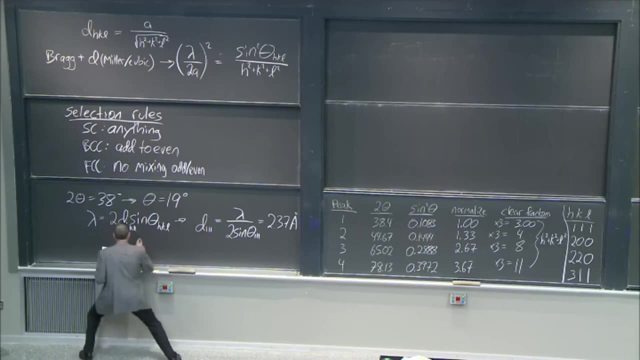 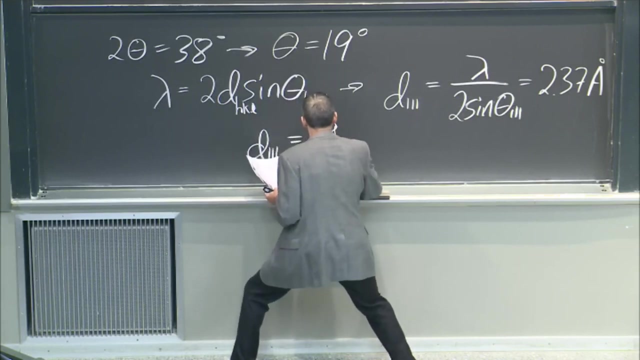 The Miller planes equation for lattice, Lattice, constant distance between any planes. Oh, this is all just coming together, And so d 1, 1, 1 is equal to a over root 3. And so a equals 4.1 angstroms. 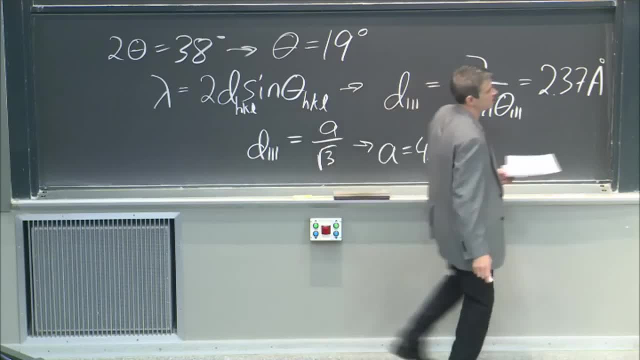 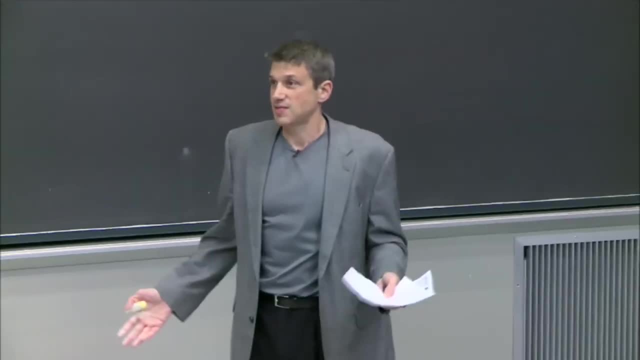 Oh, you can go even further And you you can figure out now that you know it's FCC. it's a single atom basis, FCC crystal. you could actually figure out the atomic radius. I got a and I know the closed pack direction. 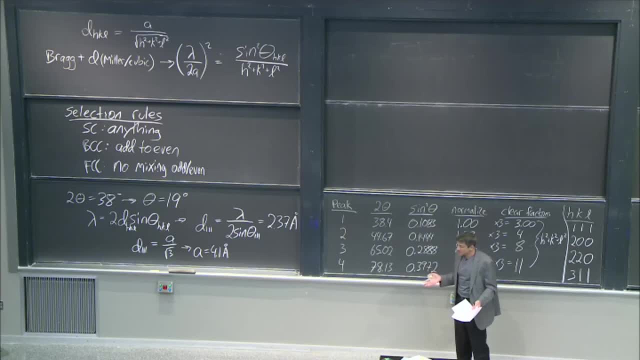 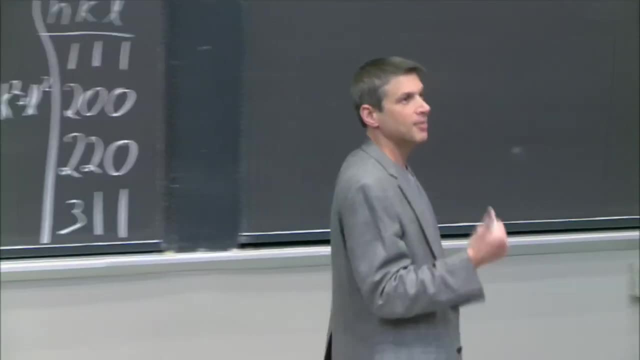 All right, I could actually figure out the atomic radius and I could go into my periodic table and figure out what I have. But I can't figure out the atomic radius. What do I have Just from the? the atomic radii listed in the periodic table and the crystal structures. 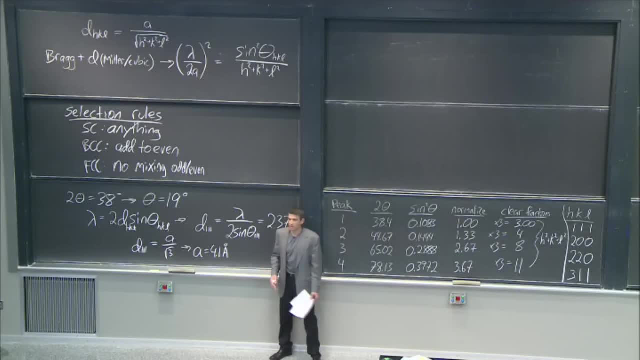 FCC, atomic radius. which one is it? It's gold, It's gold. So this is the kind of thing that you guys now have the power to do. You have the power to do this. You can go back and forth between you, know, based on your knowledge of crystals. and now, 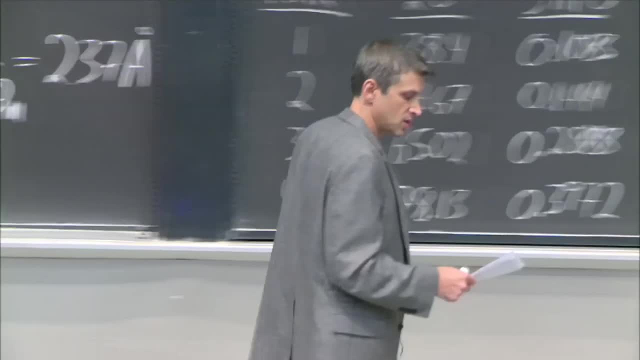 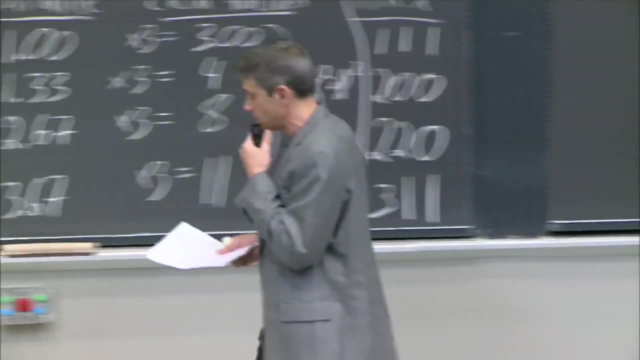 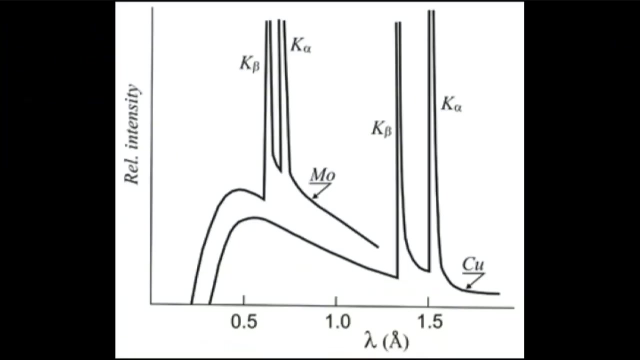 your knowledge of x-rays and how x-rays interact with crystals, You can do this Now. oh, that went too far, Now okay. So now I'm going to get to the the why this matters. So there's two different sources, two different targets. 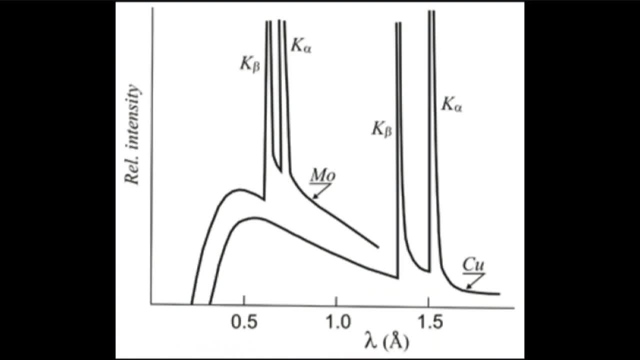 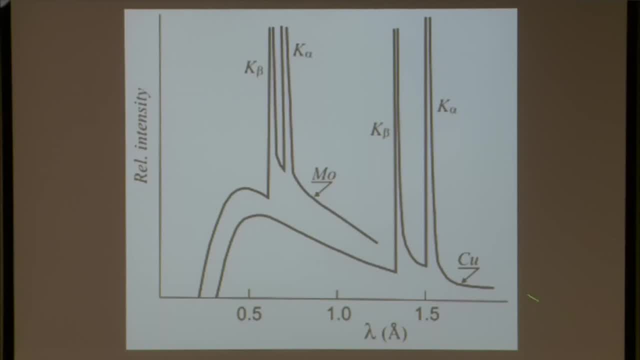 Remember we call them sources or targets. And and notice, okay, copper has. they both have this continuous radiation And- and I will talk about that- The Brinkstrahlung. We'll end with a discussion in a little bit. 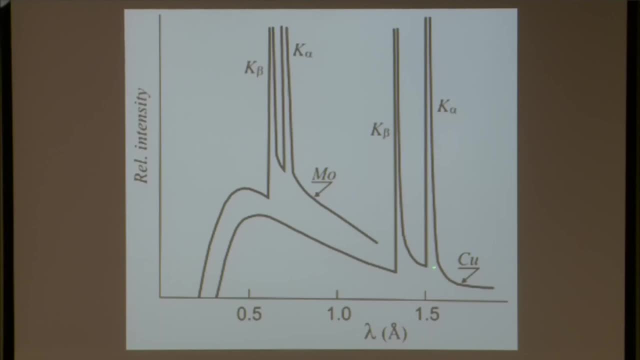 But on what you can do with that. But for now, let's keep focused on on these lines, These discrete characteristic lines. So there's the K-alpha for molybdenum, There's the K-alpha for copper. 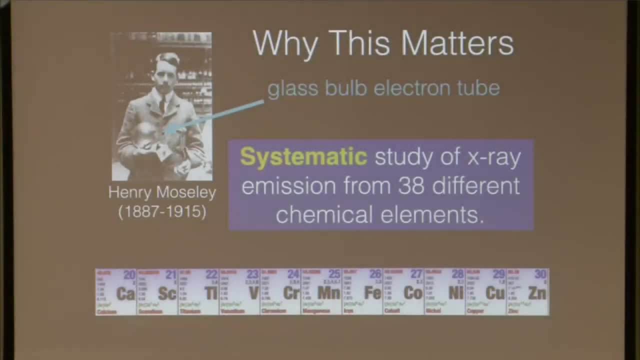 Okay, Now Moseley. Henry Moseley was a brilliant scientist And he was working with Rutherford and others, And, and, and he was really interested in looking at the trends And so so, So he took all of these elements. 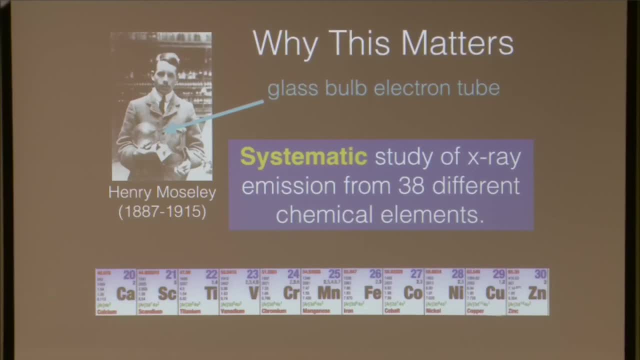 So from calcium all the way to zinc, 20 to 30.. And he said: I want to look at the K-alpha lines of all of these. I want to look at the K-alpha lines of all of these And what he found was extraordinary. 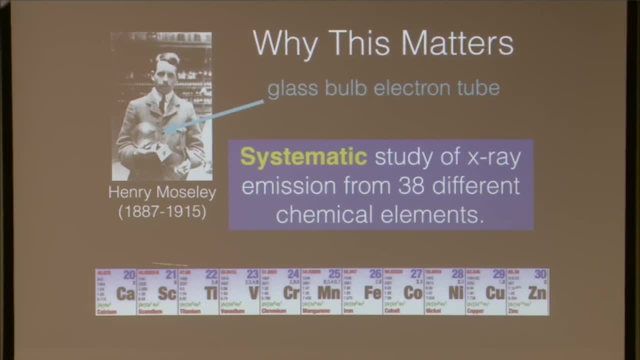 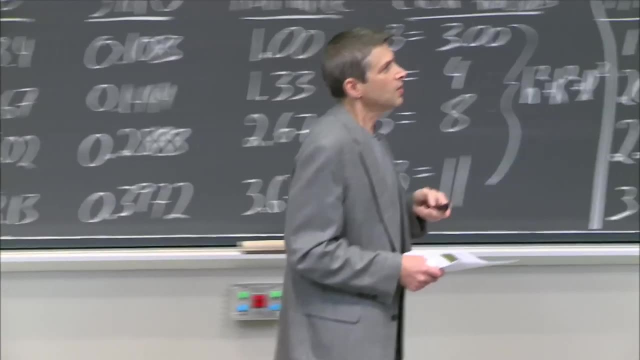 He did. he did more: 38 in total, But I'm just going to show you his data for these. Okay, And what he did was was absolutely profound, Because what he noticed, And there are the lines, 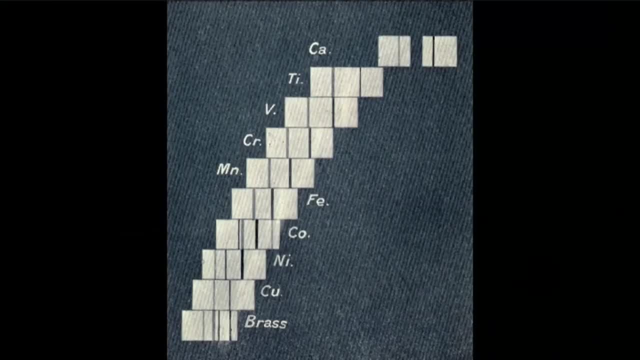 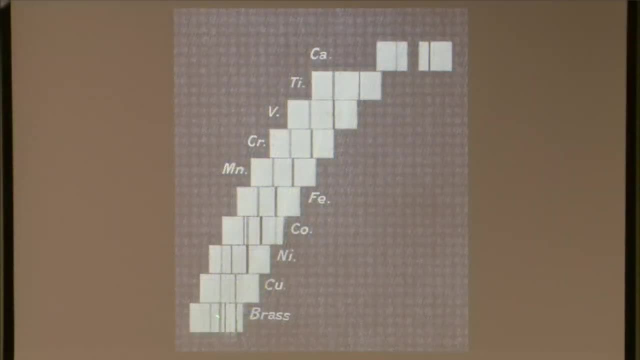 These are actually his measurements. Okay, These are his K-alpha lines And what he noticed in going from calcium down to, oh, brass. Okay, We'll talk about that in a minute. It's supposed to be zinc, isn't it? 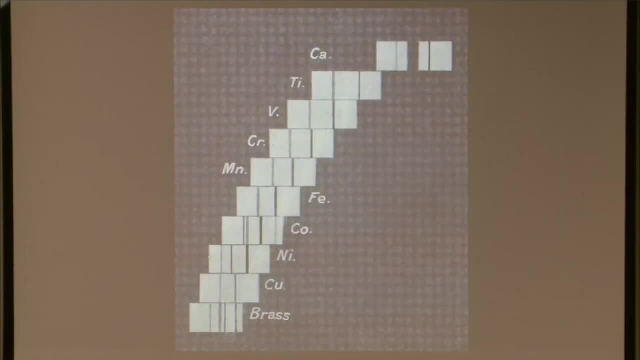 Why is it zinc? Well, why is it not zinc? Let's think about that later, But for now he noticed that this has a square root relationship to the energy. So so Moseley came up with In 19,. he was working on this in 1912.. 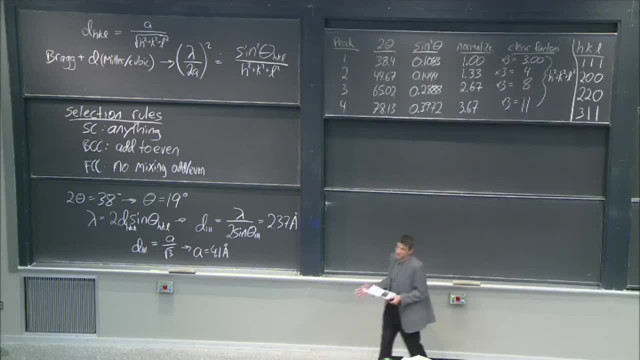 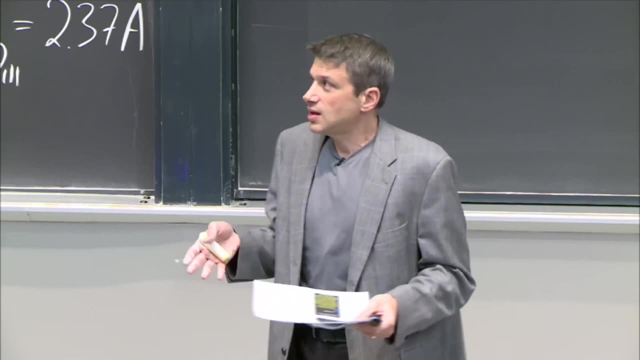 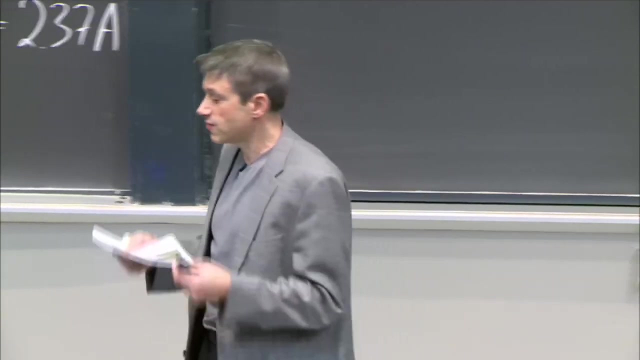 Okay, You got to remember 1913. Right, 1912 is when Rutherford did the gold foil experiments. It had been 44 years since Mendeleev put his periodic table to to paper Right And and published that. 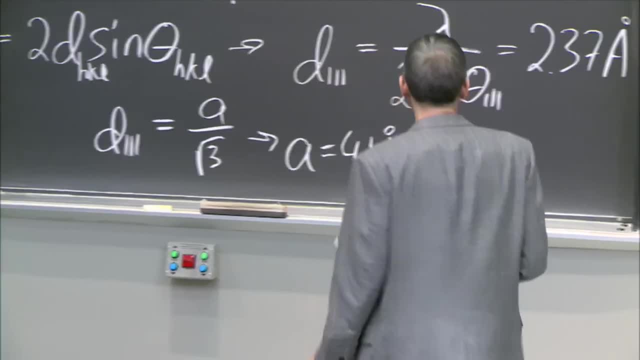 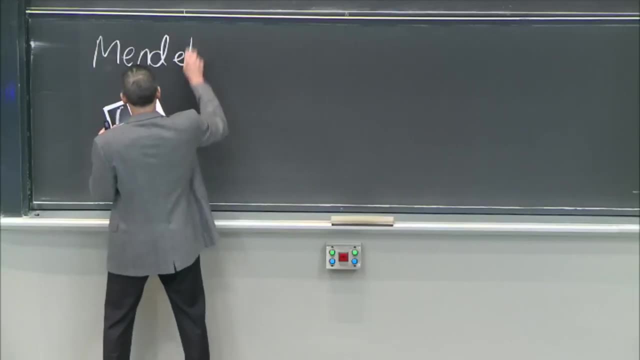 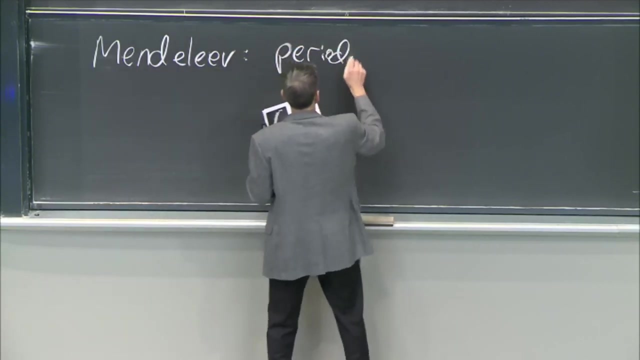 So for 44 years we had a periodic table? Yeah, But, but you see, the thing is, there was a huge problem with the periodic table Because, I mean, Mendeleev had this sort of brilliant realization that the periodicity, periodicity, 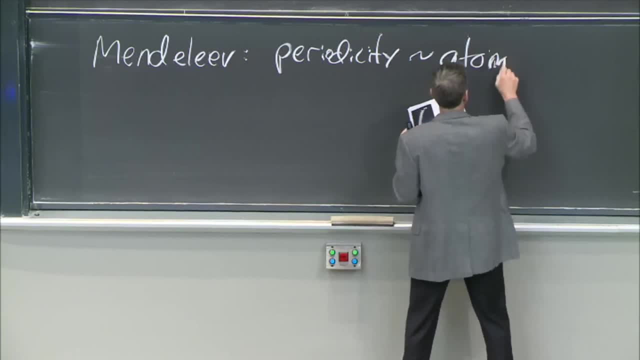 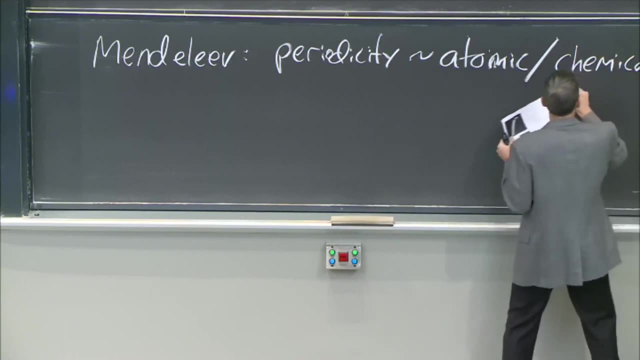 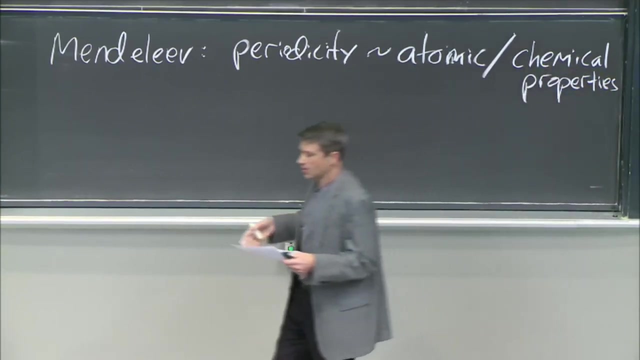 was related to both the atomic mass- and remember we talked about this- and the properties, the chemical properties, That chemical properties That allowed him to create An ordering of the elements. An ordering of the elements That is still the ordering, essentially, that we have today. 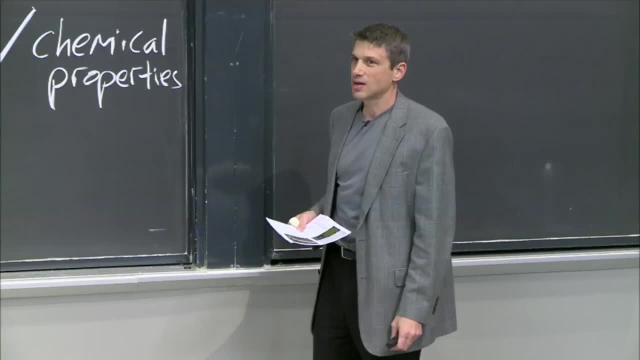 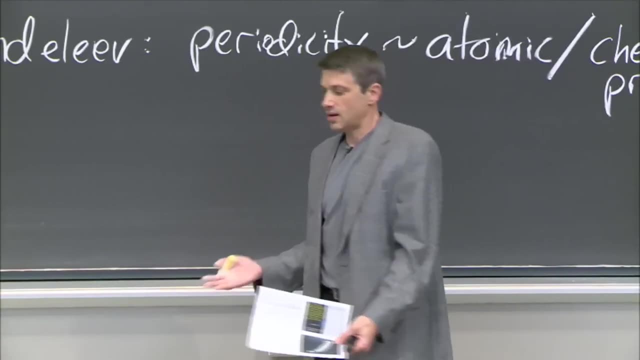 But the problem is, why did they have that ordering? I didn't really tell you why. sometimes he was like, well, the properties win, Yeah, Okay, Maybe the mass, No, no Properties win. Properties need to be aligned in this column. 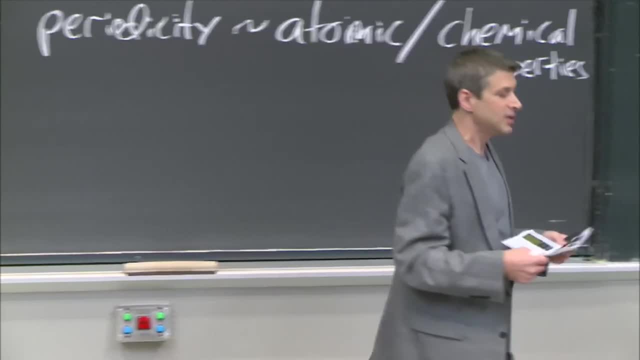 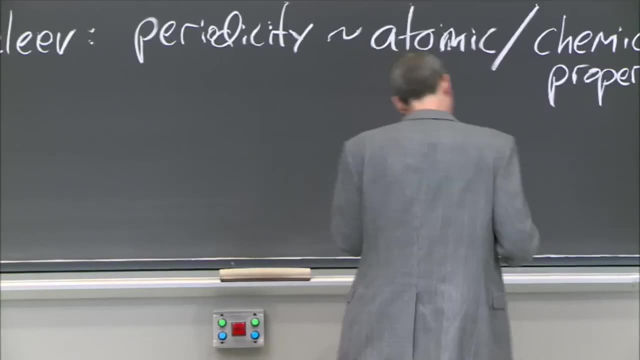 So I'm going to move those over. That's what he did, Right, But he didn't know why, Except that it made sense. It made sense to him. Moseley's experiments told us. They gave us the why. Oh, it was so important. 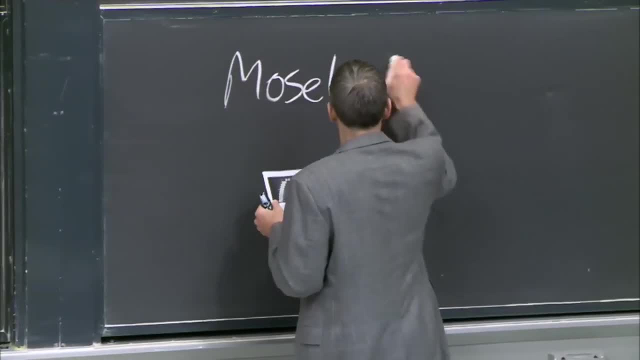 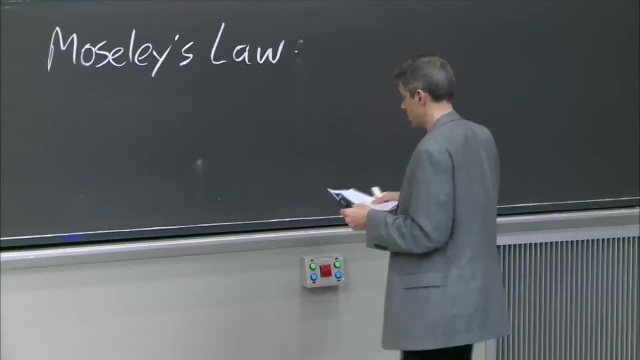 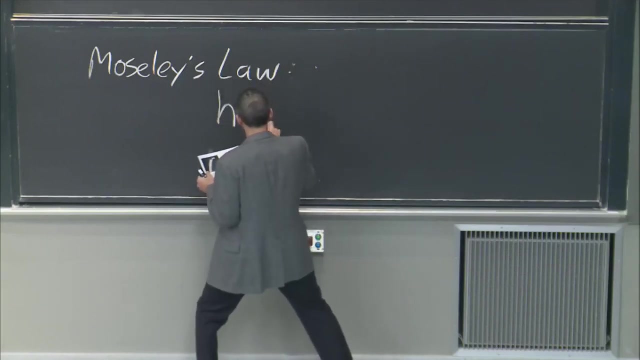 And Moseley's law. Moseley's law was essentially him thinking about the Bohr model for these x-rays, for these characteristic x-rays. So he said that h nu- so that's the frequency for some k, alpha line okay- is equal to 13.6. 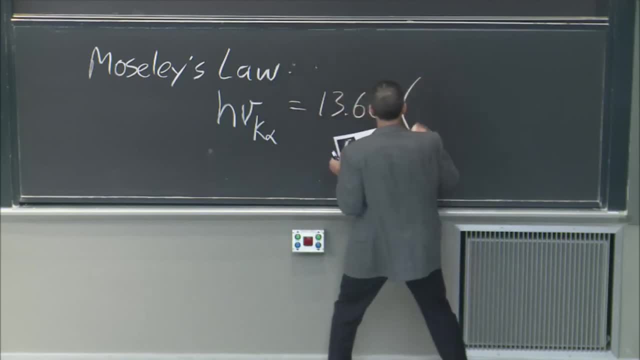 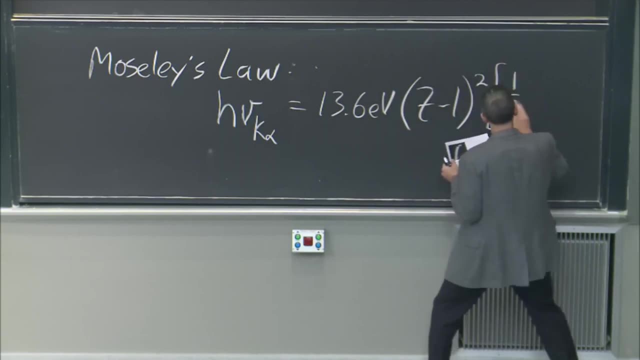 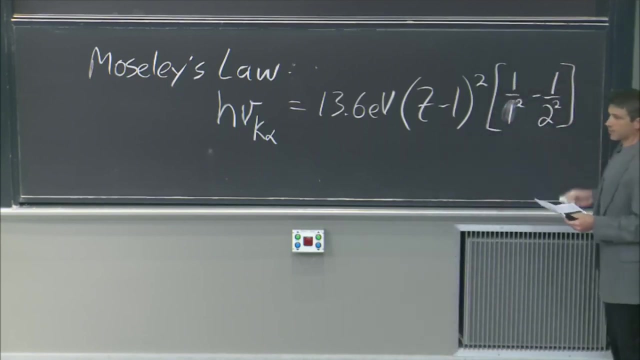 e, v- Oh, that looks familiar. Times z minus 1 squared, And then he did the difference in energies, Just like we've done now a number of times in this class. That's what he did, And this is 3 fourths. 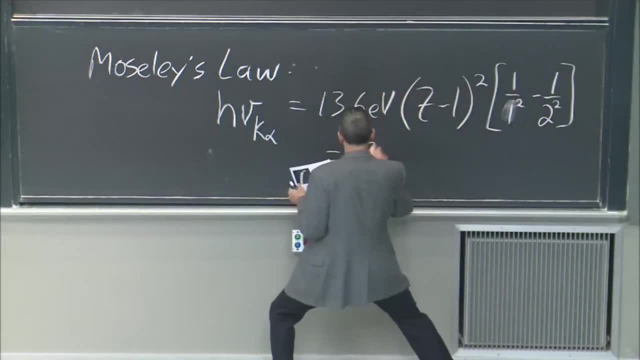 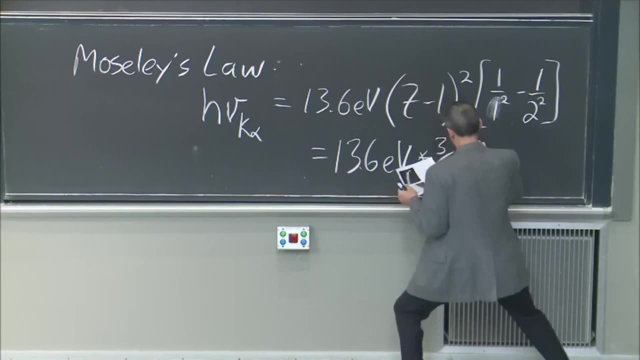 Why this? Well, let's talk about that in a second. So 13.6 e v times 3, fourths times z minus 1 squared. Okay, z minus one squared. Two things about this. right One is: why is it three? why is it? 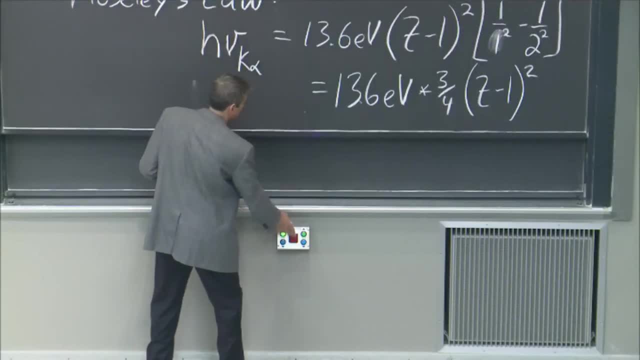 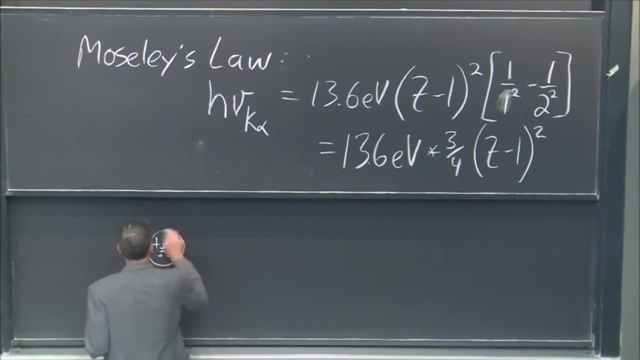 one over one squared, minus one over two squared. Well, that's because they knew, or at least they were pretty confident, that you had this, this positive charge in the middle. here, that's the, the protons in the nucleus, and then you had these electrons right. So you had 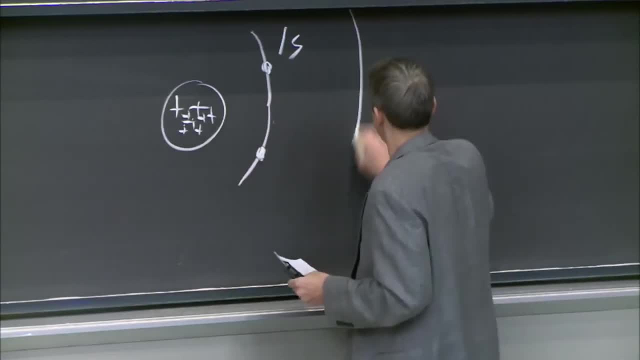 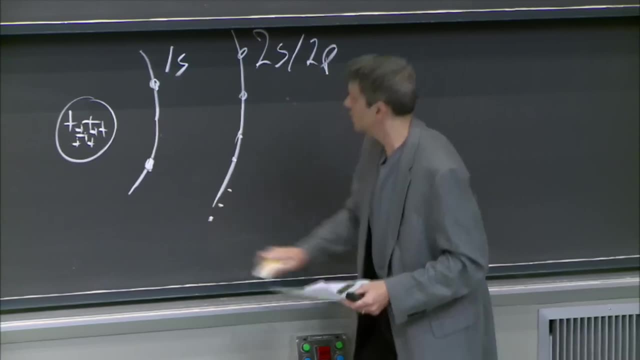 like the two, the 1s electrons, and then you had another shell out here, okay, And so they knew: okay, 2s, maybe that's combined with 2p, so it goes on. So what happens in the x-ray experiment? 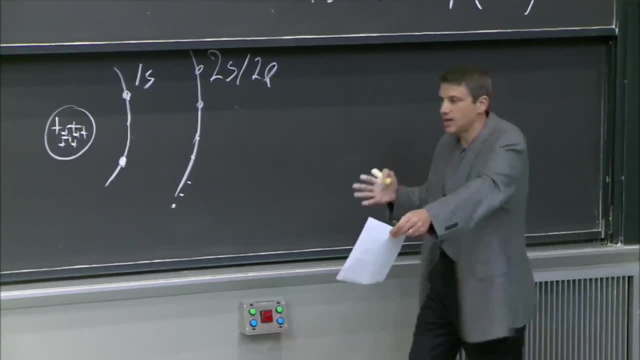 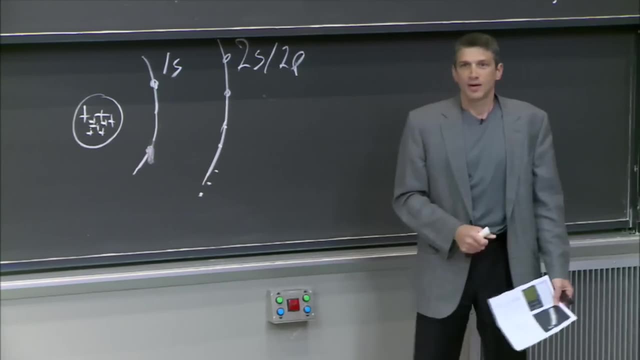 Well, what happens is you shoot an electron in. Ren can just crank the voltage up so high that an electron could come and knock that out. Right, And so this, that's what did it, And so now one of these can cascade down there. 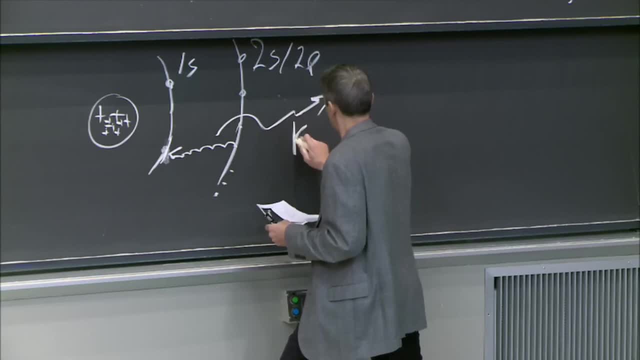 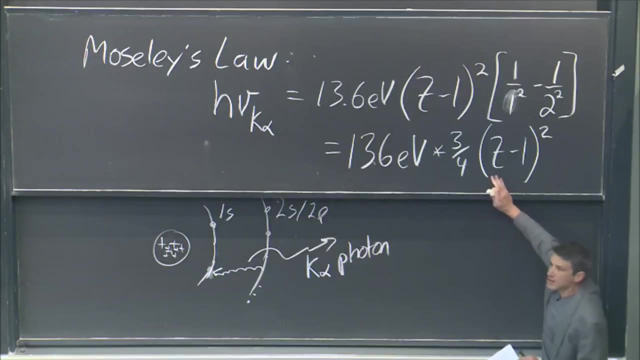 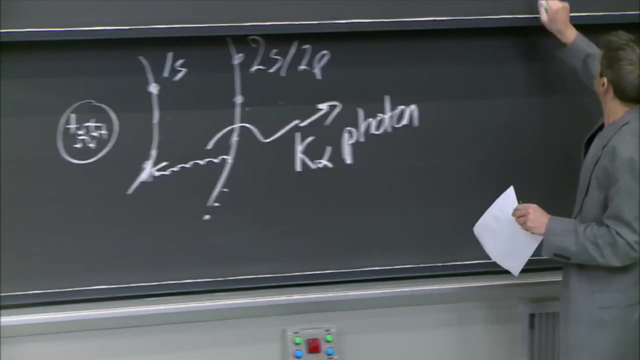 and give off a k alpha photon. right, This is. this is nothing new, We've talked about this, But you see it here in the equation. You see it in two ways. First, we're going from 2 to 1.. One squared minus one half squared. 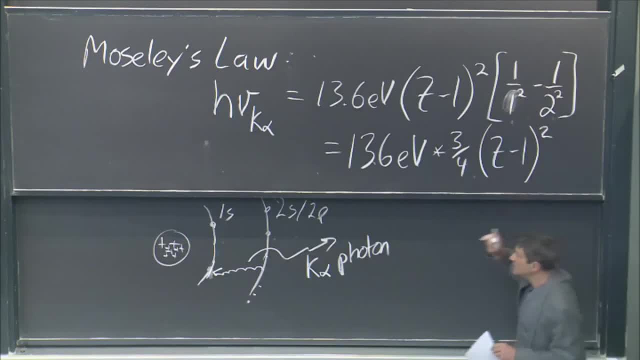 Three fourths Right, But second- and this was critical- the z minus one. The Z minus one told us that. And all these positive charges in here, all these positive charges are screened perfectly by one electron, this one that was left. 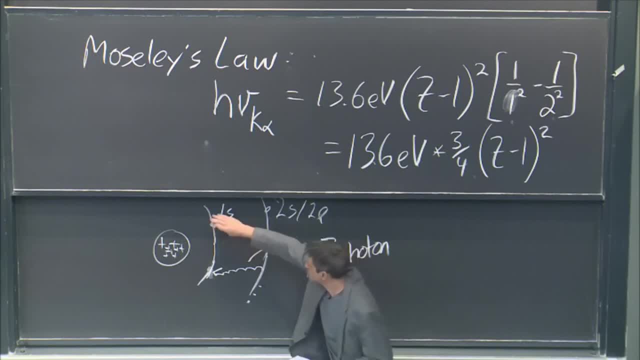 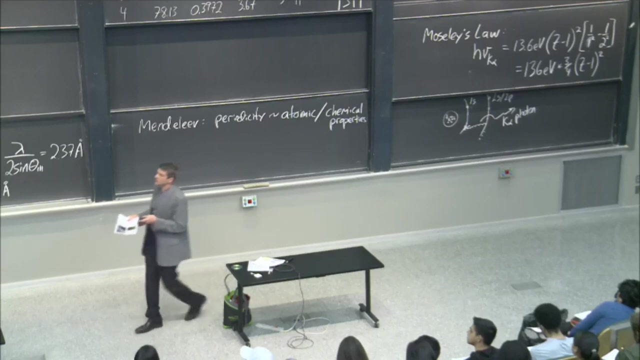 And it works. He assumed perfect screen. So what do all these see? They see z minus 1.. They see z minus 1 if z is related to the atomic number. Now here's where this was so powerful, Because when you plot and you can't read this, 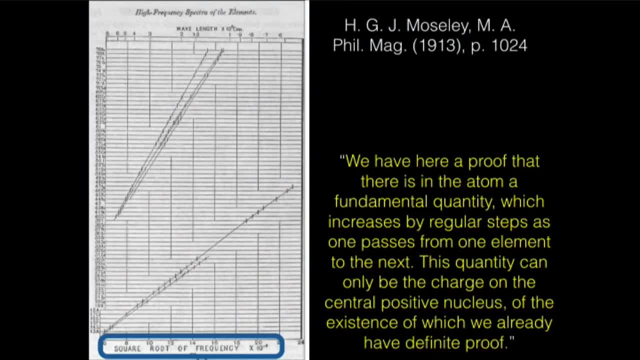 Don't worry about that. I just want to show you that it is a perfectly straight line. When you plot the k alpha transitions, these are different elements, These are his different elements. And if you plot the square root of the frequency, if you plot the square root of the frequency versus element, 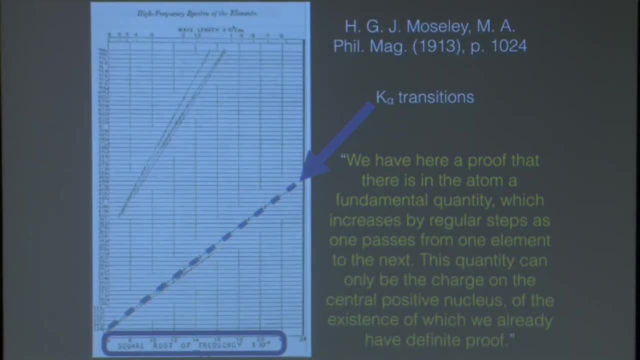 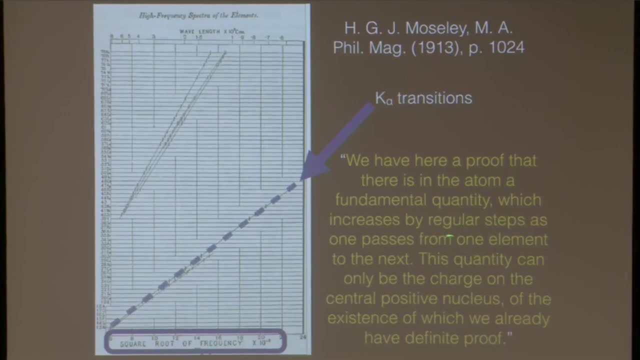 it is a perfect line That holds. And so what Moseley wrote in the paper is: we have here a proof- In 1913, that there is in the atom a fundamental quantity, a fundamental quantity which increases by regular steps as one passes from one element to the next. 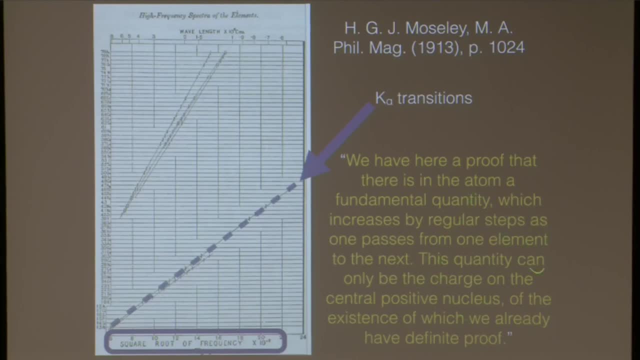 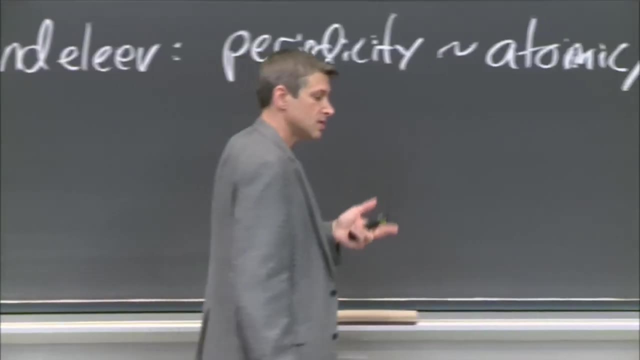 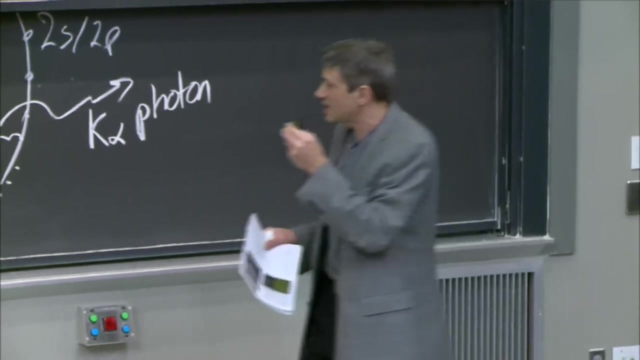 This quantity can only be only be the charge on the central positive nucleus, of the existence of which we already have definite proof. Now we know about that. We know from experiments that Rutherford did that that nucleus had the positive charge, But they didn't know that it was connected to the position. 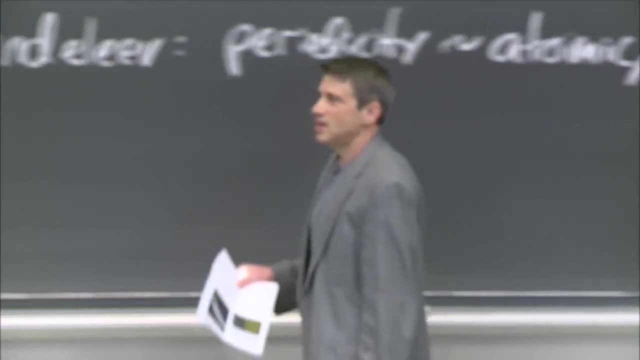 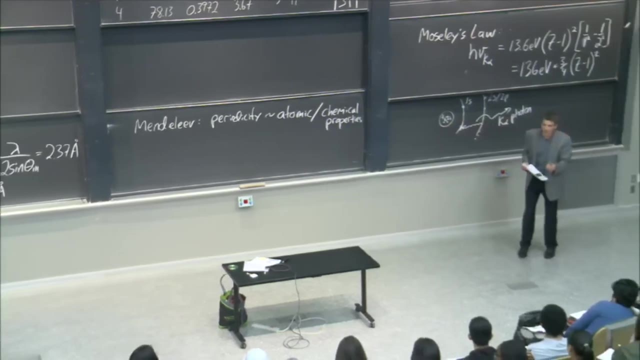 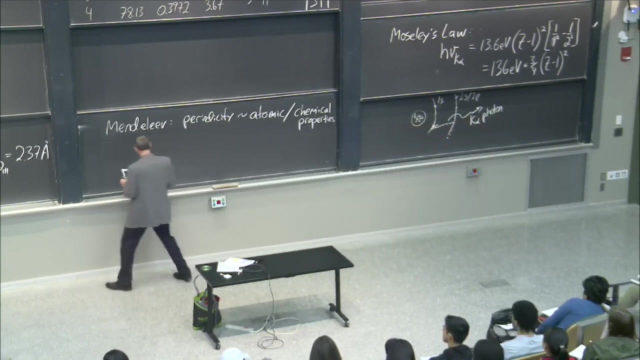 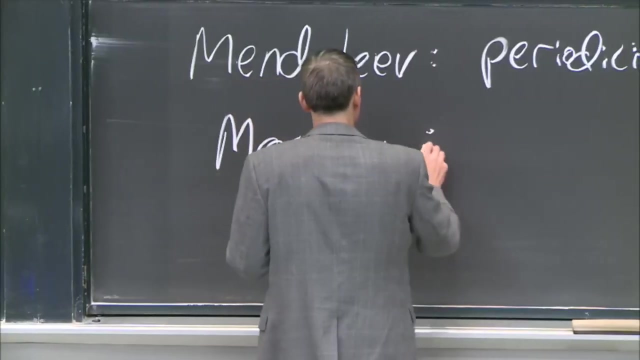 in the periodic table. In fact, years later people talking about those experiments at the time said people didn't even take Rutherford's experiments as seriously until Moseley's work came along. 44 years had come since Mendeleev, but Moseley gave it the foundation that it needed. 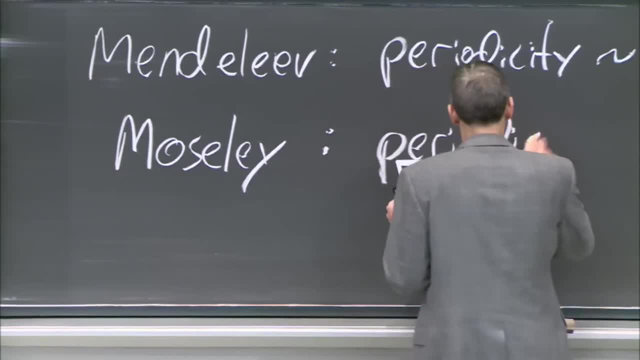 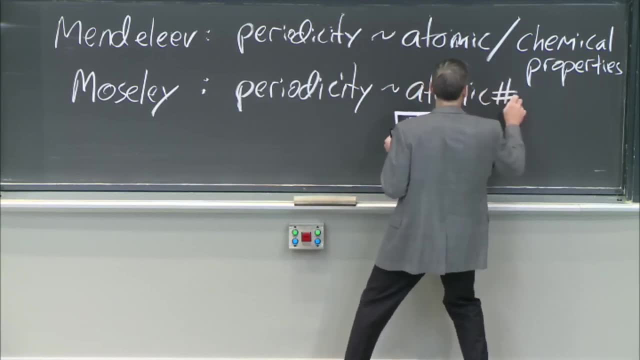 Periodicity is because of atomic number. Periodicity, Periodicity is atomic number. That was not known. That z gives you the periodicity And that gives you also the number of protons. This was a time when they didn't know what was going on. 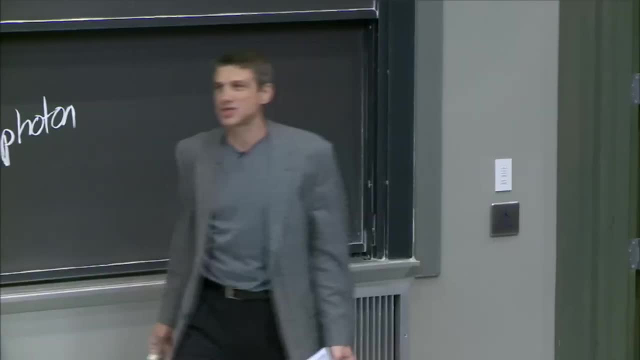 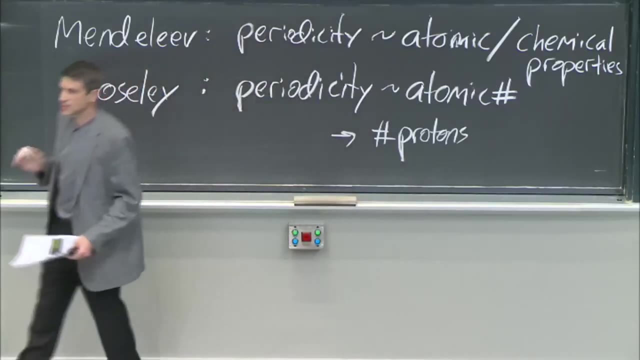 Why did the mass change so much? The neutron wasn't discovered until 1932, 20 years later, But this gave the grounding that was needed to the chemistry of the periodic table. It was a very important discovery, Very, very important discovery. 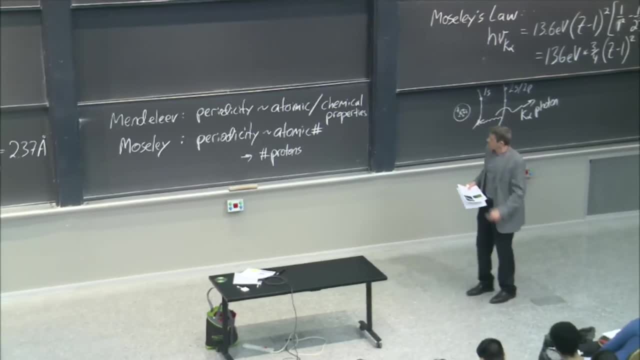 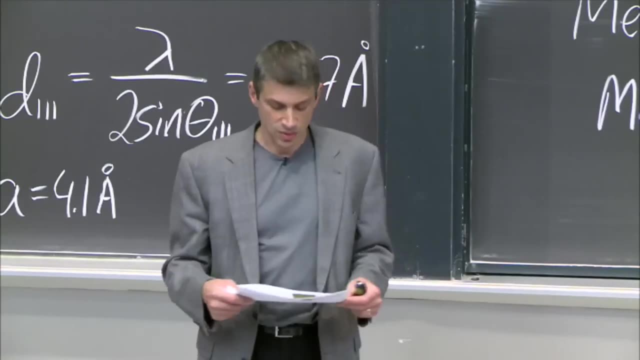 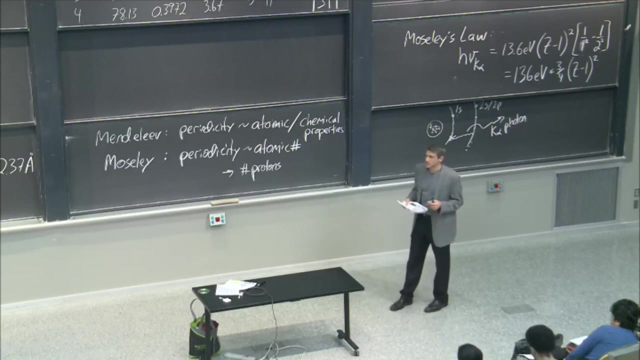 So that's my why this matters, And it's really tragic because he died tragically in World War I at age 27.. And the Nobel Prize was not given in 1916 for either physics or chemistry. He died in 1915.. 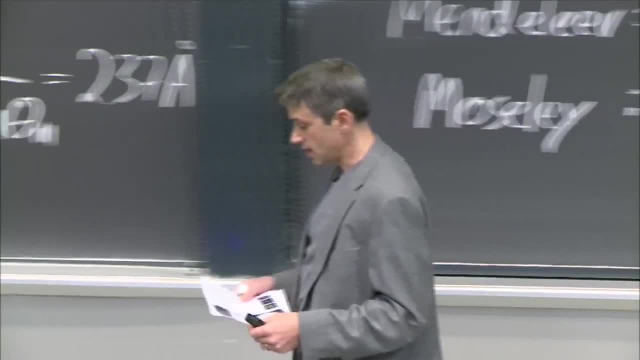 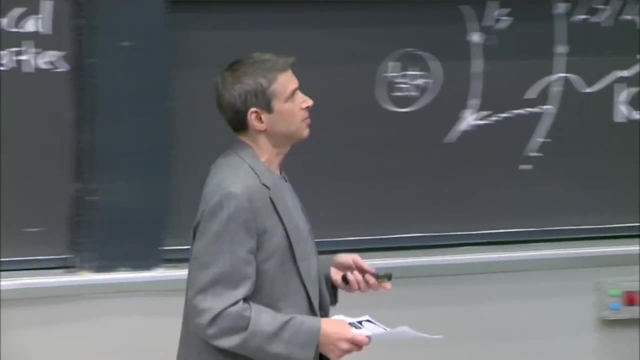 And most people at the time believed that he would have won it at age 28.. That's how important that discovery was. OK, Let's go back to brass. I got to go to brass. What's going on here? What is going on with brass? 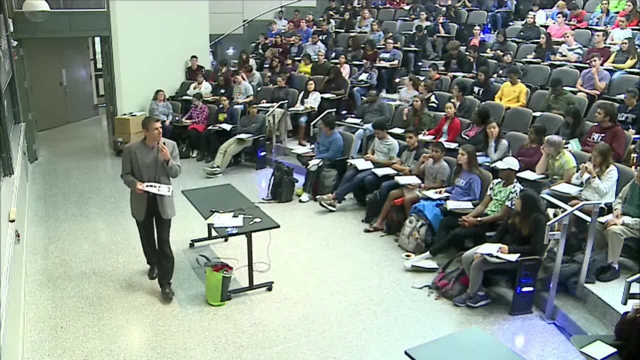 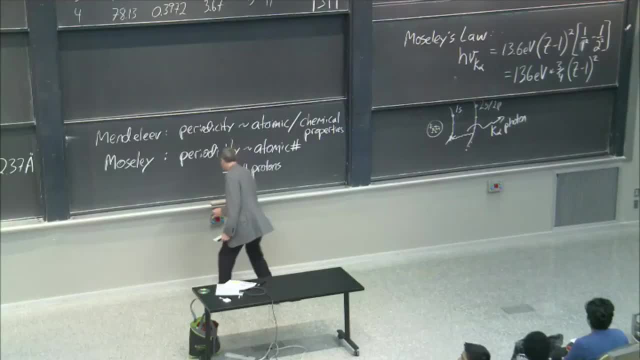 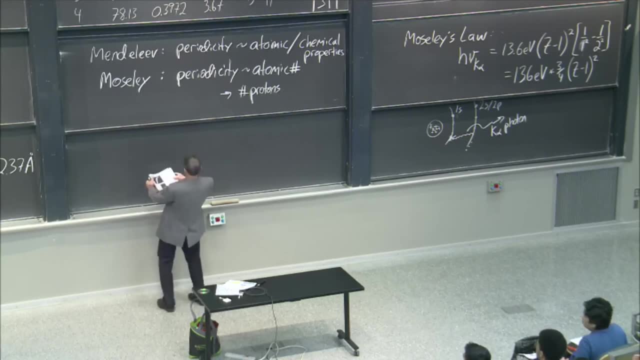 Any ideas? Why didn't he just put zinc there? It looked so good until brass. What is going on? Well, here I'll give you a hint. OK, The melting temperature. let's see Brass. OK, Zinc melts. 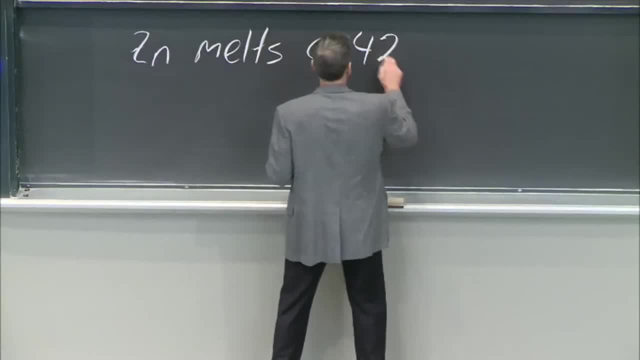 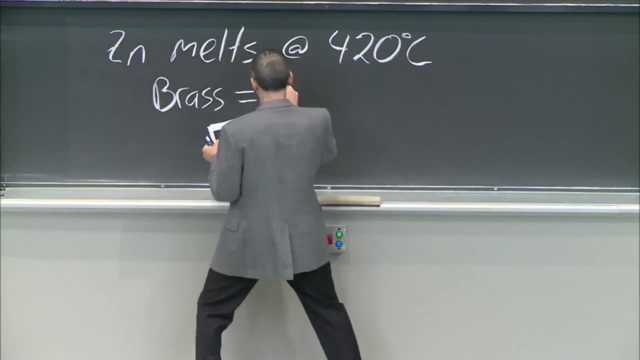 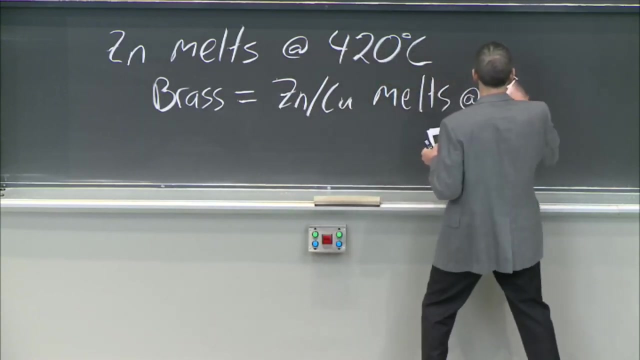 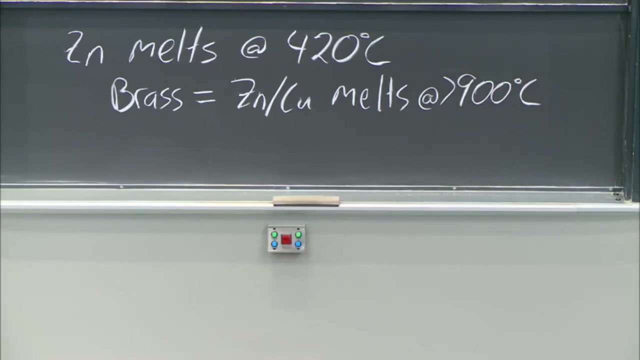 Around 420 C. Brass, which equals zinc and copper, melts at around 900 C or more Greater than 900 C. That's a hint, Because if we go back to the video, let's go back. Oh, the sound is on. 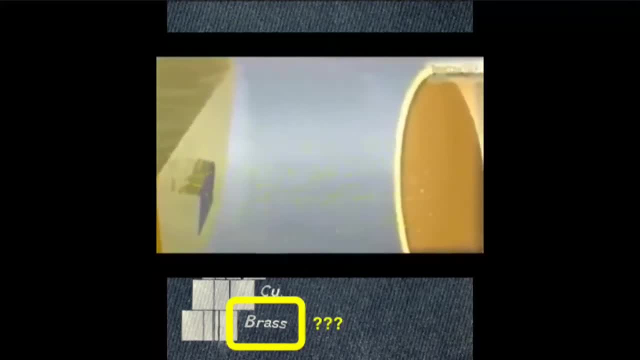 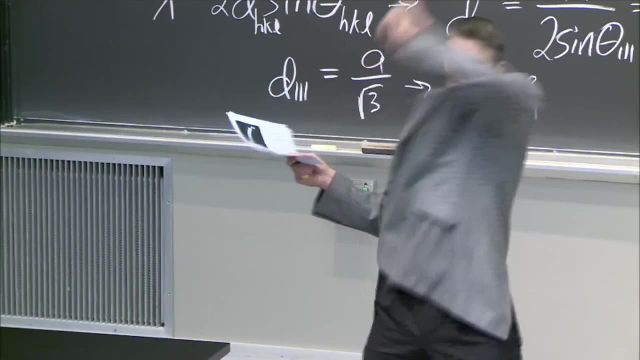 How does the shape? Those are the electrons, A small portion of the target. Let me set that up. The electrons are because I'm doing it in the middle. The electrons are coming off of cathode because Rankin has cranked the voltage way up. 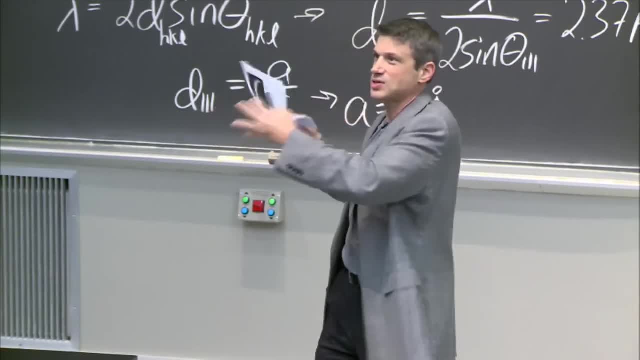 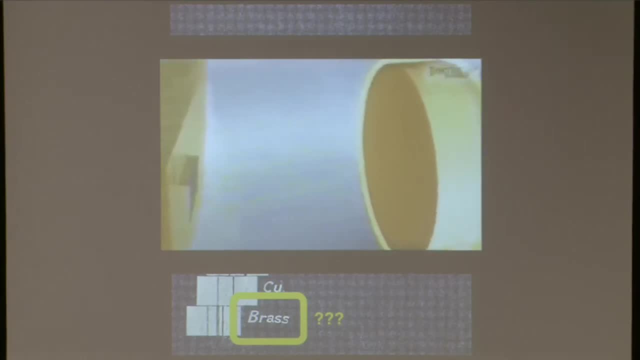 and pumped all the air out. So those electrons are coming off with thousands and thousands of KeV. OK, They're coming out, And that's what's on the right here. There they are. The cathode is shaped to focus the electrons. 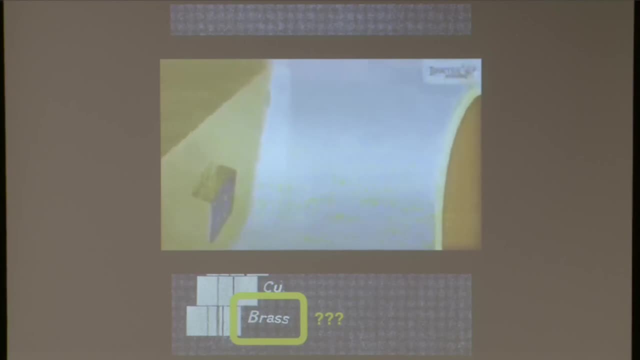 onto a small portion of the target, which increases the intensity of the X-rays produced. The target is typically a piece of glass- It's tungsten or molybdenum, which may be embedded in a stationary water or oil-cooled rod. 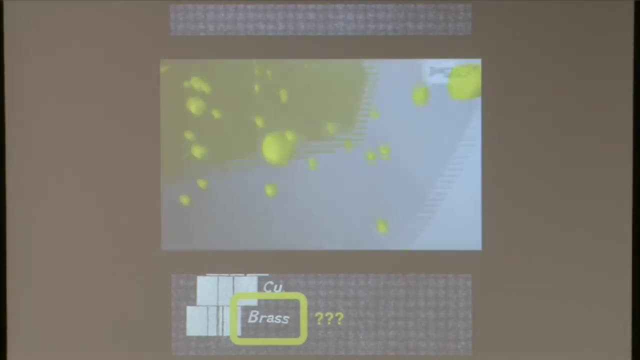 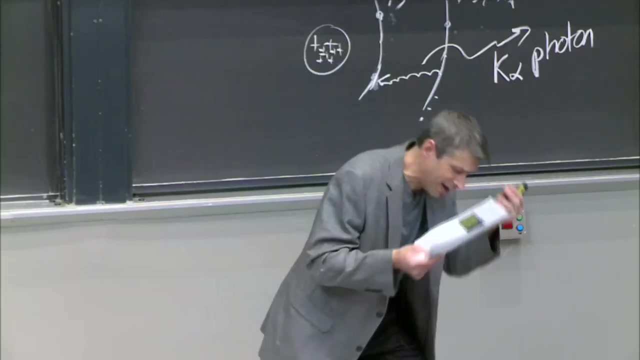 or on a rotating disk. The high-speed electrons collide with the target and rapidly lose energy. There are two X-ray producing interactions between the incident electrons and the atom. Oh, look at the power. You can feel the power coming into that tiny little piece. 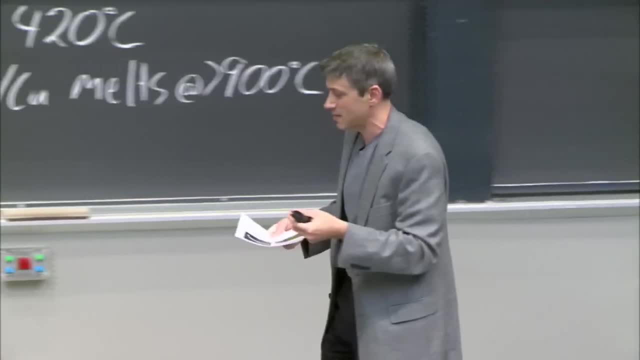 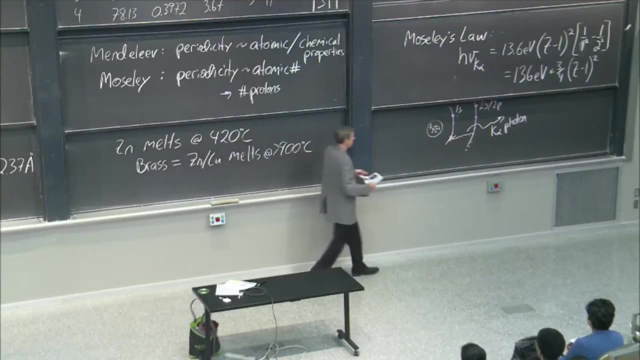 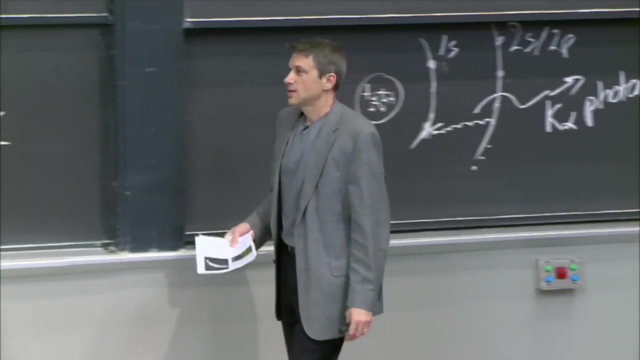 of metal. Now, some of the time you get the transition. You get the transition that we talked about. You knock an electron out and you emit a photon, a K-alpha photon or maybe an L-beta photon, right, And sometimes you slow the electron down. 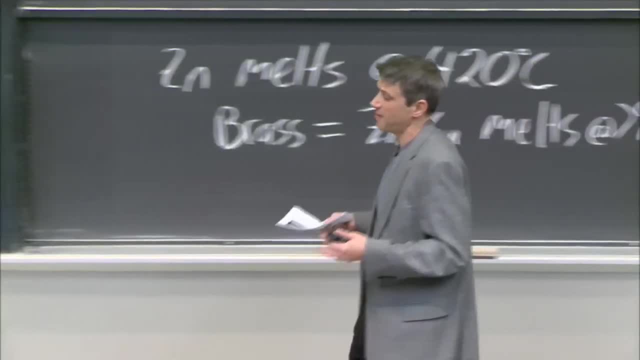 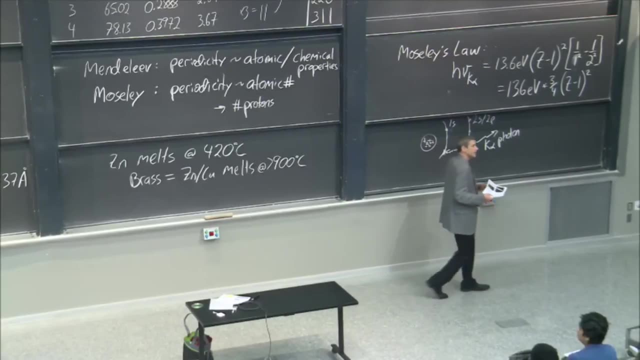 so you get the Bremsstrahlung? Yeah, but there's so much energy being pumped into this material And a lot of times those electrons just collide and heat up the metal. That metal is getting extremely hot And in these experiments, either you. 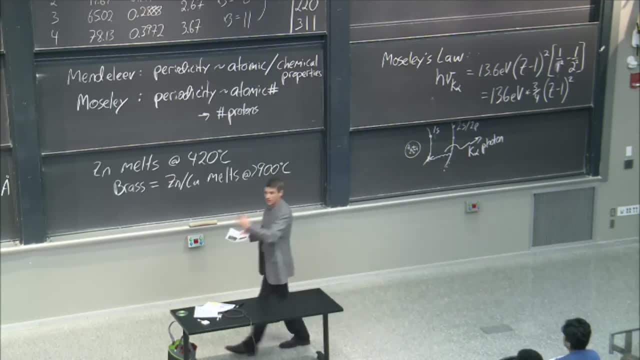 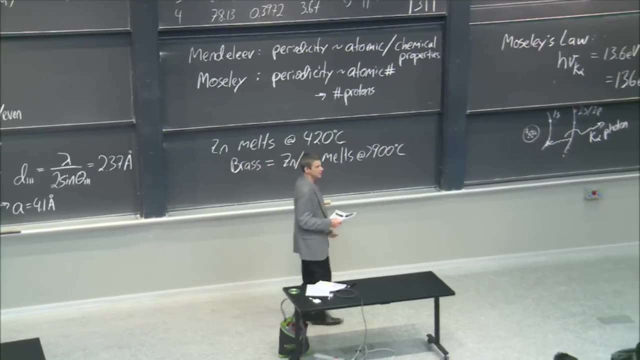 cooled it. or you might rotate it quickly, right, so that it gets to cool down, It gets a little break, right? Or you do both, Or you just throw up your hands and you say: you know what? I'm just going to go for an alloy that's. 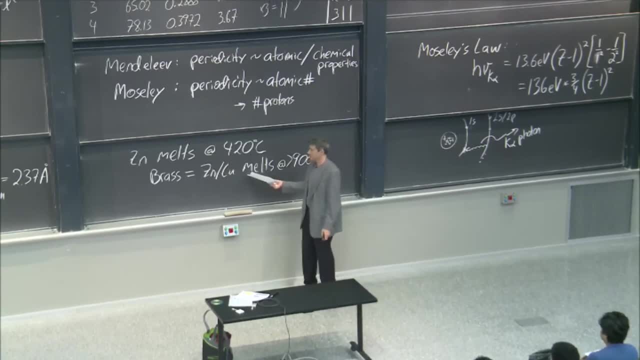 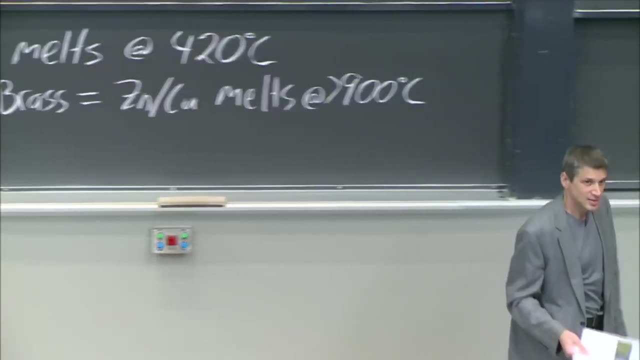 got some zinc in it but won't melt every time. Yeah, that was a good idea. So you put brass in. OK, you're going to get the copper lines, but you'll get the zinc lines. You'll get the zinc lines, right. 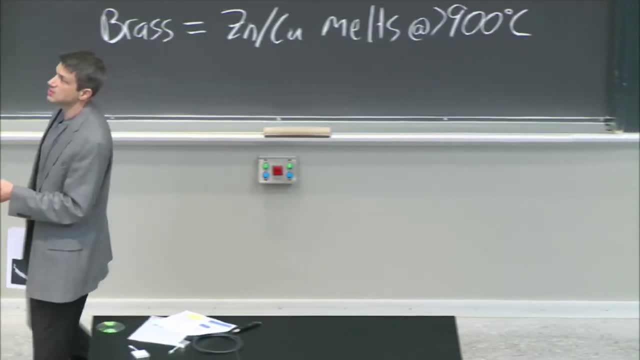 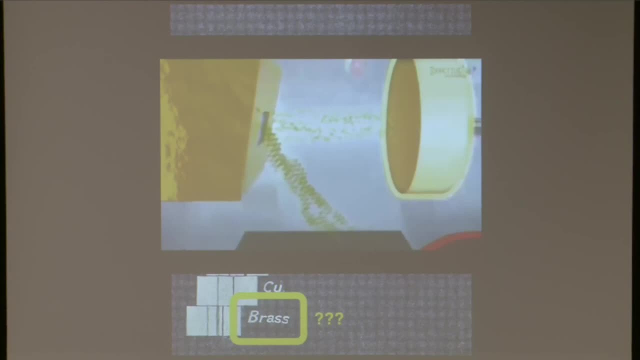 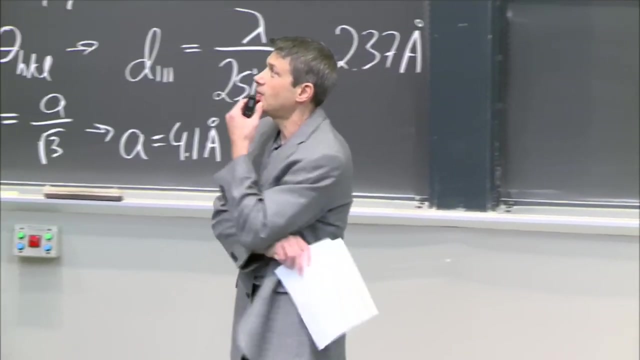 And that was why he used brass And that's why you can see you get extra lines in the case of brass. All right, OK, good, All right now. I'm very excited about Moseley. It allowed us to actually understand this. 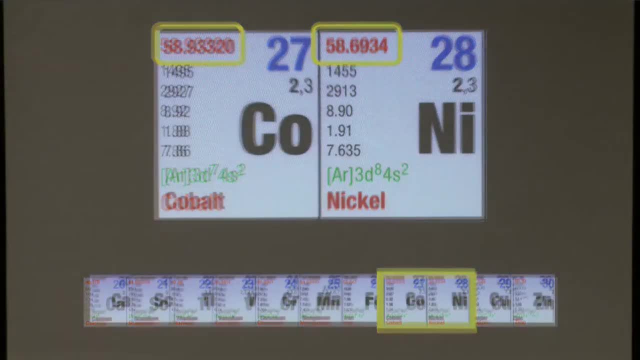 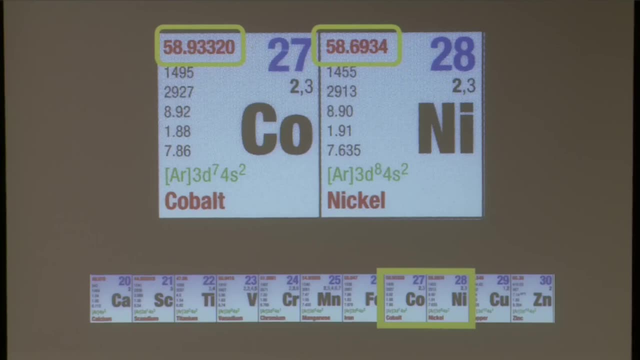 not just because- Look at this- Mendeleev was like you know what? Cobalt and nickel can't be swapped. Hey, all you people who just think about mass, you're not going to put them in the order you think. 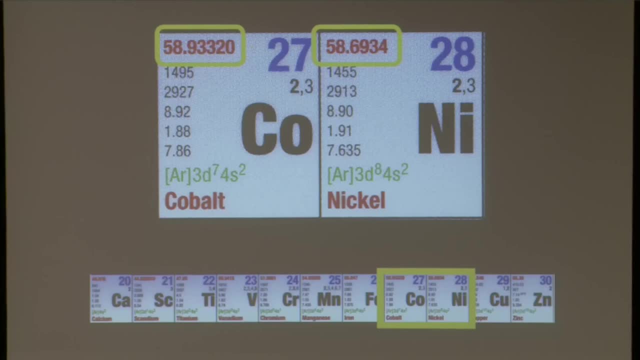 I'm changing that right. I'm changing it because properties matter. Moseley said no. you're changing it because it's the right order, because of the blue numbers. You're changing it because there is an actual count here that matters. 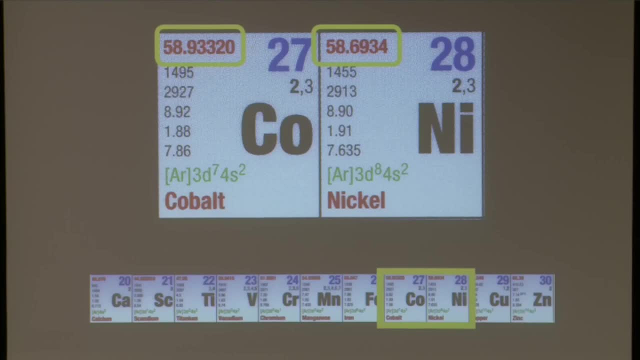 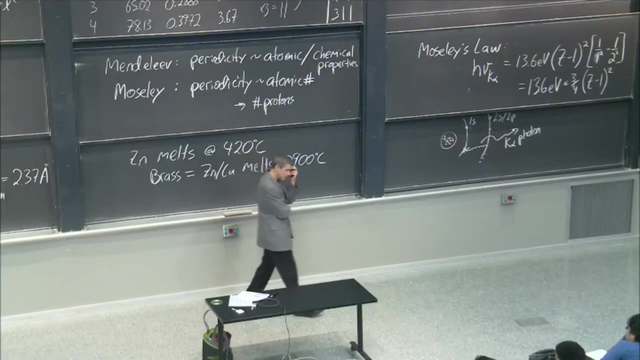 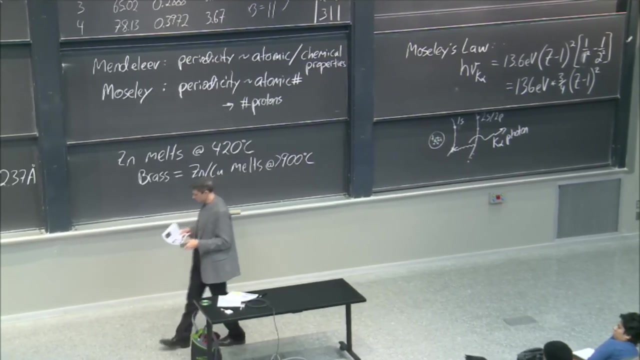 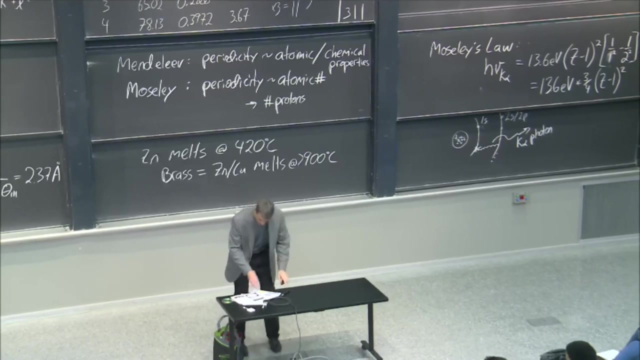 And that is why your periodic table is what it is: Absolutely critical. It put the lanthanides in the right place, It allowed the prediction of elements you know, like how to do it, like not to be a- And it set it all on this much more solid grounding. 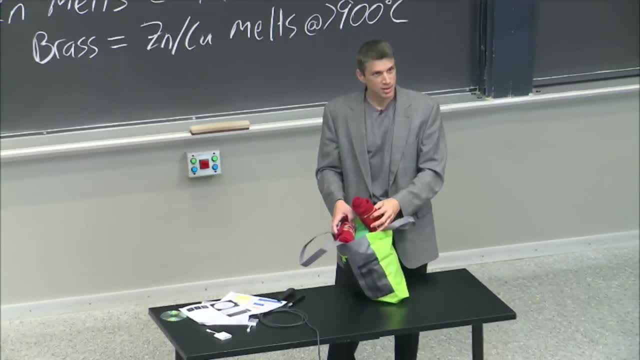 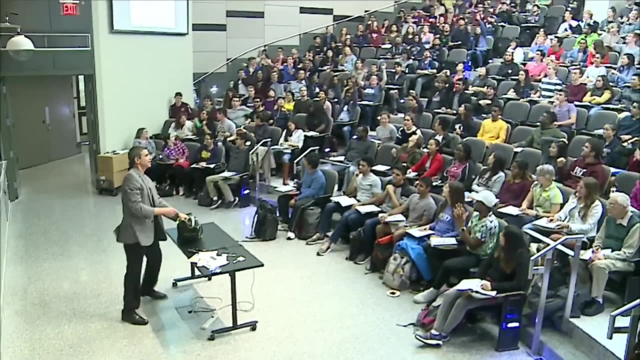 So that is the contribution of Moseley. I can't help it. I got to. I'm very excited, So I brought T-shirts. I knew I was talking about Moseley. Now I'm going. OK, All right there. 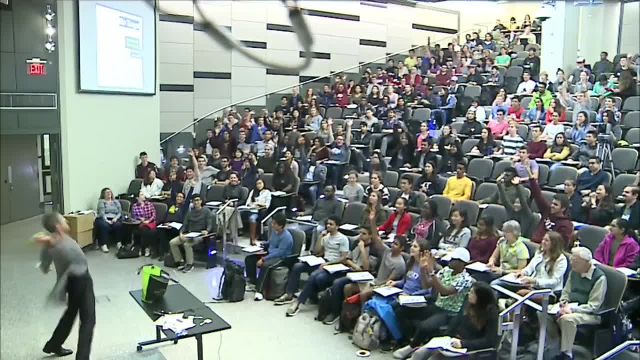 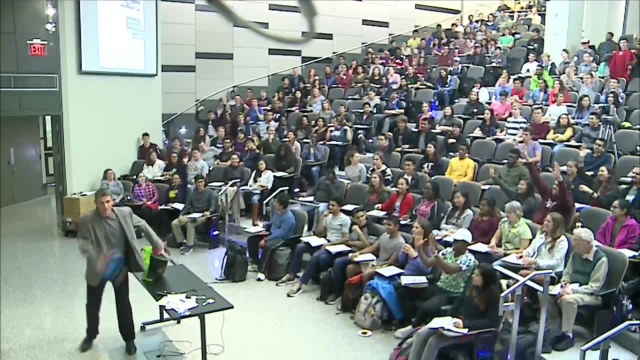 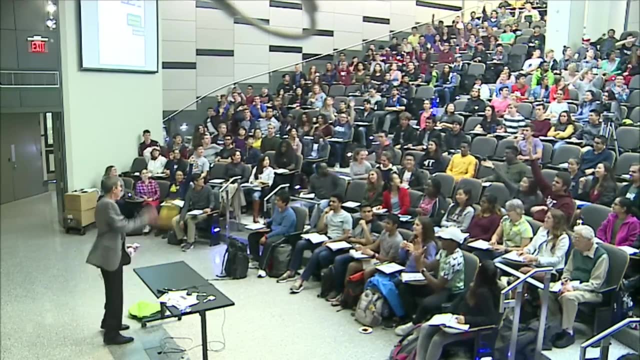 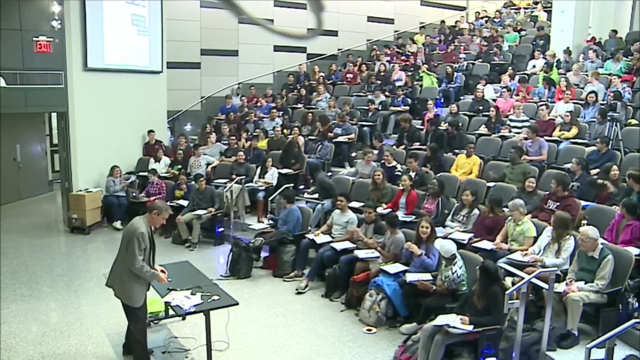 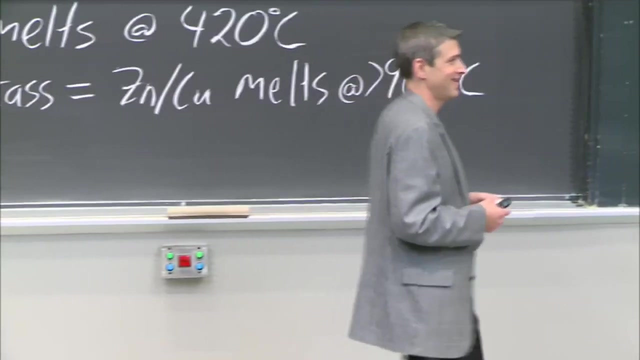 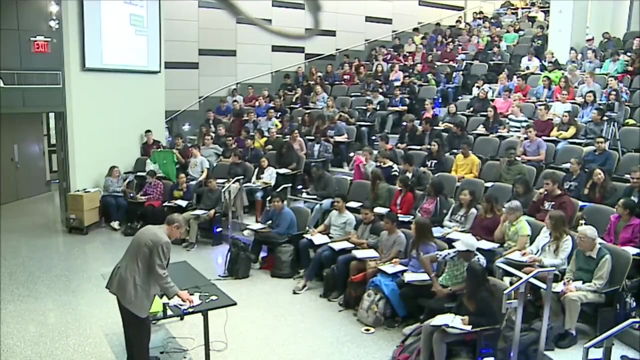 And oh, that's a bad arm- And up there And hold on, Hold on now. Okay, there, There, And this is all for Mosley. This is all for Mosley, All right Now. okay, Now, apart from me showing off, I don't have much of an arm. 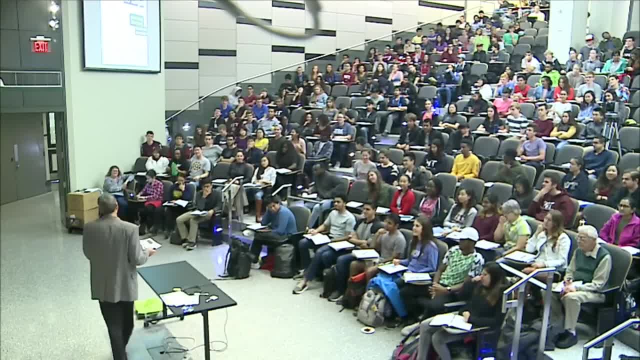 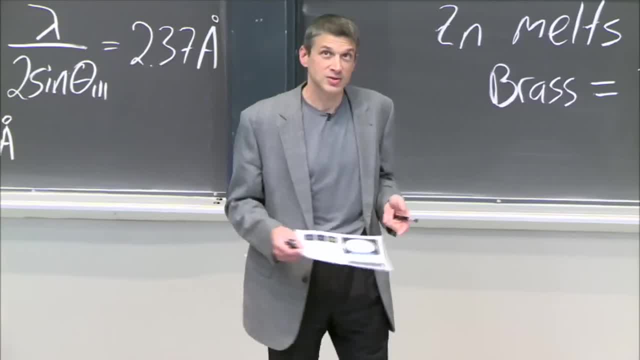 one thing I'd like to say is: if you did already get a T-shirt, please just hand it off to a friend or somebody You know let's share. Sharing is always caring. Now there's another type of x-ray I want to talk about. 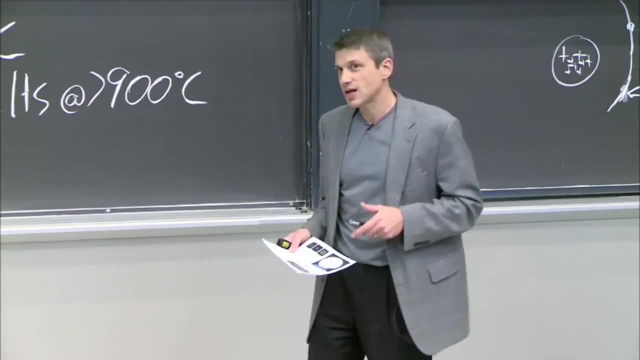 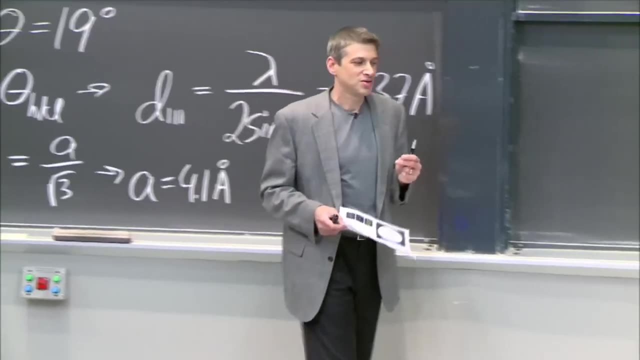 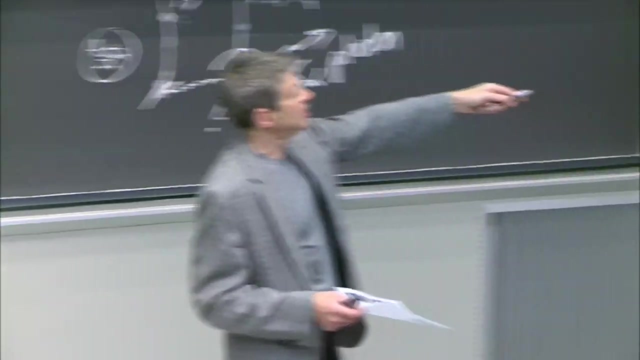 And actually this is much less used today. I hope you've gotten a sense of how powerful these characteristic x-rays are. You know exactly what the wavelength is, But in the very earliest XRD experiments it was the Bremsstrahlung radiation that was used. 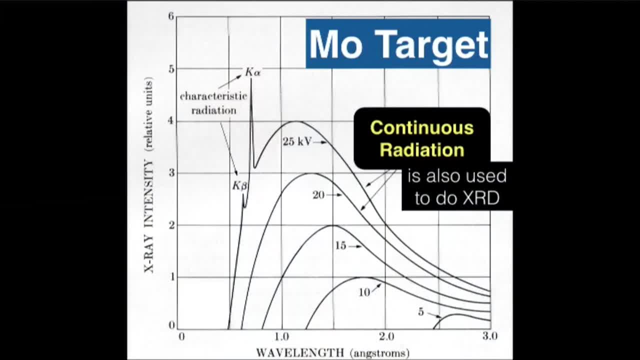 And that was by Von Laue, So I want to just tell you about that. And so here's an example of an MO target. Now, let's remind ourselves what we're looking at. These are x-rays. These are x-rays. 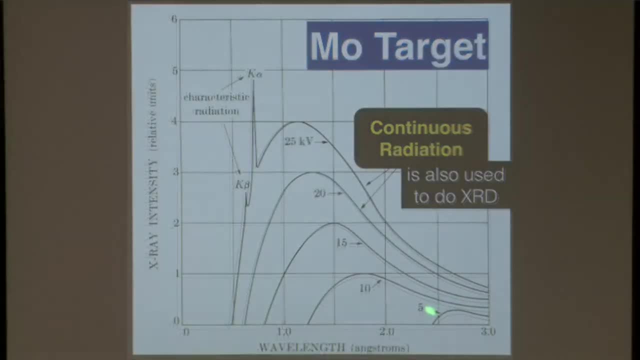 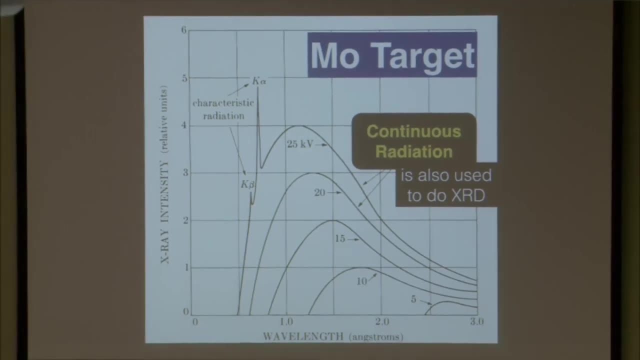 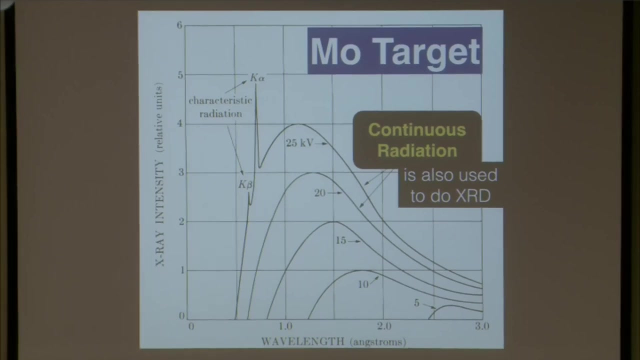 These are x-ray intensities versus wavelength And this corresponds this: 5, 10,, 15,, 20, that corresponds to the kiloelectron volts, That's the thousands of electron volts of the incoming electron, That electron that came in here and knocked this out from the cathode. 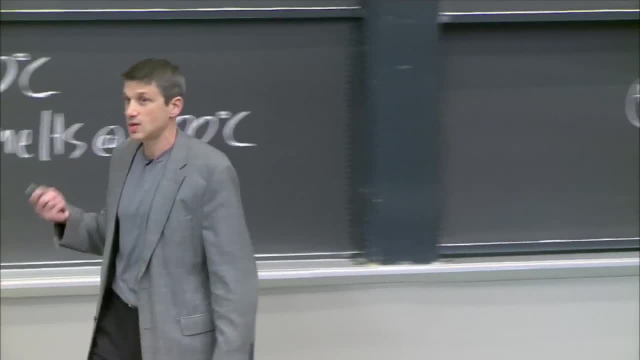 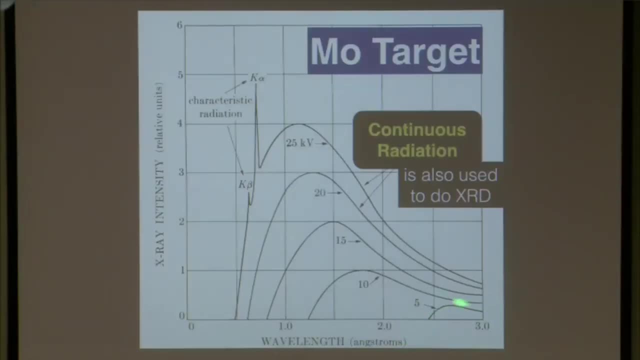 Right. Okay, Now that electron: if it comes in- and we talked about this already, but let me remind you- if it comes in at a kind of low energy, well, you're still going to get this continuous spectrum, This continuous spectrum. 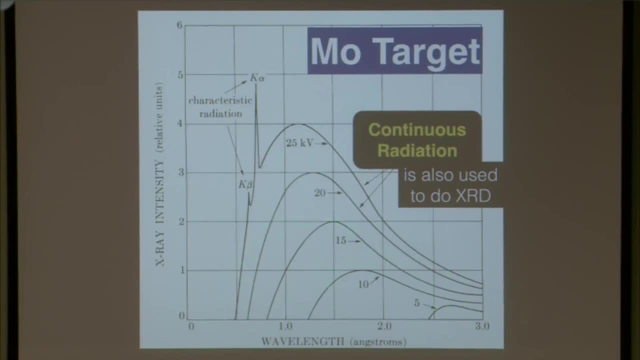 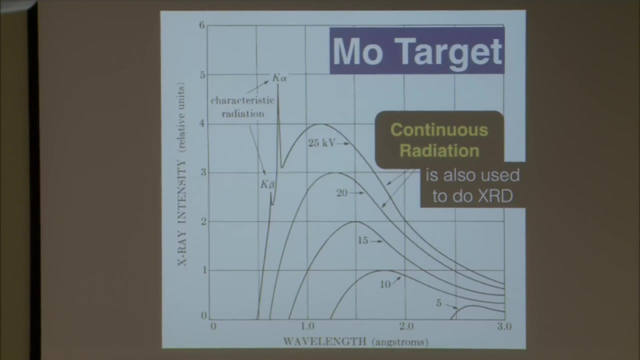 Why does it look like that, Beyond the scope of what we need to know? but, in case you're wondering, it has to do with very complicated effects that happen when things- when x-rays- come off and then are reabsorbed, Right. 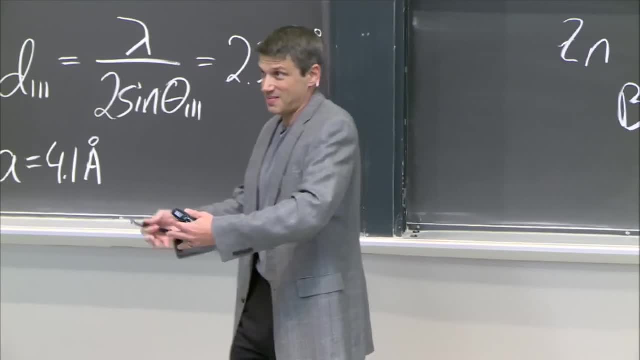 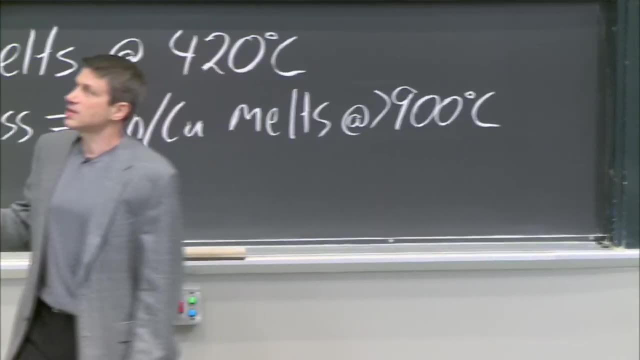 By the same material. You can imagine that that could lead to all sorts of interesting cascades of absorption and emission. That's what leads to the shape, But we don't need to know those details. What we need to know is that, as you increase the power of those instants, 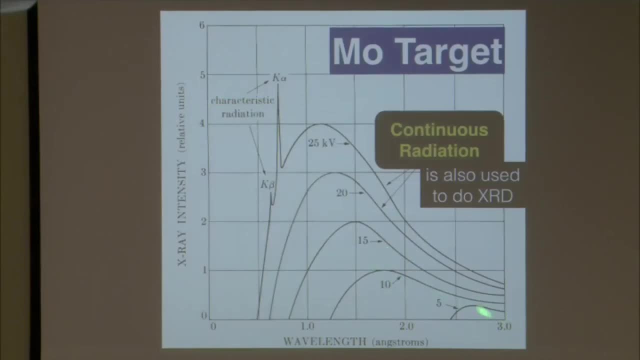 as you increase the power of those instants, of those incident electrons, you're going to get more and more intensity of x-rays And this goes down. This wavelength, the minimum wavelength or maximum energy of the continuous spectrum, the maximum energy, goes up. 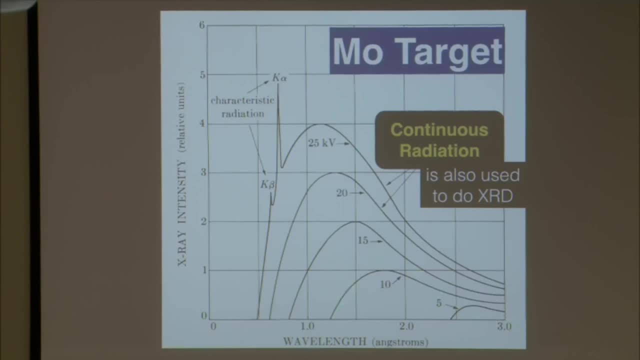 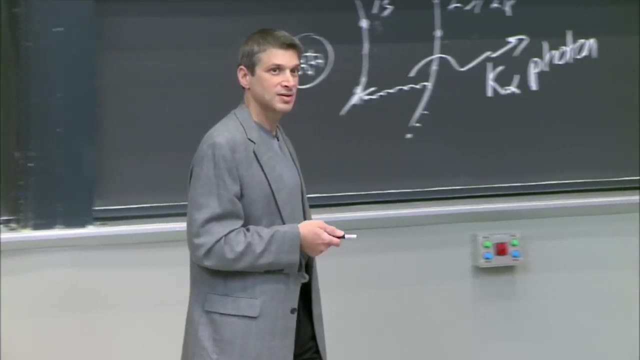 Because the maximum energy you can get in the continuous spectrum is equal to the incident electron itself. So it's set Right. Remember the Dwayne something limit Dwayne Hunt. Okay, We talked about that already. How to get that value? 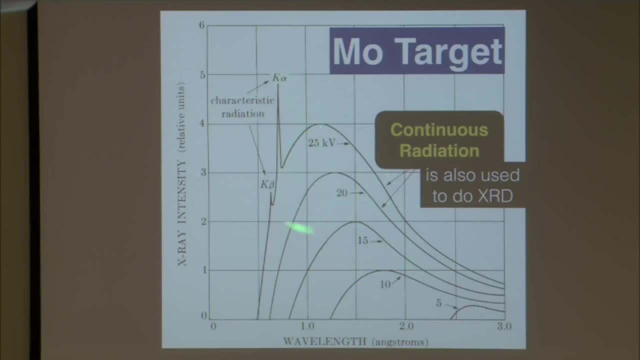 Yeah. but then you get to this certain point and look, all of a sudden the characteristic lines appear Right And those are the K-alpha lines from molybdenum. Why all of a sudden? Well, because you got over the amount of energy needed. 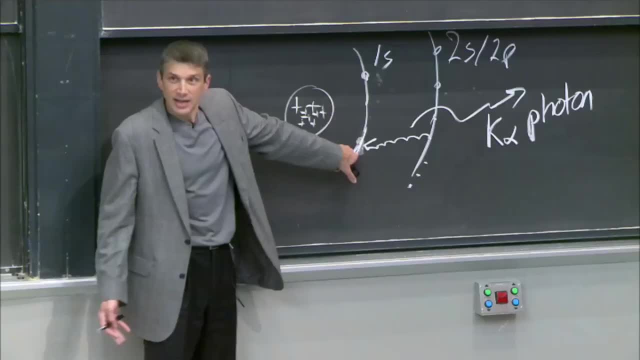 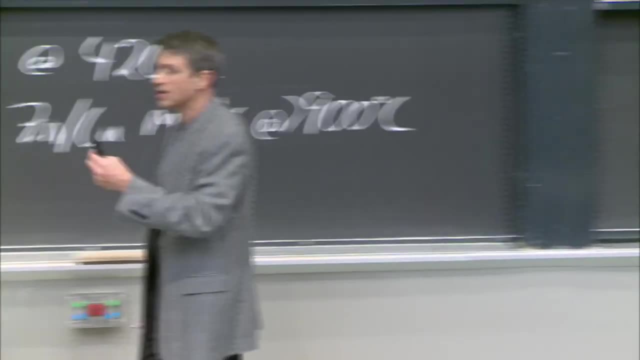 to kick out a 1s electron from molybdenum. That's exactly why, Before that, you had enough energy to produce x-rays, but not enough to kick out the 1s electron. It's kicking out the 1s electron that gives you characteristic peaks. 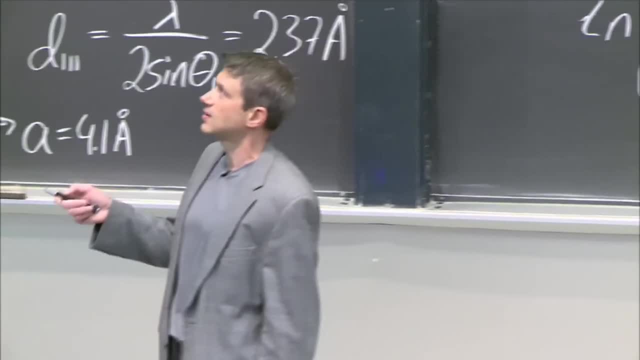 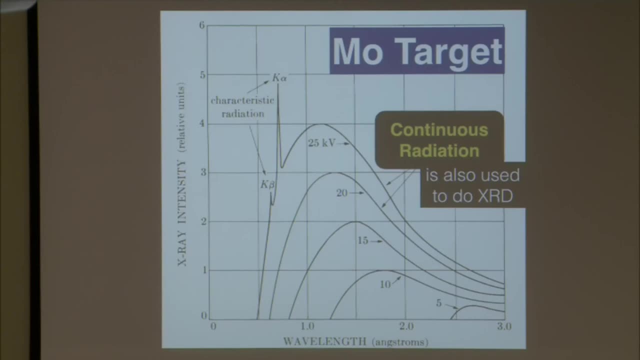 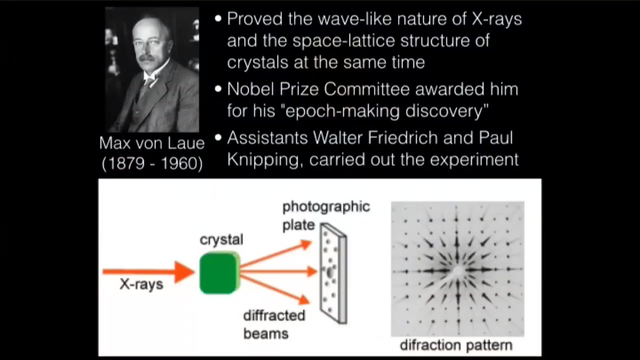 Okay, good, This is all reminder stuff, but I want to get back on that page. But see now, okay, this continuous part is also used, And it was used, like I said, by von Laue, And von Laue was again a really, really smart cookie. 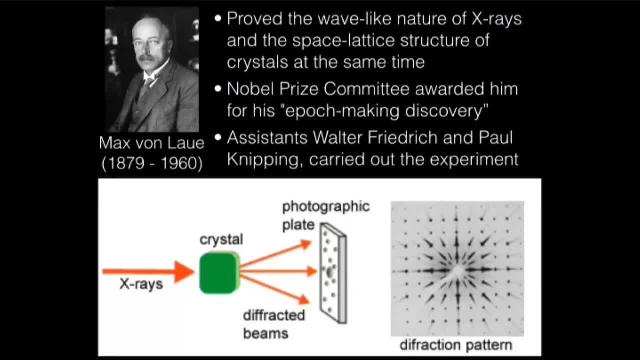 And he used the Bragg condition- okay- to prove that the x-rays and the space lattice structure of crystals can be interfered with each other to make this diffraction. But what he did was different. Okay, so the Nobel Prize was given for this epoch-making discovery. 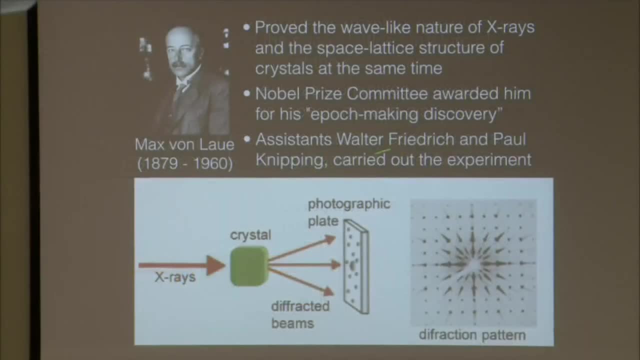 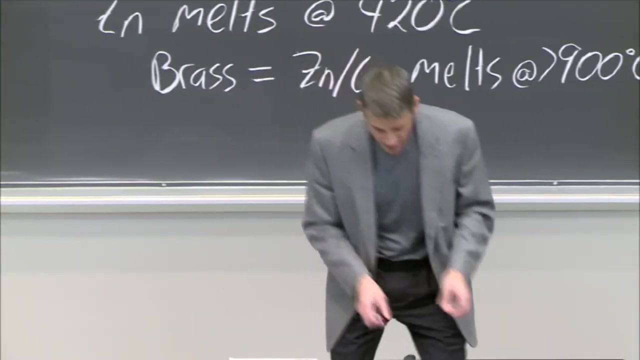 And I'm actually very happy that the people that worked with him also shared the Nobel Prize right, Walter and Paul. What they did was different, though: They took this continuous spectrum and instead of having so, instead of fixing the angle and the lambda- 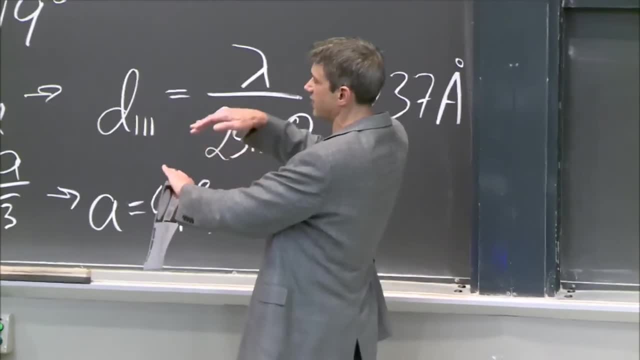 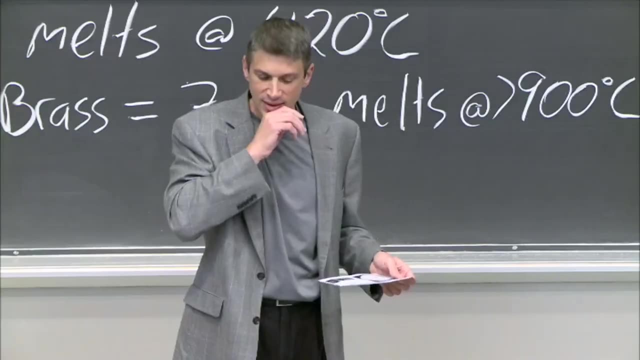 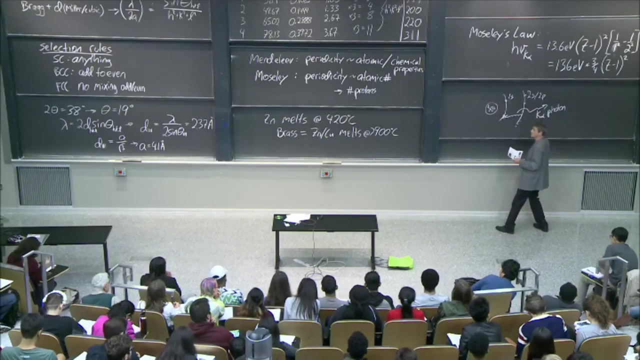 I'm sorry, instead of varying the angle, but having a fixed lambda, they did the opposite, Because the continuous spectrum has all lambdas, right, And so you can imagine how this works, right, You can imagine how this works So in the Laue version of XRD. 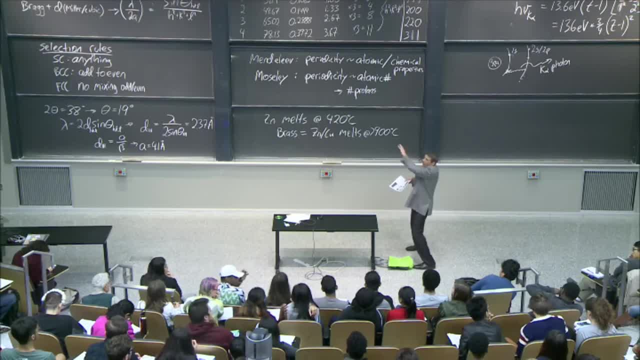 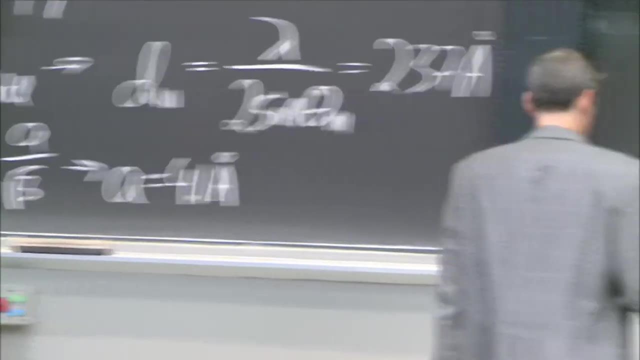 you shoot the x-rays, which have all the wavelengths in them, at a crystal. that's fixed. I'm not changing the angle. okay, I'm not changing the angle. And what you get are still diffraction peaks. You get spots, right. 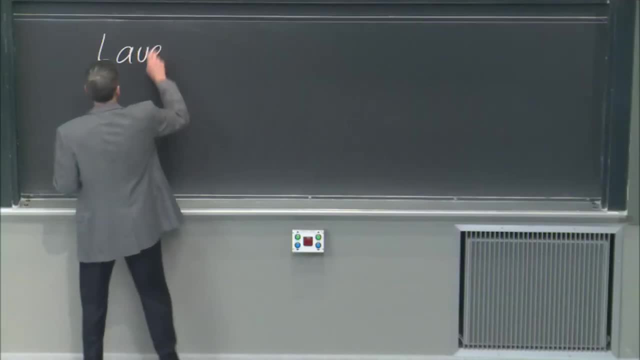 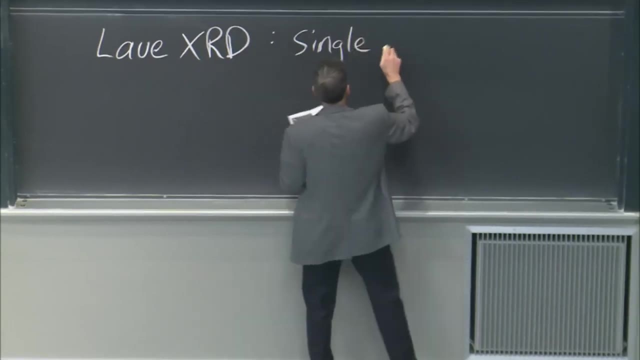 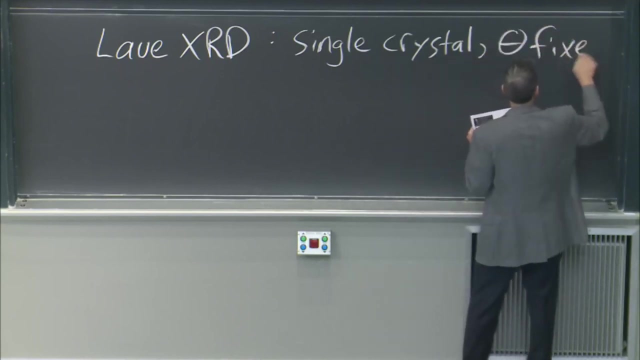 So in Laue XRD? in Laue XRD, you have a single crystal. It's got to be the same everywhere. in this case You have a single crystal. Theta is fixed right, You don't move it around. but lambda varies. 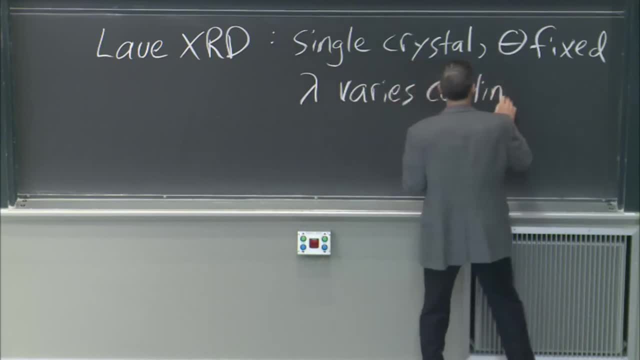 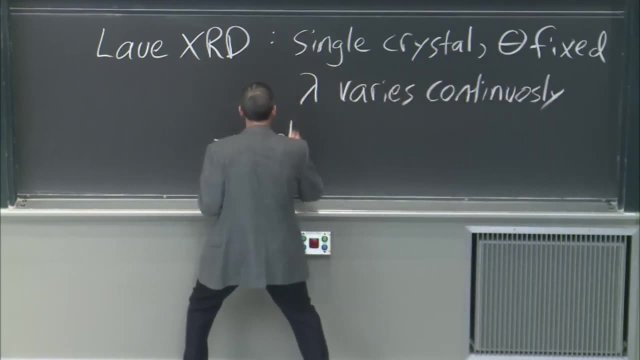 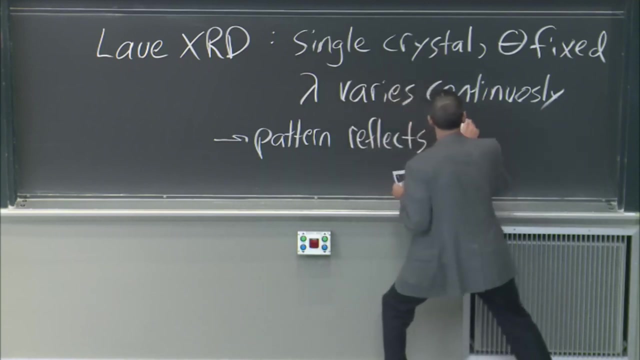 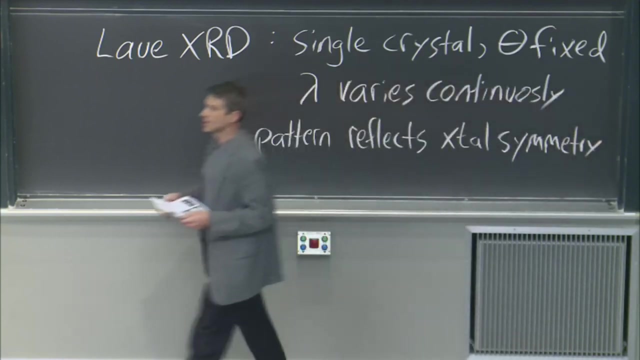 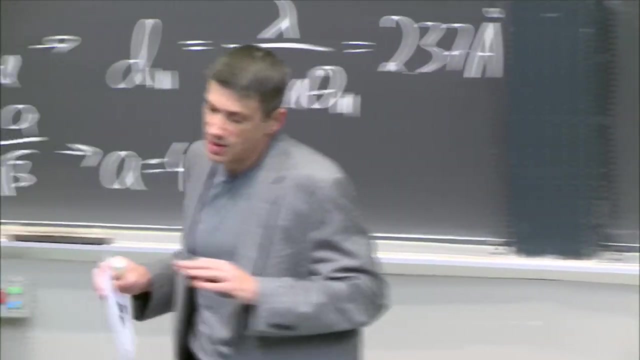 Continuously Okay, And the pattern that you get reflects the symmetry Pattern, reflects the crystal symmetry. How is that possible? Well, you can actually see this by thinking about the. do? I have another picture, His one. You can see this by thinking about that model. 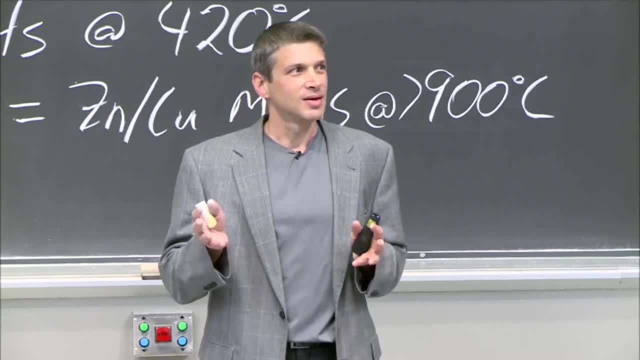 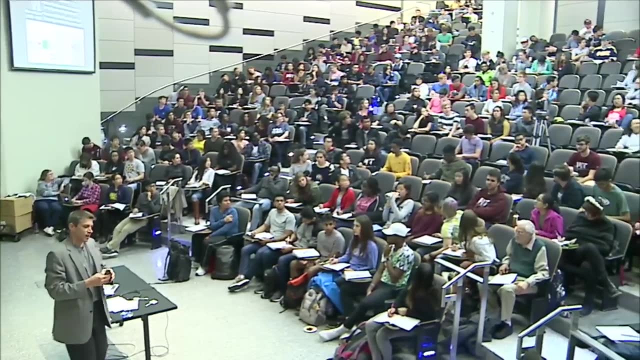 which is somewhere out there in the sea. Where is the model? I don't see it All the way in the back waving around. If I, let's see if I can draw this, Let's see If I shoot. I'm not going to try. 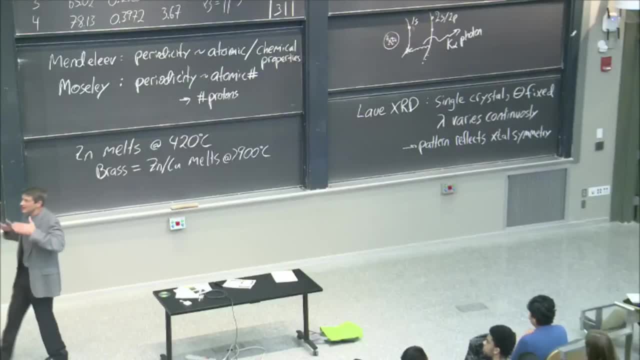 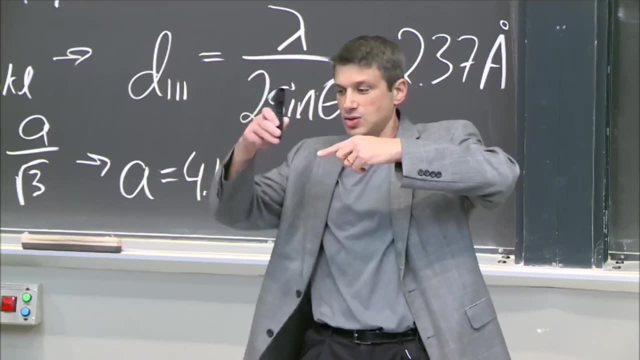 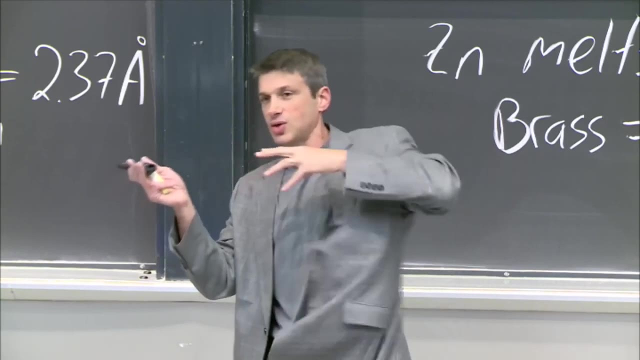 If I shoot x-rays that have a fixed lambda in but I vary the angle, then, as we've been talking about, there's going to be certain angles where you get constructive interference. Now, if I keep the thing fixed and I shoot all lambdas into it, 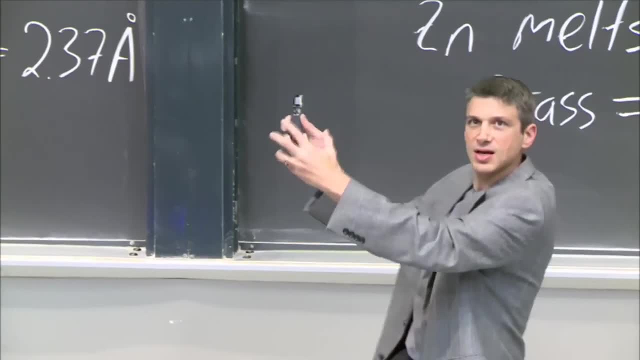 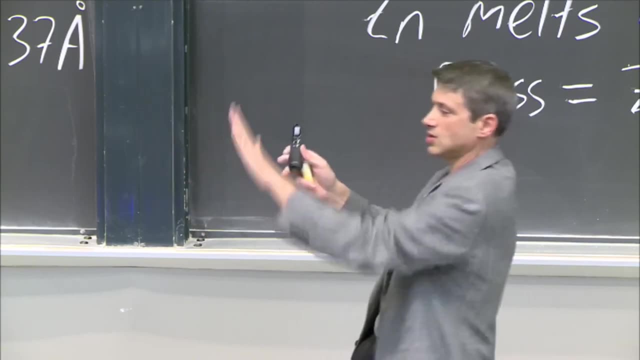 well, take a look at the crystal. Imagine that I'm holding that structure right now. Okay, Well, I'm going to see this set of planes here. So I'm going to see this set of planes. Maybe they're the 100 planes. 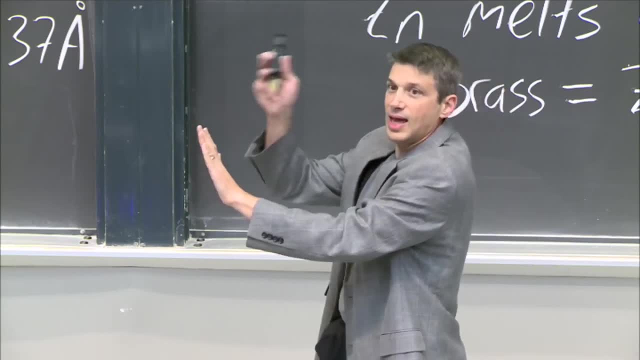 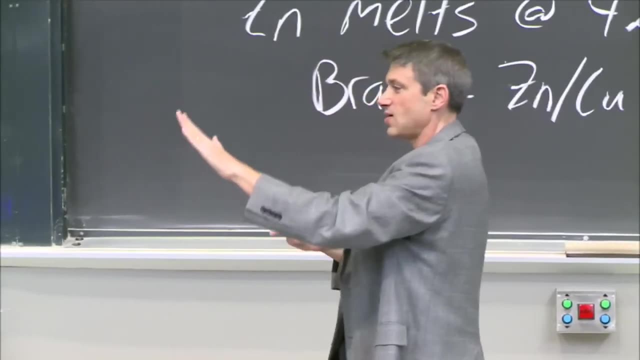 I don't know All right And I'm going to bounce off of that and constructively interfere, maybe if I've got the right lambda. But see, if I'm looking at the crystal and it's fixed, I'm going to see also there's another set of planes like that. 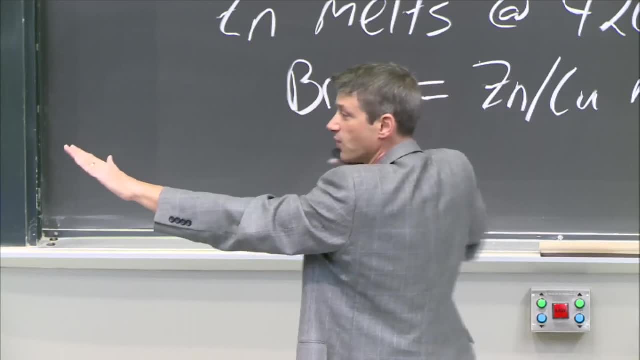 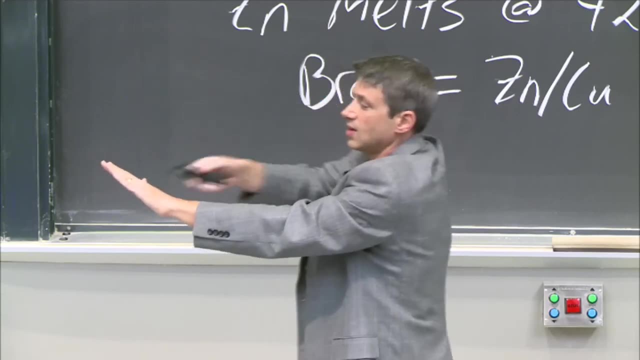 You see, There's another set of planes like that And if I'm a different wavelength- not the same one, but a different one- I might constructively interfere with those. But you can see that the angle that I make would be different. 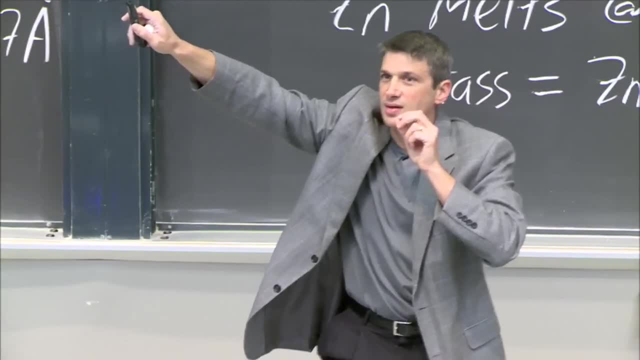 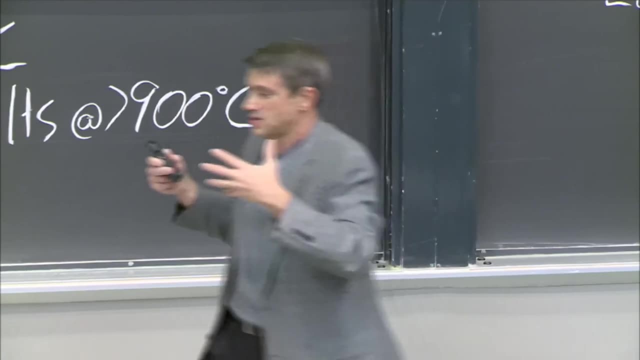 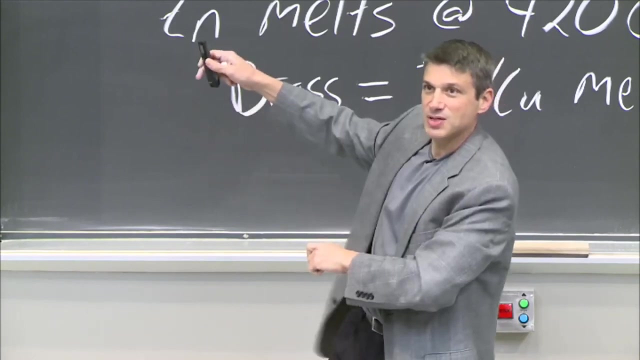 And so I'll put a spot in a different place, You see, So I've got all the wavelengths there, And as they constructively interfere with different planes that they see, they make different spots, They make different spots, And that's what those are. 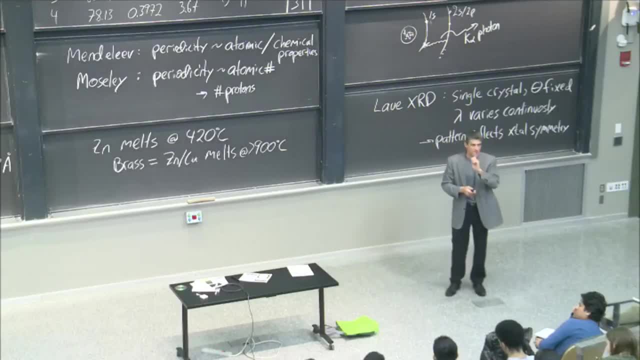 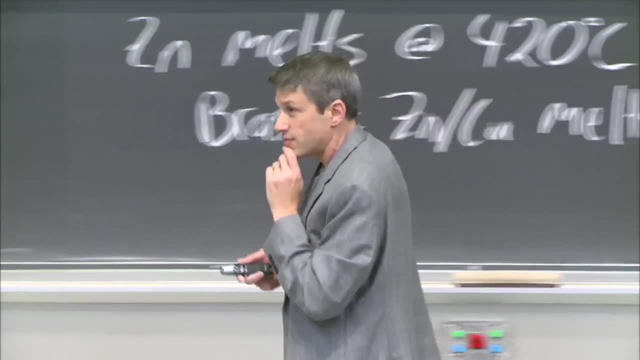 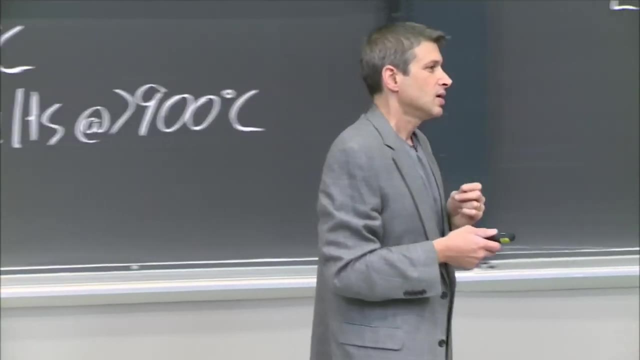 In those spots it's more complicated. to get crystal structure from those spots It's more complicated. You can get symmetry fairly easily, But getting the structure itself is a little bit more complicated. It can be tricky And for that and other reasons 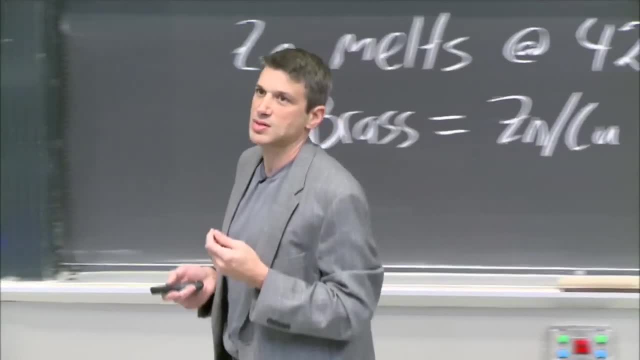 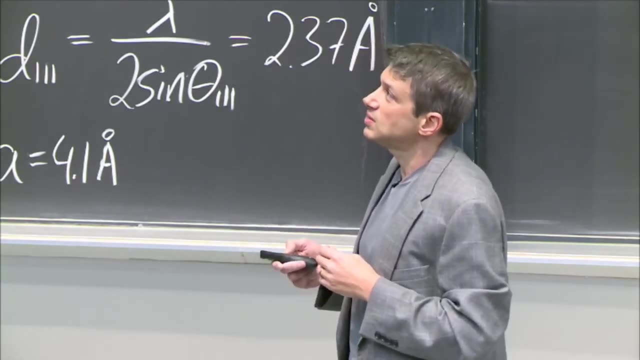 most work today is done with characteristic peaks, XRD, But this happened before And so I wanted to show it to you. And this resolved- actually in one of Laue's very famous papers it resolved- the structure of zinc sulfide. 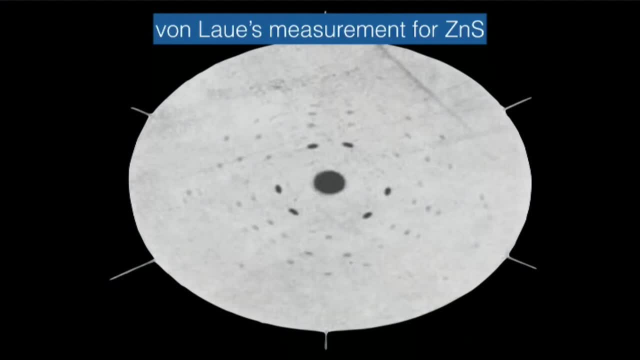 It was very important work. And those are the spots. Look at that pattern there. See, the thing that you could get is the symmetry, Oh, by the way. by the way, we will only test. I'm not going to test you on Laue. 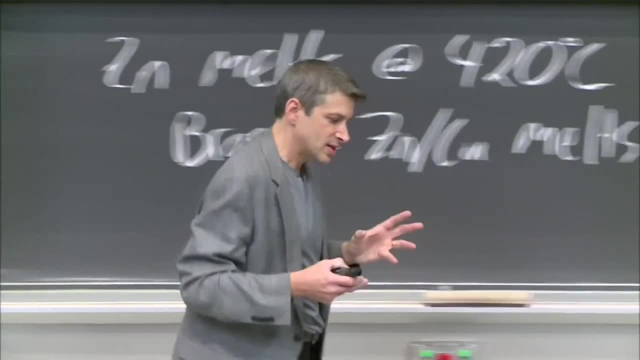 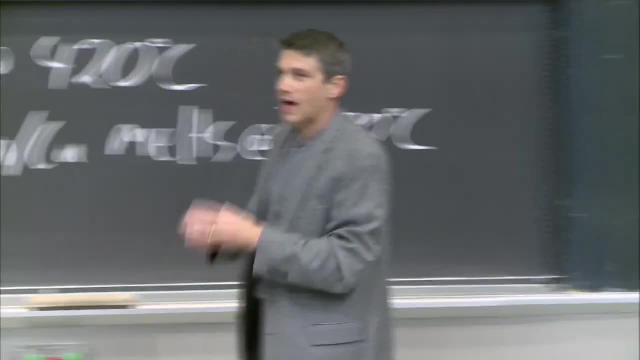 I'm only talking about it for five minutes here, Right? So in this class, I want you to know about using characteristic peaks and all the things we've been talking about. Laue is just on the side for knowledge. We won't test on this. 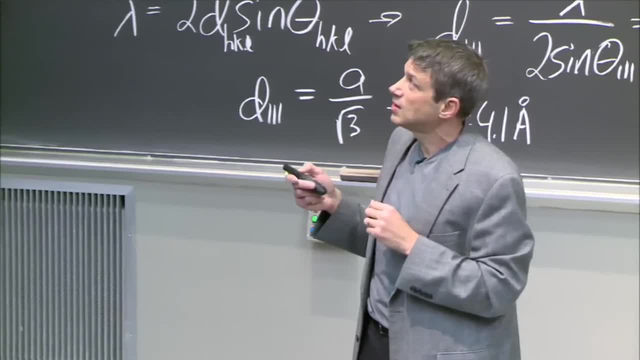 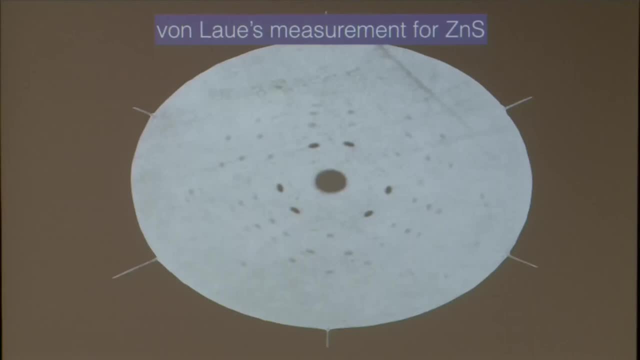 But I want to end by telling you a story. This tells you something about crystal symmetry. What is symmetry? Well, it just means: if I rotate it, is it the same? Or if I translate it, is it the same. Give me just one minute. 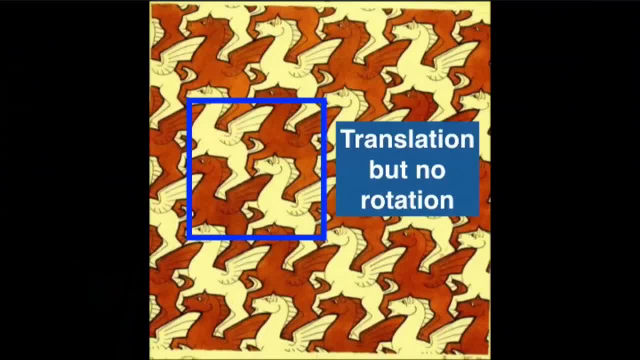 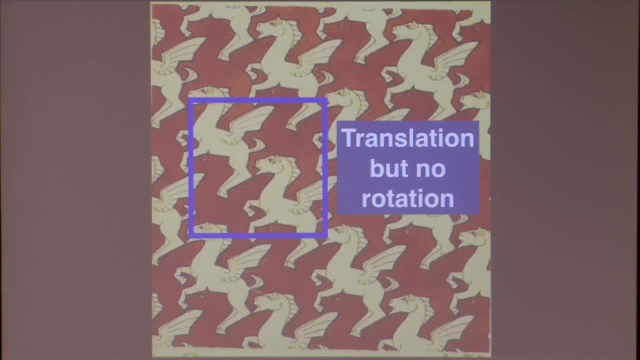 Because this is actually a really interesting story. That's translational symmetry. We looked at this picture already. There's no rotational symmetry. To get back to this picture, I'd have to rotate the whole thing by 360 degrees. But see, there are crystals that actually have.